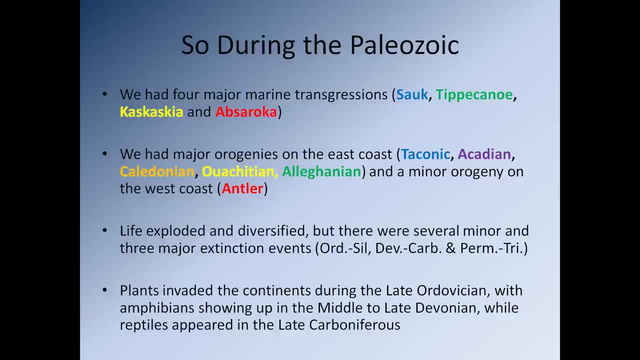 are termed the Sok, the Tippecanoe, the Kaskaskia and the Absaroka, And each of them result. each of them produced an Epiric sea that either partially or completely covered the United States and the vast majority of what is now North America. So we're going to be talking about the Mesozoic. 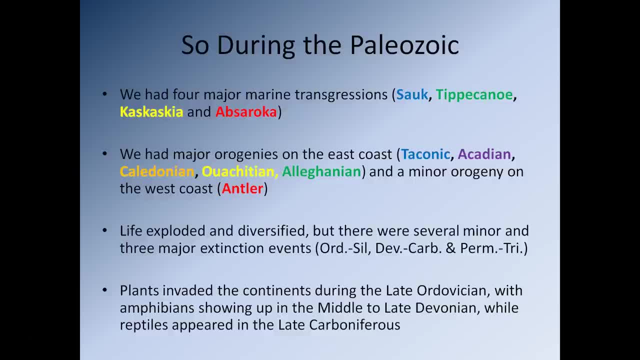 and the Epiric seas, So we're going to be talking about the Mesozoic and the Absaroka, And we also had orogenies on the east coast, So we had the Taconic Orogeny, the Acadian Orogeny, the Caledonian Orogeny. 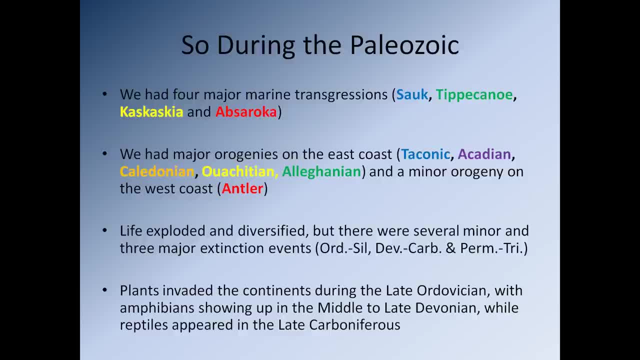 the Achetan Orogeny and the Elikahenian Orogeny, That's on the east coast, And we had a minor orogeny on the west coast which was called the Antler Orogeny. We also see that life exploded. 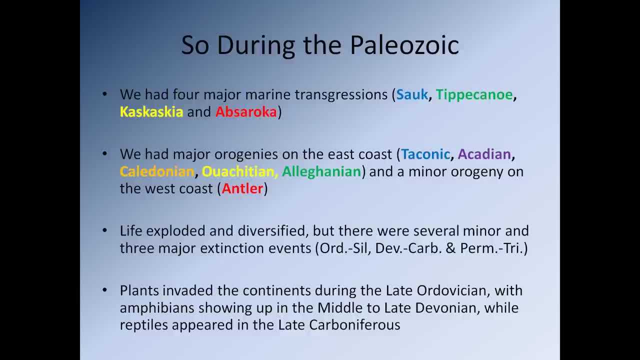 and diversified, But there were several minor and major extinction events during the Paleozoic as well. So during the Paleozoic we had the Ordovician Orogeny And we also had the Antler Orogeny And we also had the Antler Orogeny And we also had the Antler Orogeny And we also have plants invading. 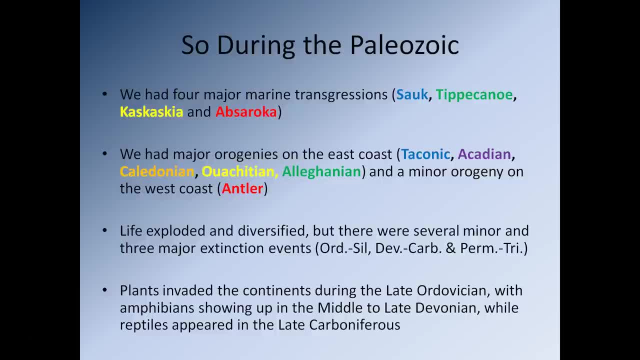 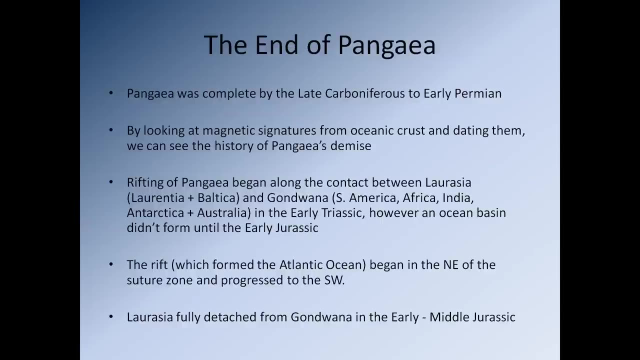 the continents from the late Ordovician onwards. We have amphibians showing up in the middle to late Devonian And we have reptiles appearing in the late Carboniferous. So it was all go pretty much for the world during the Paleozoic, especially towards the end. So the transition 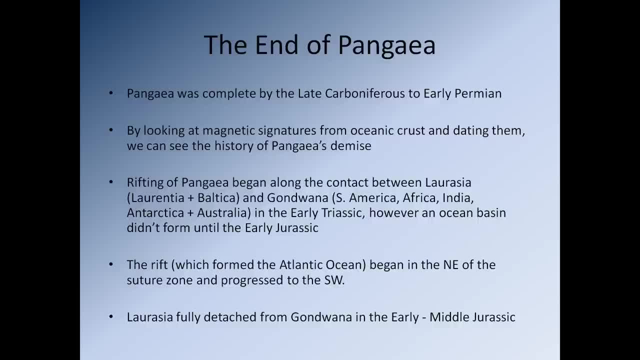 from the Permian into the Triassic is a very important part of the Paleozoic And it's a very important part of the Paleozoic, And it's a very important part of the Paleozoic, And it's marked by two things. The first thing is that we see a lot of organisms disappearing that were 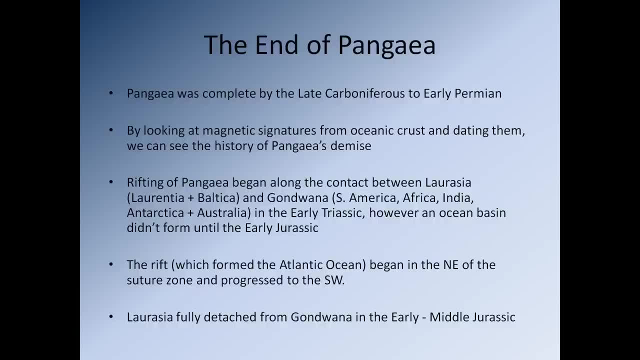 present in the Permian. So, of course, if you remember the Permian-Triassic, mass extinction occurs and it kills off a lot of organisms. And so, to start with, when we look at the rock record, we see the loss of a significant proportion of these organisms. So that tells us that we've 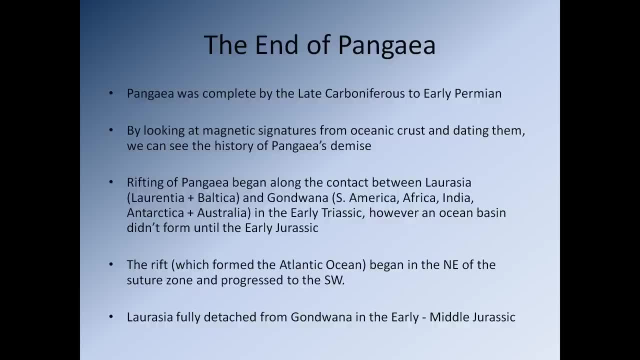 crossed the boundary from the Permian into the Triassic. The other thing that begins to show us that we've moved from the Permian into the Triassic is that we've moved from the Permian into the Triassic is we begin to see the first indications of the breakup of Pangaea. So if you remember, 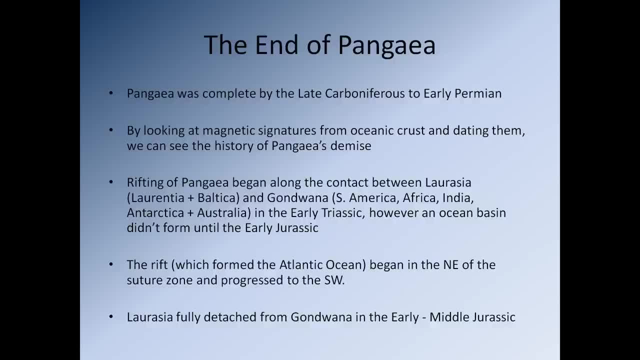 Pangaea formed when Gondwana made contact with Laurasia during the late Carboniferous to early Permian And by the end of the Permian into the Triassic. that supercontinent is now falling to pieces. So by looking at the magnetic signatures from oceanic crust and also dating the oceanic 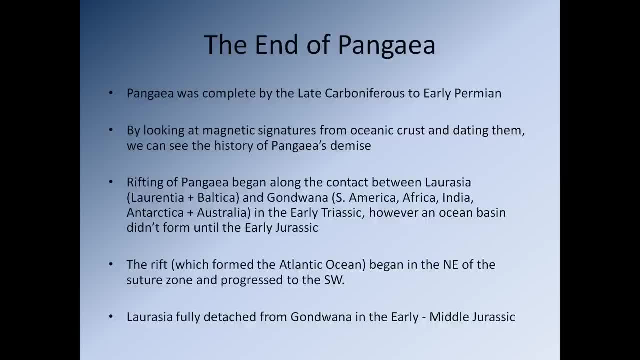 crust. we can see the history of Pangaea's demise, Because, obviously, when a two piece of continent move away from each other, well, the space in between them gets filled by an ocean basin, And so we can actually see the start of, you know the date on which that ocean basin starts forming. We 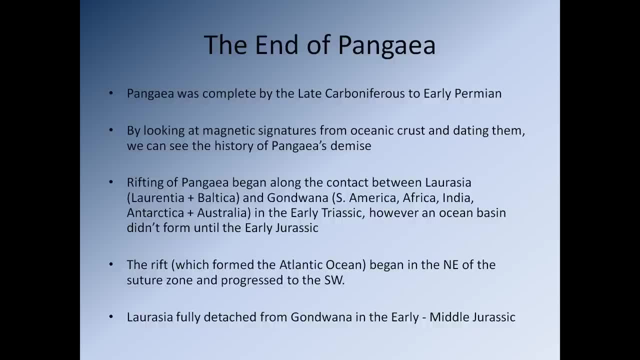 can find the oldest oceanic crust, we can date it and we can say: right, this is when the oceanic crust started forming. So we know when these basins began to be produced. So we know that rifting of Pangaea's energy began along the contact between Laurasia, so that's Laurentia, post Baltica, and Gondwana. so 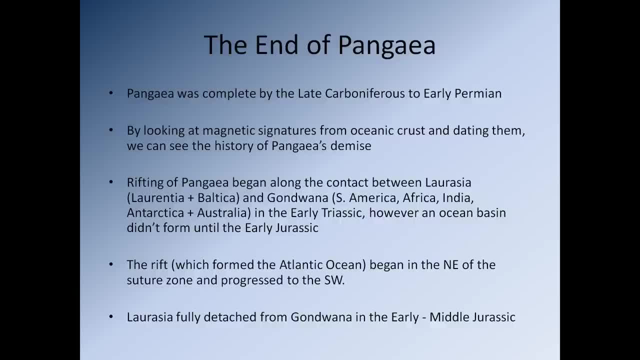 Gondwana is South America, Africa, India, Antarctica and Australia, And we know it began in the mid Triassic. however, we didn't actually see an ocean basin forming between those two supercontinents until the early Jurassic, so it took a while for an ocean basin to actually form. So the rift that 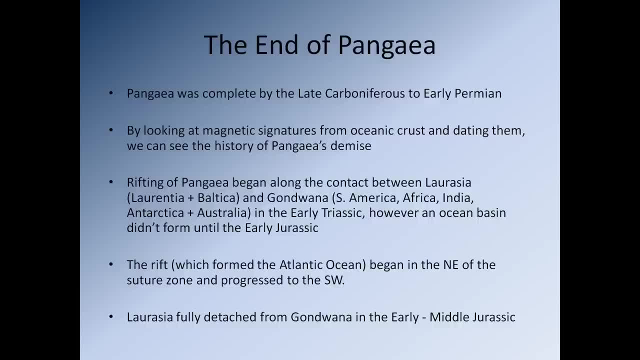 would eventually go to form. the Atlantic Ocean began in the northeast of the Suture Zone between Gondwana and Laresia, again the northeast of the suture zone between Gondwana and Laresia, and it progressed in a southwesterly direction. So we see that Laresia and Gondwana have fully 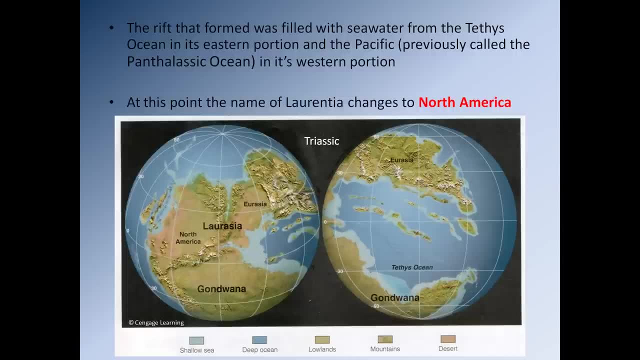 detached themselves from each other by the early to middle Jurassic. So this is our situation. So obviously, towards the end of the Carboniferous to early Permian we had the formation of Pangaea, So we had Gondwana come slamming into Laresia and that formed essentially a range of mountains. 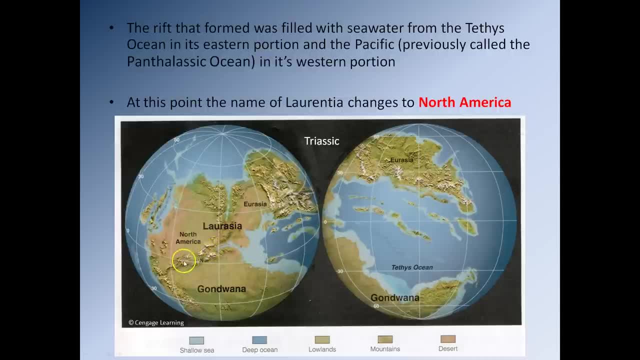 that goes from what is now southern Europe down the eastern seaboard of the United States and into what is now the Gulf Coast region, So that separates Laresia from Gondwana, and at the same time over here we had Siberia crashing into Baltica to produce the Ural Mountains here. 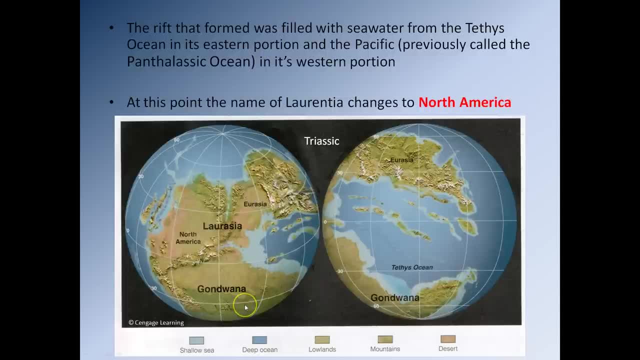 And obviously that produced the supercontinent Pangaea. So what we're going to see is we're going to see that rifting begins to occur along this suture zone here between Gondwana and Laresia, And the rift itself starts up here in the northeastern corner. 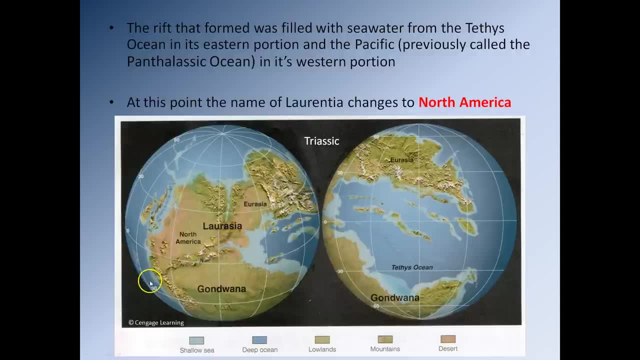 and it progresses in this direction towards the southwest. So, okay, so, in terms of the, the body of water that's surrounding Pangaea, okay, it was referred to, as it was initially referred to earlier, as the panthelassic ocean. However, by the time we make it into the Meser, it's now referred to as 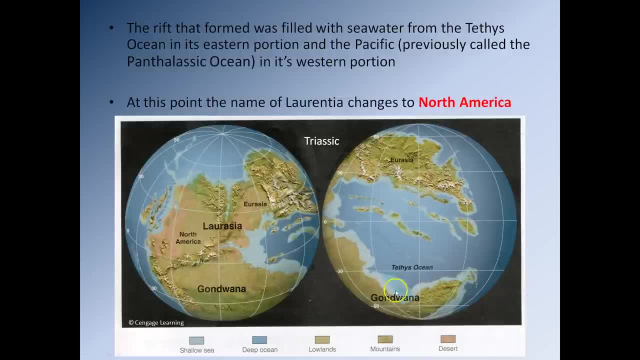 the Pacific, And we also have a very important body of water over here. This is called the Teffis Ocean. So the Teffis Ocean is very important because it is situated over the equator. It's a relatively restricted body of water, And so what we're going to end up with here is a nice 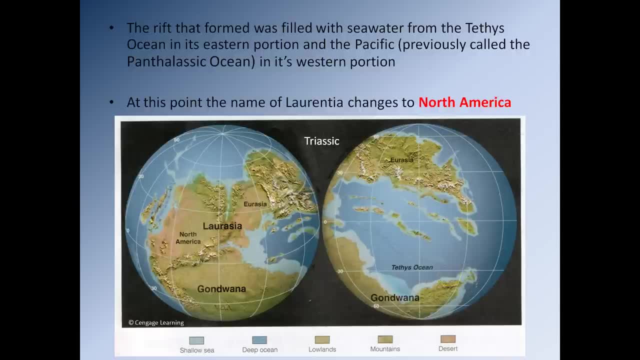 warm body of water, a little bit like the modern Indian Ocean, And so this is going to have a very interesting repercussions for water circulation later on in the Meserzoic. So this is the point, by the way, at which we no longer have Laurentia, We're no longer talking. 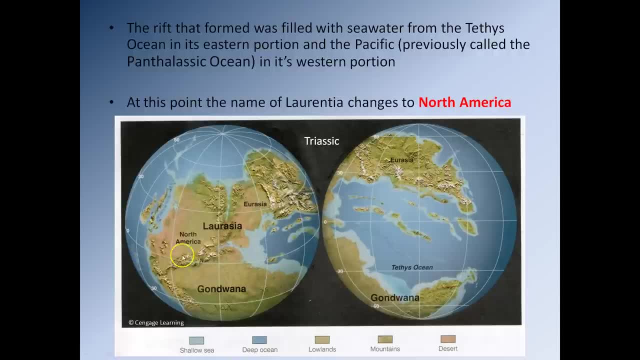 about Laurentia. We now discuss this piece of crust and we refer to it as North America. So North America essentially consists of Greenland's going to be about here, Canada's going to be about here, The United States is going to be about here And pieces of Northern Mexico are going to be. 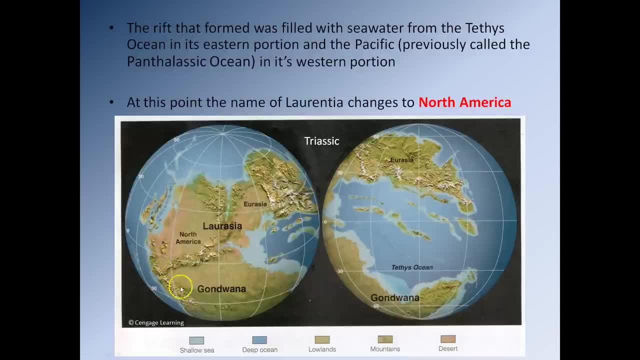 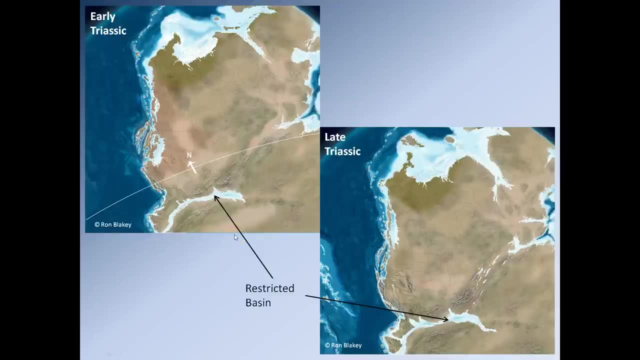 somewhere around here. Okay, So we now have what we would classify as North America. So all right. So this is our situation in the early Triassic. So, as we can quite clearly see, we have La Raya here, Gondwana. 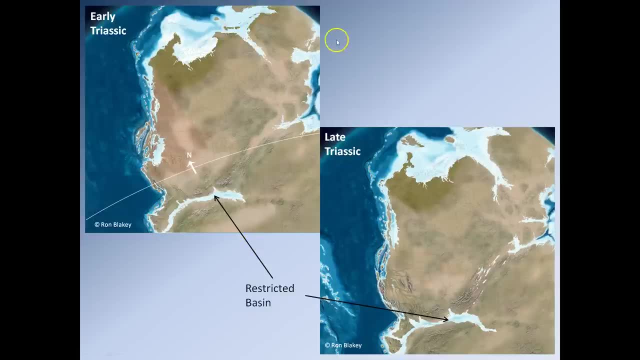 down here and we have the Sucha Zone here. We have the Hessinian Mountains in Southern Europe. used to be there. They've been completely eroded away, They're gone. The Achiton Mountains over here in the Gulf States. So here's Texas down here. They're pretty much gone as well, And we 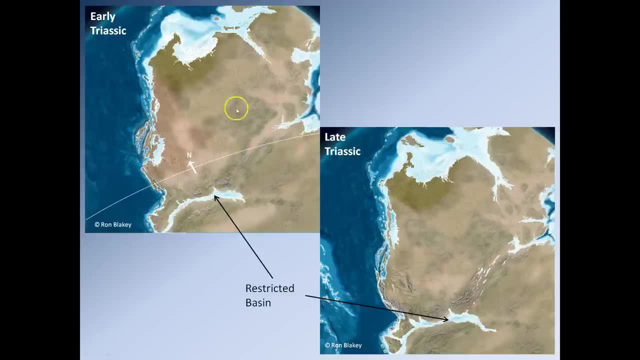 have the Mobile Belt right here. You can just see it in this area. here We have a bit of the Appalachians left, but they also have been significantly eroded down. So this is the situation in the early Triassic. We also have the formation of a restricted body of water down here in the 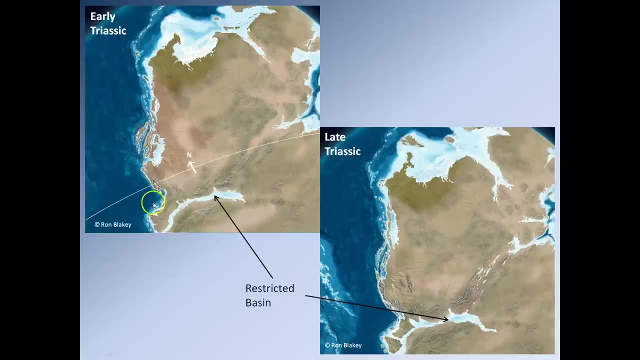 southwest of portion of the Sucha Zone. That's nothing to do with rifting. That's just some water that's gotten trapped in this area and is slowly evaporating away. So as we move into the late Triassic we begin to see rifting develop along this Sucha Zone. 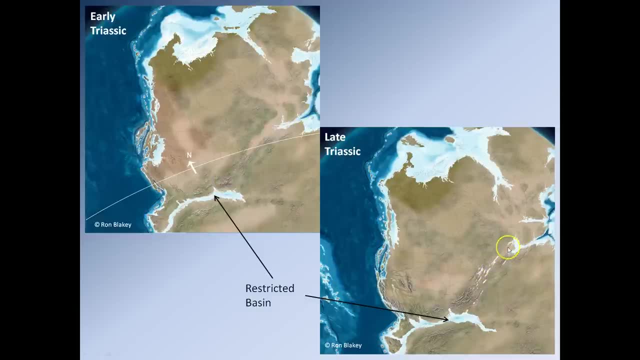 And we can see it developing, because we begin to form lots and lots of big, long, normal faults, all running parallel to each other in an approximately northeast, southwest direction. And so this is telling us, the crust is beginning to undergo extension, It's beginning to be stretched. So, initially, when you take a piece of rock and you begin to 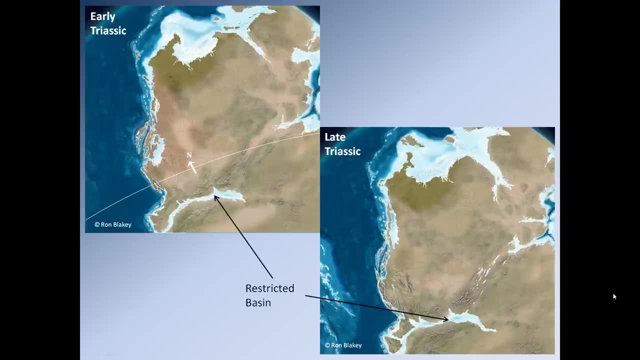 stretch it for a short period of time, that rock will behave like a liquid or behave a bit like silly putty. It will begin, you can stretch it and as you stretch it begins to become thinner. But you can't do that for very, very long with rock. So once you reach 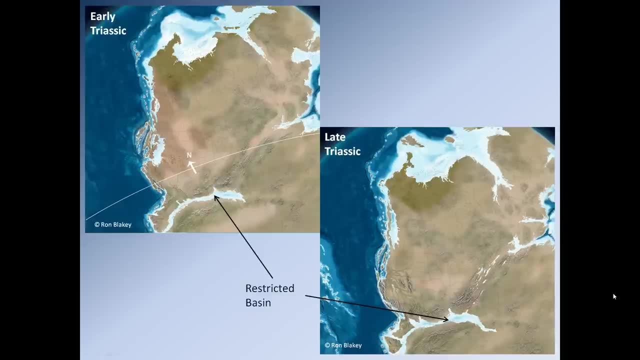 a certain point the rock can't really stretch any further and it begins to break. So instead of flowing like a liquid, it starts to break and fail like a solid. So when it begins to break and fail, that means essentially you begin to form blocks of rock. and as you pull those blocks of rock, those 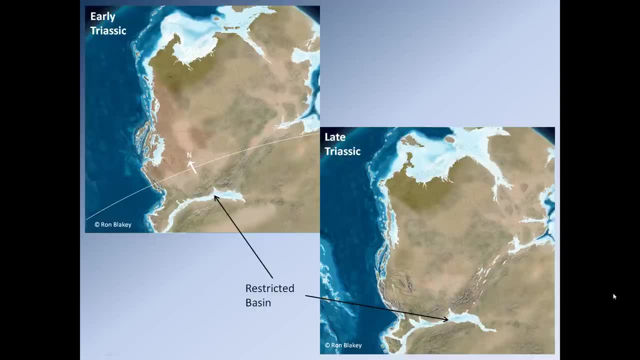 blocks of rock will drop down relative to one another. And as those blocks of rock drop down, well, they're going to form a topographic low which we refer to as a rift valley, And one of the indicators that we have a rift valley is it will be a linear body. So you can see it here. this: 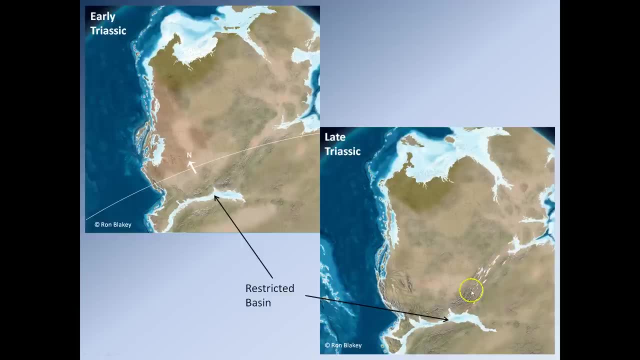 is our linear rift valley here, And we can see it has lots and lots of long normal faults that are all orientated parallel to each other. They are also orientated parallel with the elongation direction of the rift valley And so that's showing us we have all these blocks of rock. 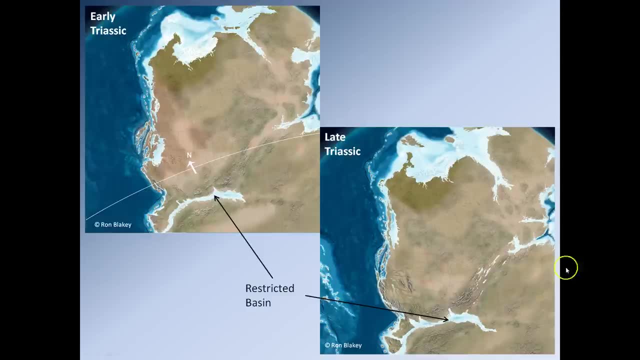 all dropping down relative to each other, because this area of crust right here is being stretched, And it's being stretched because La Raya is trying to go this way and Gondwana is trying to go this way, And so this area of rock in between is undergoing extension. 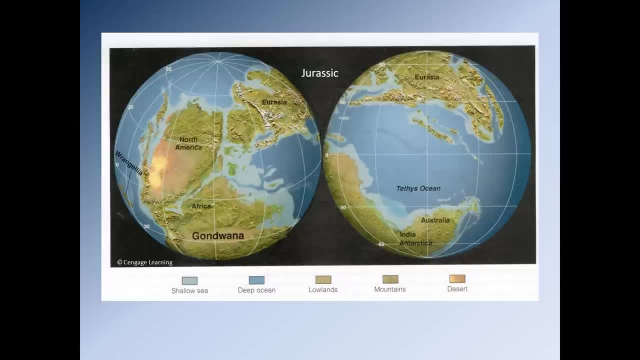 Okay, so by the time we're into the Jurassic, what's going on? Well, the rift zone here between Gondwana and between North America has begun to become quite extensive and we have the rift zone filling with water. So we have the start of what will become the rift valley And we have the 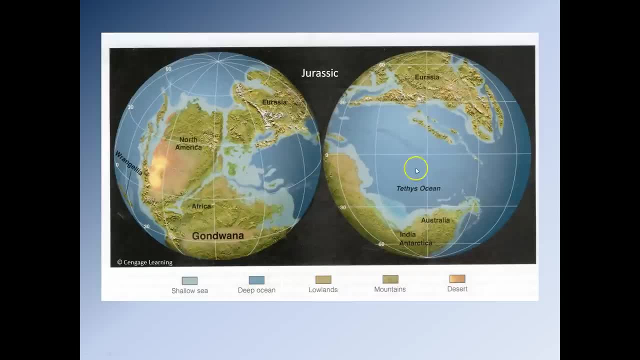 rift zone filling between Asia and South Network. So Gondwana and shortcut can be duplicated and this will become the modern North Atlantic. We can also see still in the Jurassic we still have the Tephys Ocean. here Gondwana is still in one piece: Africa, South. 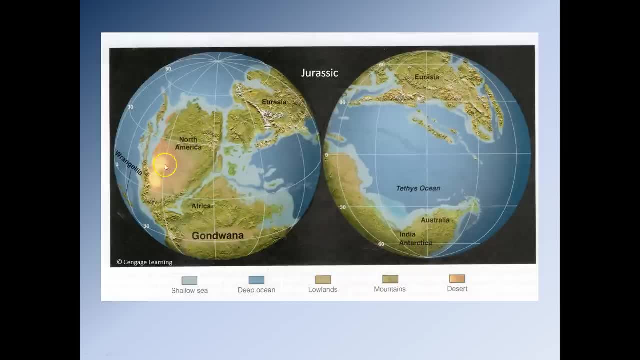 America, Australia, India and Antarctica. they're all still together. North America is still in one piece. We still have Greenland, Canada, North America, a little bit of Mexico down here And, although it doesn't look like it because we had this line of water here, North America is still. 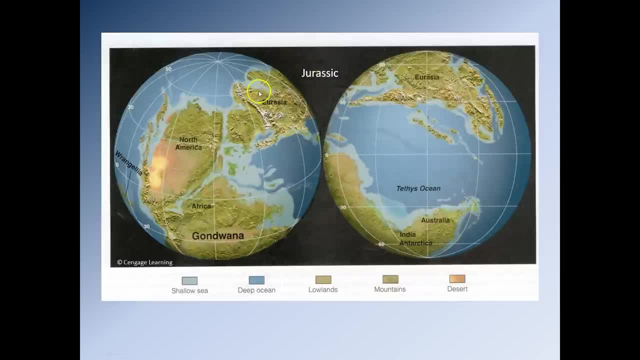 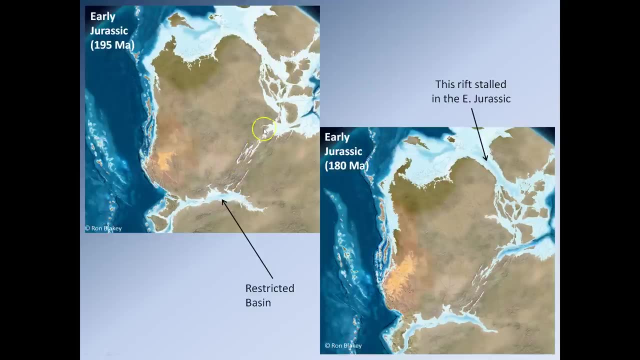 which we are still referring to as Laurasia or Eurasia, depending on you know what you want to call it. Okay, so as we move into the Jurassic, we begin to see this rift valley starts to fill with water. Now, this is still a restricted basin down here. okay, The water itself is coming from. 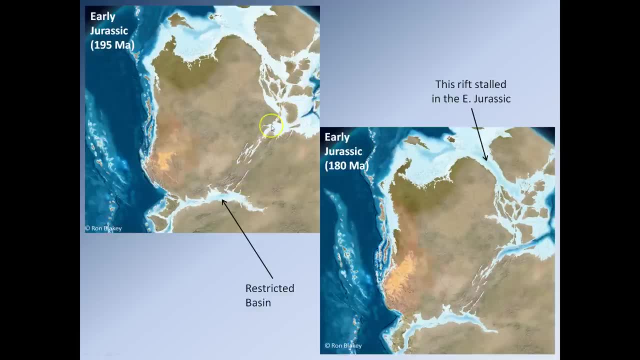 the northeast and is going to start filling the basin from towards the southwest. So by the time we make it into the early Jurassic, we can see we have this deep line coming here. okay, This is the formation of the ocean crust proper. okay, So all of this rifting here has just been continental. 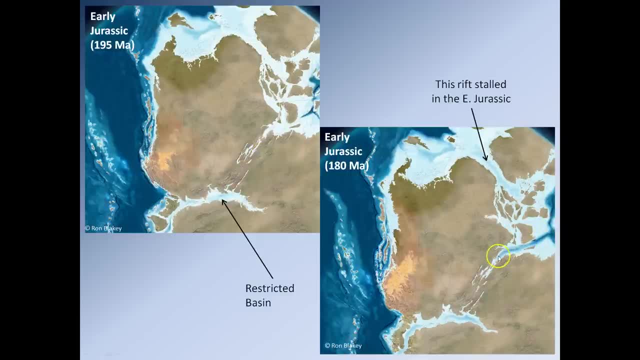 crust. It's at this point we start seeing the formation. well, the melting of the mantle underneath the rift, That melting mantle produces basaltic magma, mafic magma that rises through the crust, pushes the crust apart and creates oceanic crust. So at this point we actually have 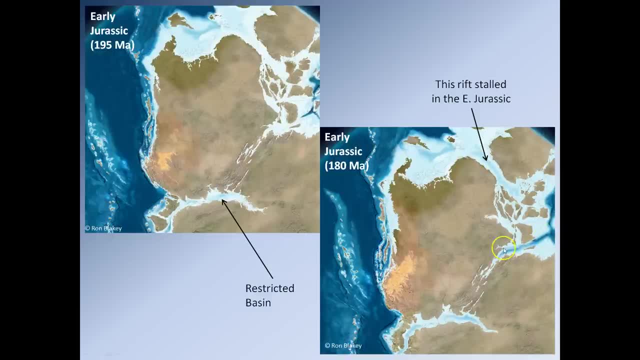 the starfish. This is part of the formation of the North Atlantic taking place. okay, So we also have the early stages of some rifting up here between Greenland and Scandinavia. Now this isn't actually going to develop very much, but it is the very, very early stages of the rifting that will eventually lead to 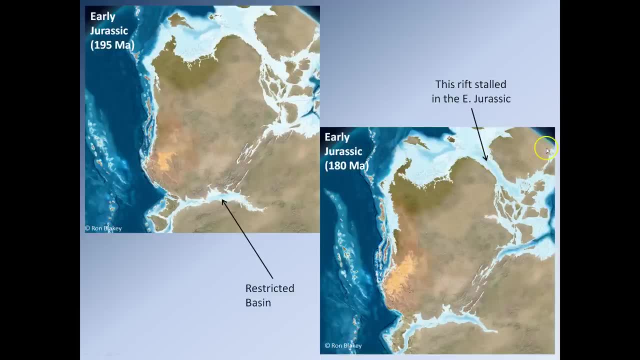 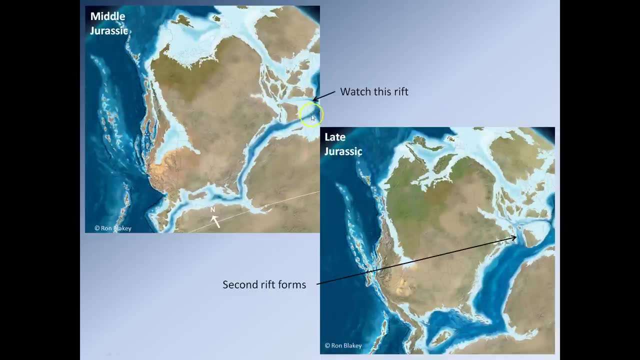 the separation of North America and Eurasia. Okay, so, as we're going through the Jurassic anyway, this rift valley is becoming more and more pronounced By the time we're into the middle Jurassic. you can see, we're going to be in the middle of the North Atlantic and we're going to 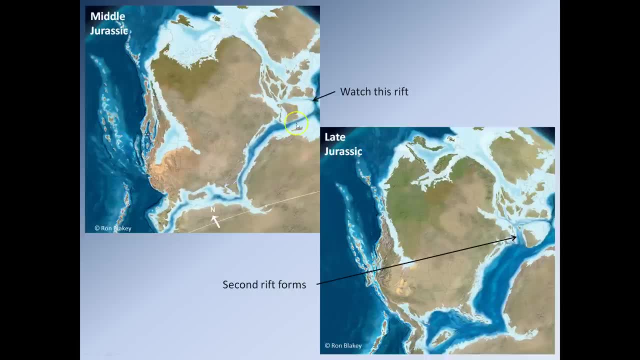 have a solid line of dark blue here going all the way from the Atlantic all the way into now what is the modern-day Gulf region? And so this is all new oceanic crust forming, so we now have a proper oceanic basin forming. So at this point we have a rift that's running down the middle, creating new. 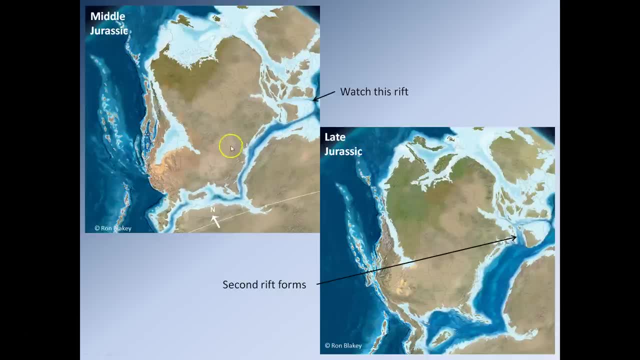 oceanic crust that's going to push North America this way up towards the northwest and it's going to push Gondwana this way down towards the southeast. And as we keep going into the late Jurassic, we can see that the formation of the oceanic crust has 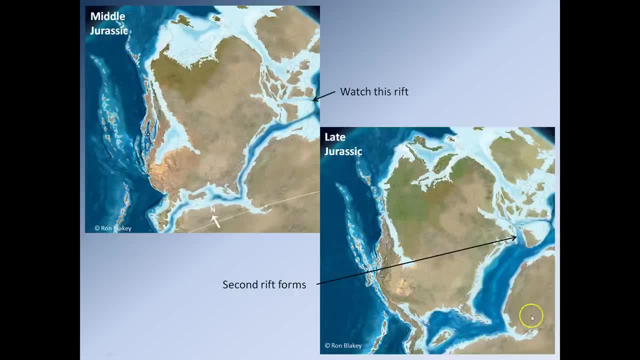 continued to push North America to the northwest, Gondwana to the southeast, and the ocean basin steadily getting larger. We can also see that if you look here, here's Spain, or modern-day Spain, and you can see there's no rift here yet, But by the time we're into the late Jurassic, you can see. 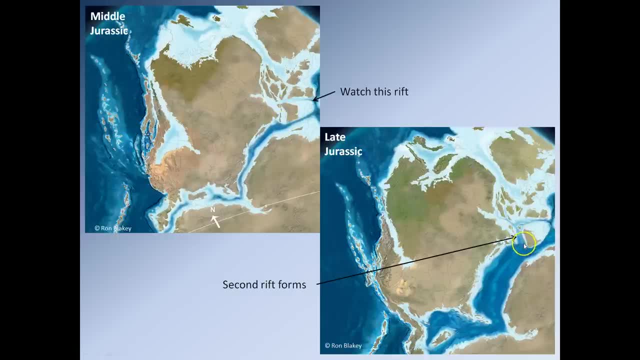 a rift has started to develop here between essentially along what is the west coast of Spain and Portugal, And it's coming down the middle of the Atlantic and it's going to push North America to the southeast and it's coming up here. Here's the United Kingdom and Ireland right there, and you. 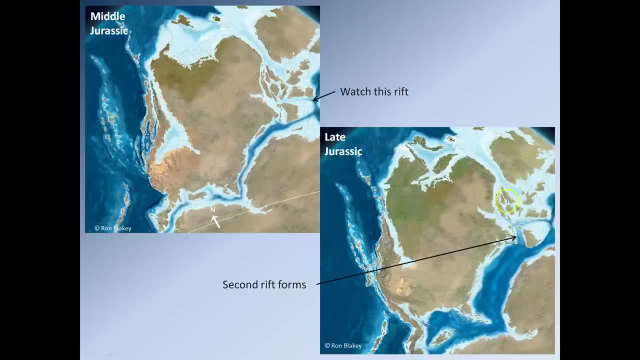 can see, this rift is starting to develop up here between the United Kingdom and Ireland and Greenland, right here. Okay, now once again, this rift still isn't particularly well-developed. so make it clear: North America and Europe are still attached to each other at this point. There's still one landmass. 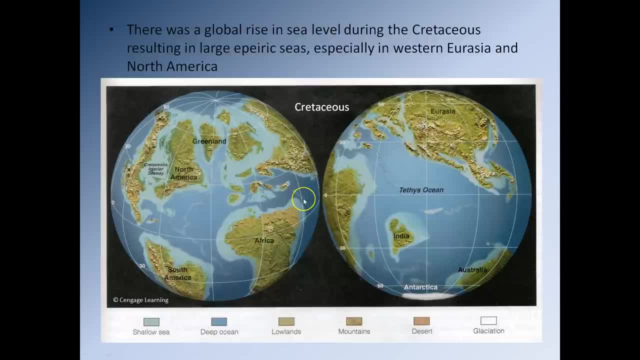 Okay, so by the time we make it into the Cretaceous, what's going on now? Well, the Cretaceous is marked by a period of very, very high sea levels, So the global sea level is about 250 meters higher than present-day. 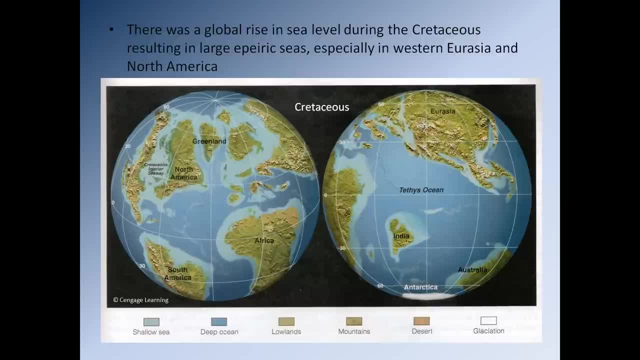 And so this leads to very, very widespread global empiric sea. So we have a global marine transgression going on. So you can see, Europe is nearly completely underwater. Large portions of coastal Africa are underwater. Northern South America especially is underwater. We have this. 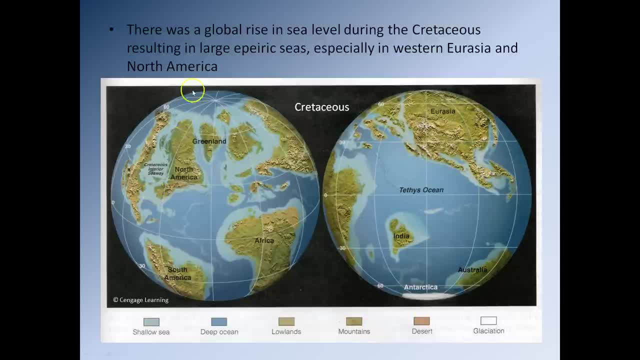 what's called the Cretaceous Interior Seaway, that bisects North America all the way from the Arctic Ocean up here, down to the Atlantic Ocean, And so this is a very, very high sea level, And so this is a very, very high sea level, And so we have this what's called the Cretaceous Interior Seaway. 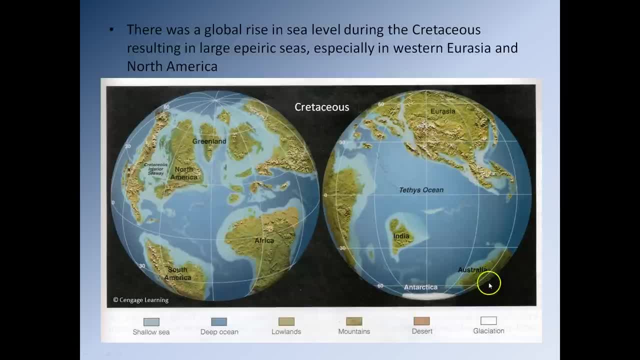 down to the Gulf of Mexico down here, And we can quite clearly see that portions of Asia are also underwater. Now we can also see by this point: South America, Africa, India, Australia and Antarctica have all separated from one another and they're all going off doing their own thing. 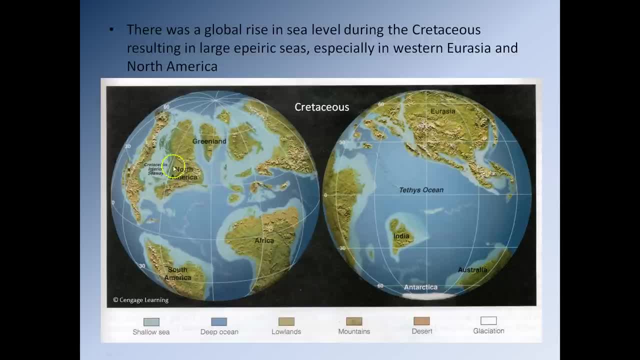 Now, although this diagram shows that North America and Europe look pretty much detached from each other, they are still attached to each other until right before the end of the Cretaceous. So we have this what's called the Cretaceous Interior Seaway that bisects North America all the way from. 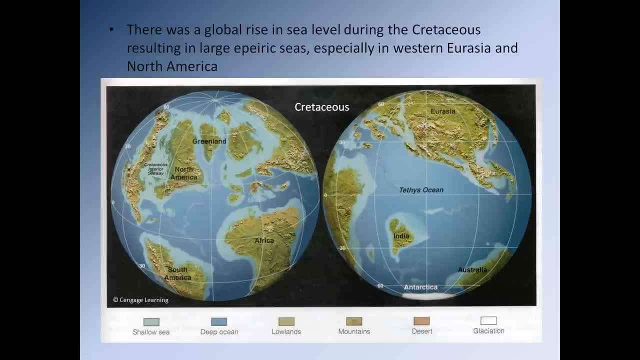 Right, literally the last minute of the Cretaceous. Okay, so, throughout the Cretaceous, North America, Europe, Asia, they're still moving together as one landmass. Okay, so, by the Cretaceous, what's going on? So in the early Cretaceous, the North Atlantic and 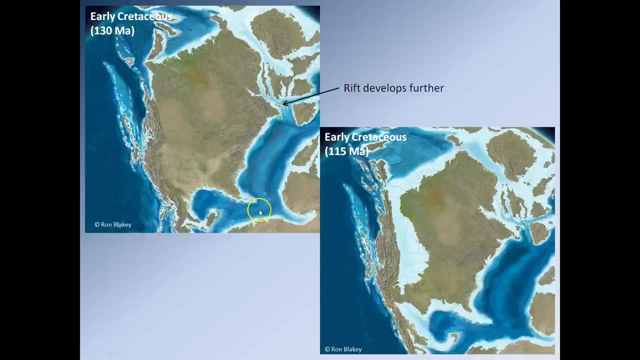 Gulf region is opening up nicely. We have lots of new oceanic crust forming once again, pushing North America off to the northwest, pushing Gondwana down here towards the southeast, And we can see that this rift that starts here, this rift that starts here, this rift that starts here, 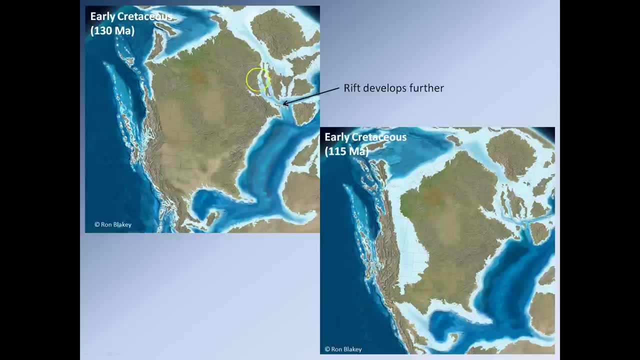 starting here has kind of stalled out a little bit. It's still there but it's not really growing very fast. You can see, by the time we're into the later portion of the early Cretaceous it's still there, not really developed very much. North America is still attached to Europe at this point. 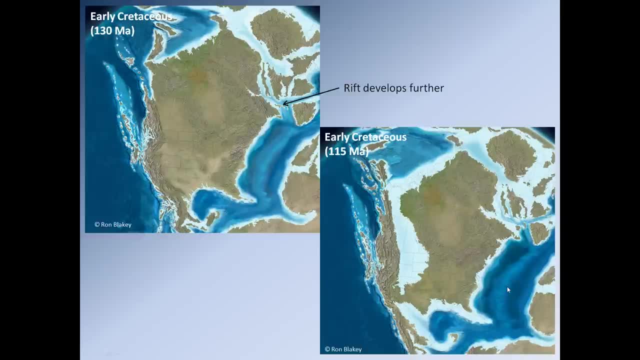 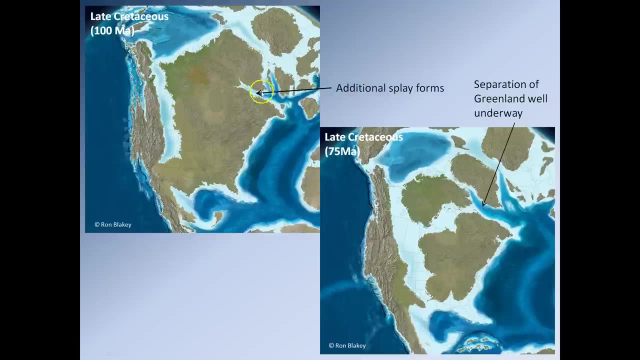 The North Atlantic and Gulf is still getting a little bit larger. It's steadily growing By the time we're into the late Cretaceous. you can see the North Atlantic's getting larger and you can see this rift has really started to develop now. Okay, we can see it's actually 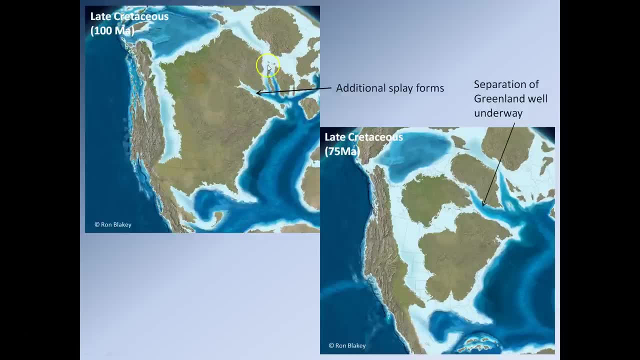 begun to split into two. One limb is coming out of the other and the other limb is coming out of the other. It's coming up here, so it's going to come up between the United Kingdom and Greenland and it's going to work its way up here between Greenland and Scandinavia. 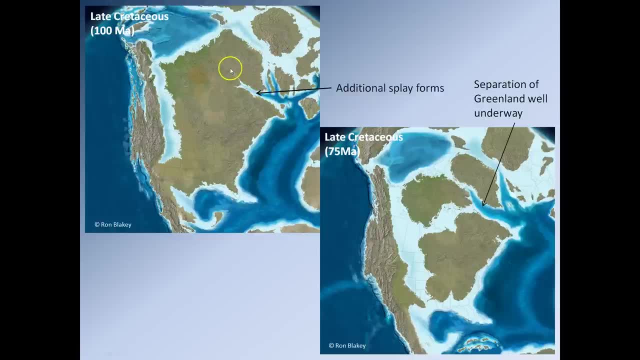 And another limb is going to come up here and that's going to separate Greenland from North America. By the time we're into the very late Cretaceous, we can see these rifts have developed very nicely. We can see that the United Kingdom is now well separated from Greenland by oceanic 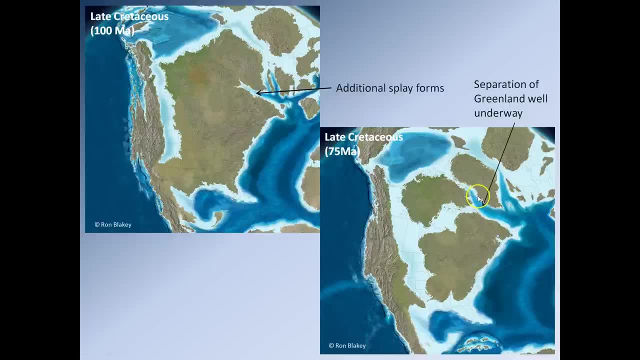 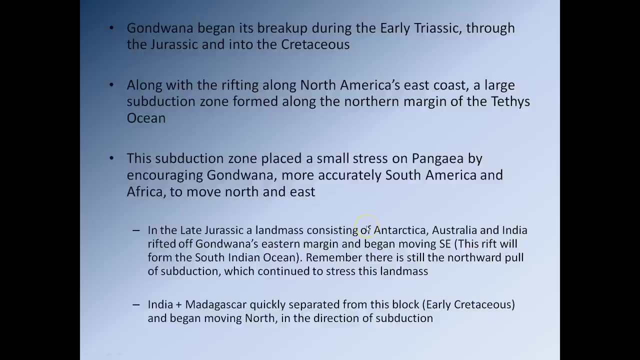 crust. We can see Greenland is beginning to separate from North America, but you can also see that they are still attached to each other, just holding on. So, in terms of the separation between North America and Europe, as I said, it really, really, really, the separation does not. 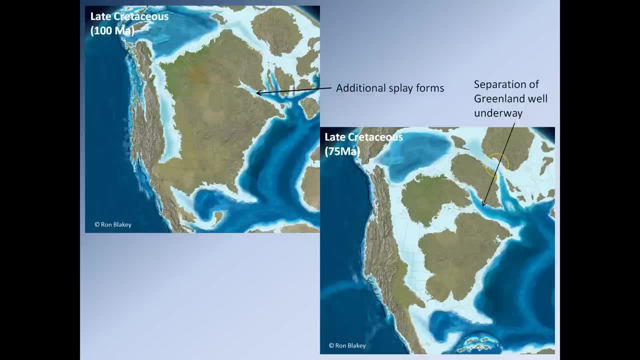 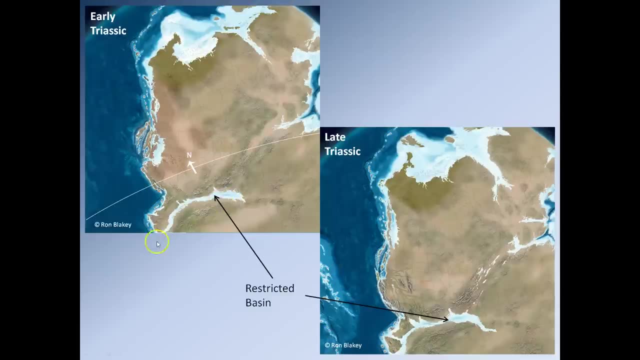 fully occur until right at the end of the Cretaceous. Another thing that you might have noticed is, as we've been moving through, so if we come, if we look here, this is the Triassic. This region down here is going to develop into Mexico. You can see that over time. you can see that 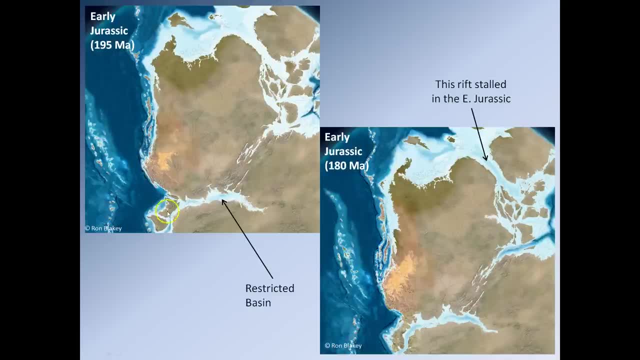 slowly but surely. we have several island arcs and we're going to see that we're going to have some of these island arcs appearing and attaching themselves into this region down here. So we have a subduction zone running down here, pulling oceanic crust this way, pulling material towards. 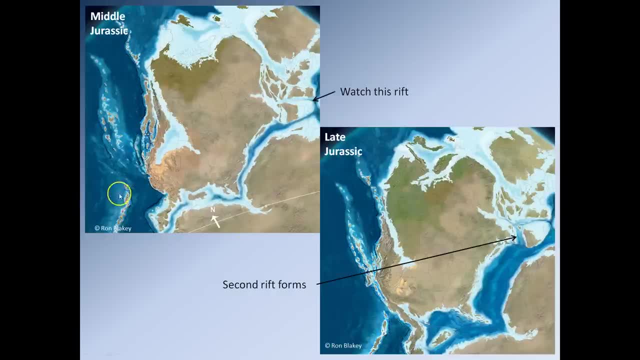 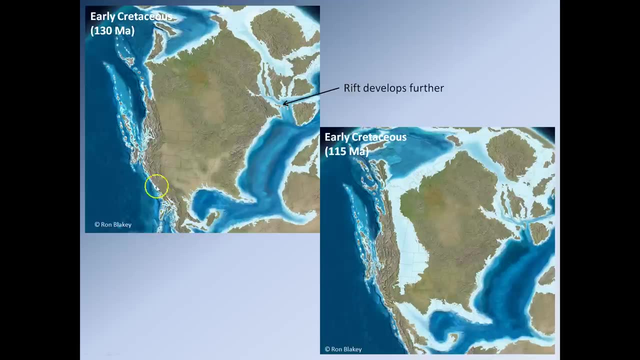 what is now modern-day Mexico. So you can see, you have several of these island arcs moving across and they're going to steadily collide with what is now modern-day Mexico and start to build up the mass of modern-day Mexico all the way through the Mesozoic. We can see Mexico is steadily getting. 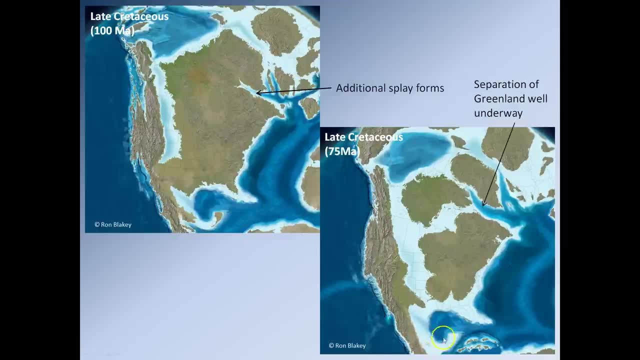 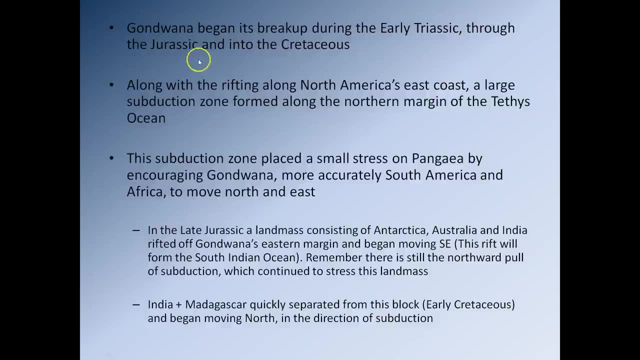 larger and as we move into the late Cretaceous we can see that, you know, modern-day Mexico is nearly fully formed at that point. So, in terms of Gondwana, it began its breakup during the early Triassic through the Jurassic and into the Cretaceous. 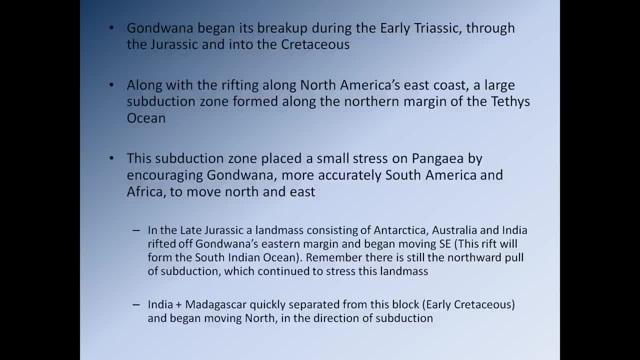 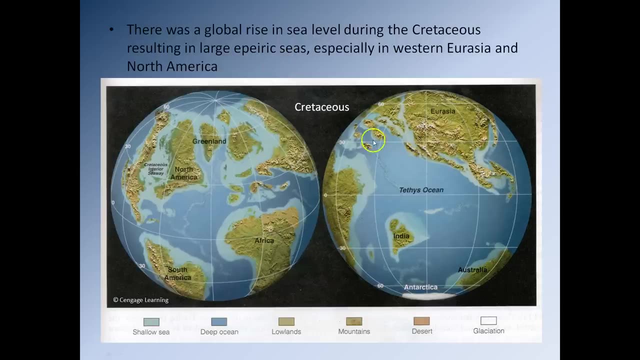 So remember, Gondwana is South America, Africa, India, Australia and Antarctica. So along with the rifting along North America's east coast, a large subduction zone formed along the northern margin of the Tethys Ocean. So here we go. So if we go back here, we have a subduction zone that's running all the way. 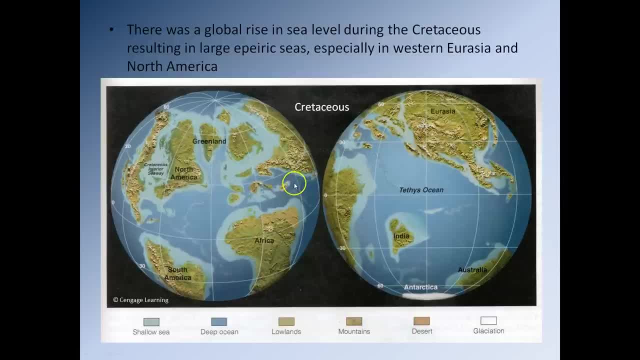 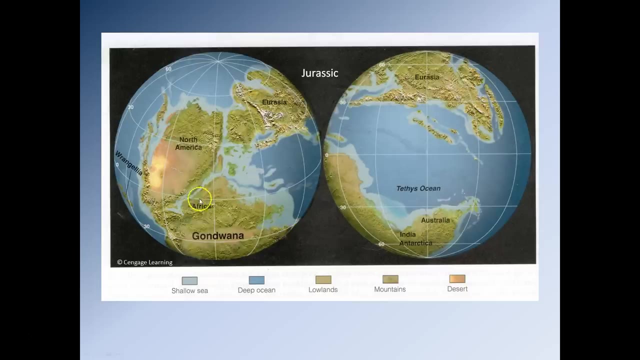 along here, And it continues all the way along here, along the southern margin, well, I should say along here, essentially cutting through the center of Europe. okay, So what this is going to do is is, as Gondwana starts getting pushed this way away from North America, as the North Atlantic opens up, 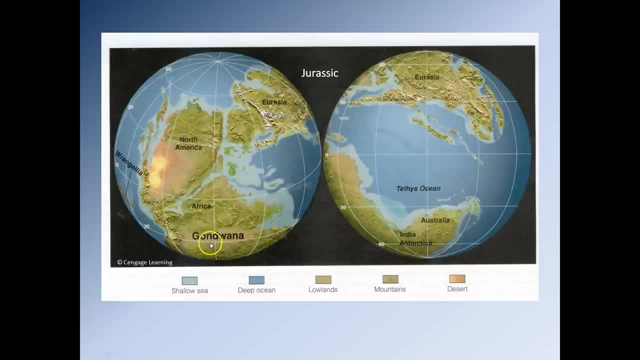 we're going to get South America and Africa start to rift off from each other and then the force, this subduction zone that's running up here, is going to start pulling material in this direction. So it's going to start pulling Africa up towards Europe Now, eventually. 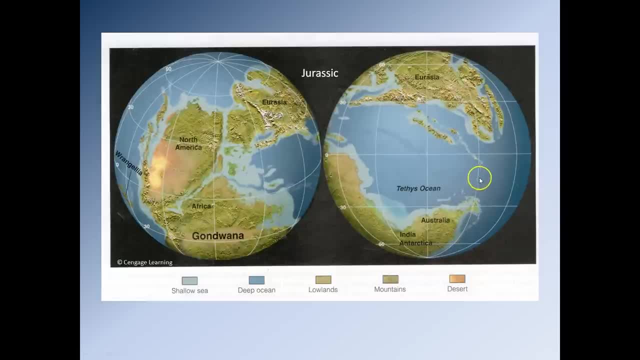 Australia is going to separate from Antarctica and that's going to start being pulled north northwards by the same subduction zone, And India is going to do the same thing. India is around here And India is also. when it separates is also going to start being pulled northwards by the subduction zone running. 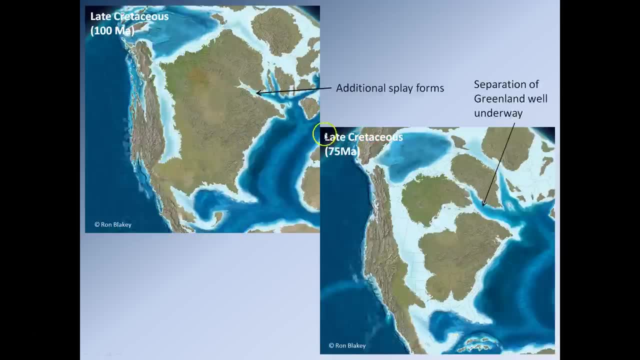 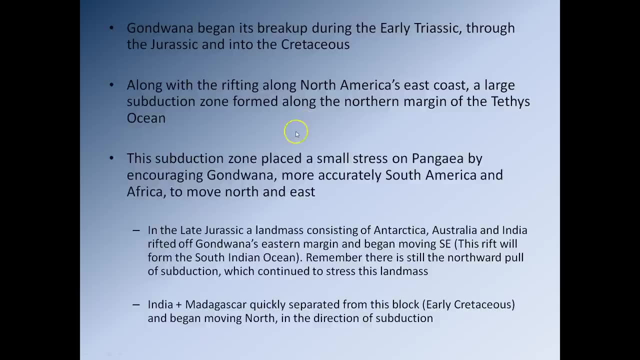 along here. So that subduction zone is quite important because it's explaining what, explains why Africa, India and Australia all start to move there The way they do. So the subduction zone began to place a small stress on Pangea. 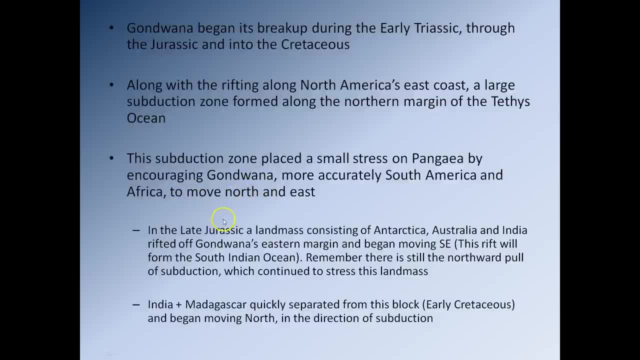 because it was encouraging Gondwana, or more accurately, South America and Africa, to move in the north northeasterly direction. So in the late Jurassic, a landmass consisting of Antarctica, Australia and India rifted off Gondwana's eastern margin. So in the late Jurassic you end up with: 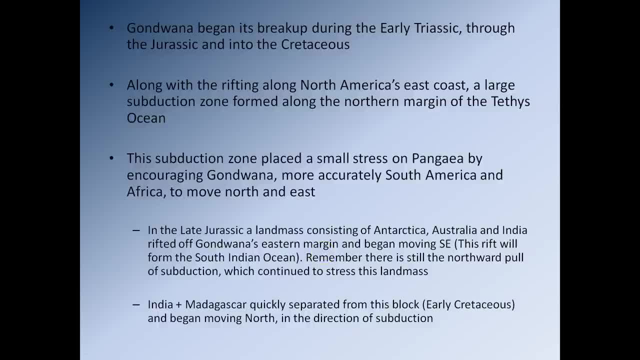 two landmasses. Gondwana splits into two. One landmass is Africa and South America, The other landmass is Australia, India and Antarctica, And they start separating, They start going their own way, And the rift that's pushing them in different directions will now go to form what is now the modern-day Indian Ocean. 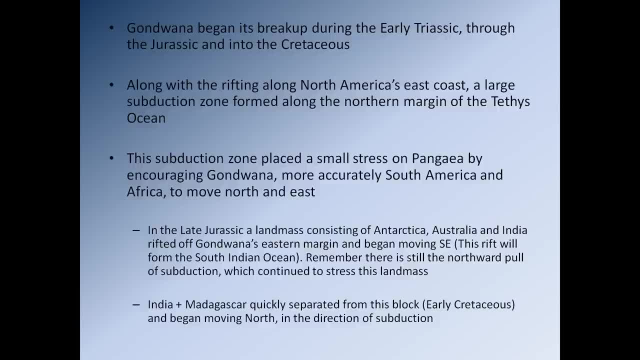 So we also need to remember there's still this northerly pull, though, towards Asia, That's trying to take Africa, India and Australia in an approximately northerly direction. So not long after this rift occurs, we then get the separation of India and Madagascar off this new landmass. 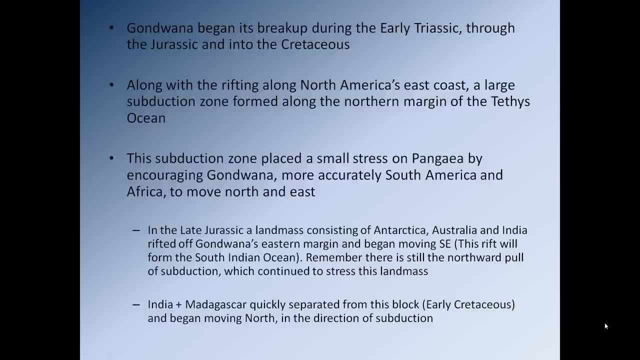 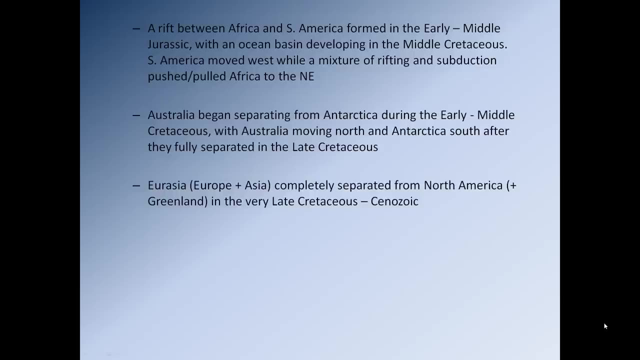 So in the late jurassic we form this landmass of antarctica, australia and india and then in the early cretaceous india and madagascar rift off that landmass and start going off to do their own thing. so in the early to middle jurassic we also begin to see the formation of a rift between: 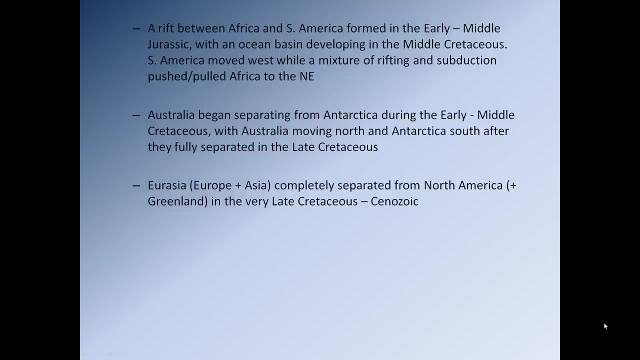 africa and south america and that's going to develop into the south atlantic and we have a complete ocean basin by the middle cretaceous. so by the middle cretaceous, south america is completely separated from africa, so south america starts moving in a westward direction. 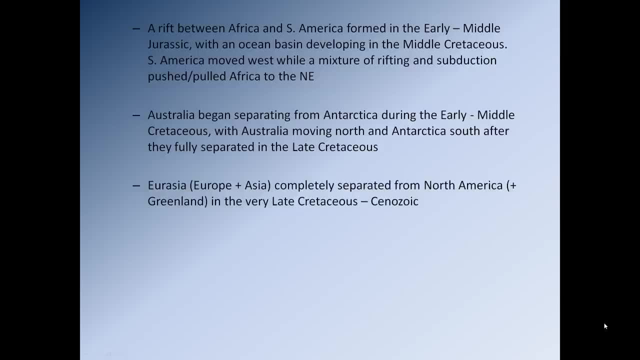 africa starts moving in an eastly direction and of course africa's also being pulled northwards by that subduction zone. australia and antarctica stick together during the all the way through the mesozoic. during the early to middle cretaceous, we begin to see 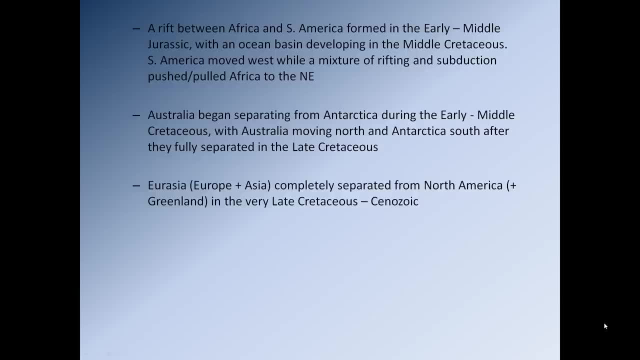 australia wanting to try and move in a northerly direction and antarctica's trying to move in a southerly direction towards the south pole, and so we begin to see that extension of those two continents essentially resulting in the rift, resulting in rifting and full separation by the 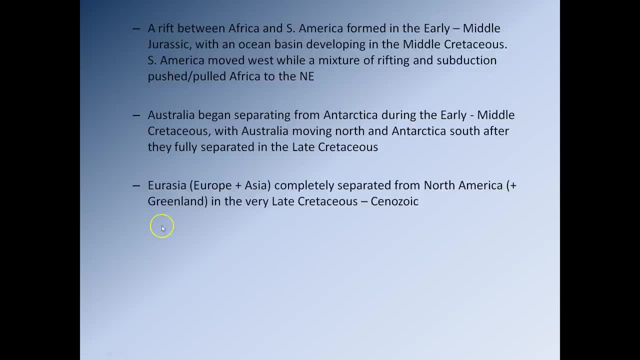 late cretaceous, in terms of north america, europe and asia. well, obviously, europe and asia stay stuck together. that hasn't changed. in terms of north america and europe, the contact between sucha zone, between those two landmasses, well, that contact between those two landmasses is going to be. 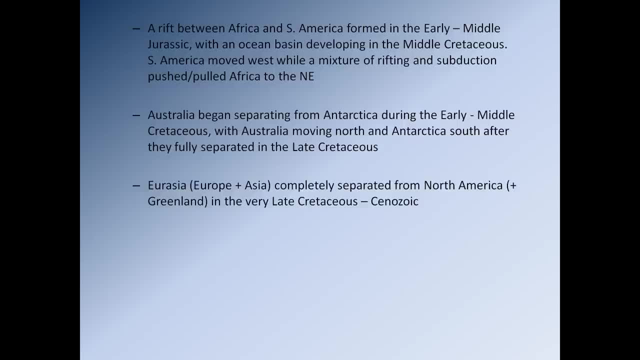 essentially stays complete until depend. you know it's a it's a bit, you know it's a bit. uh, you know bit difficult to work out exactly when the separation completely occurred, but the essentially, the suture zone between north america and europe is intact until, literally either the very, very 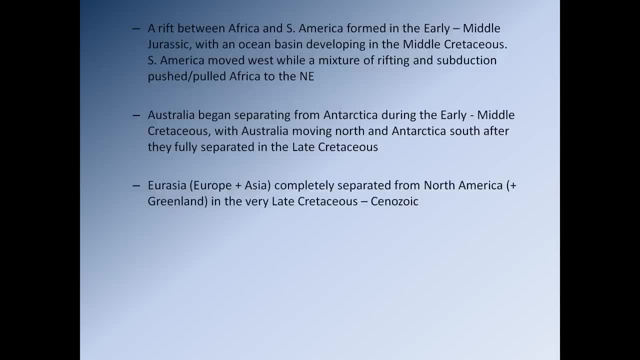 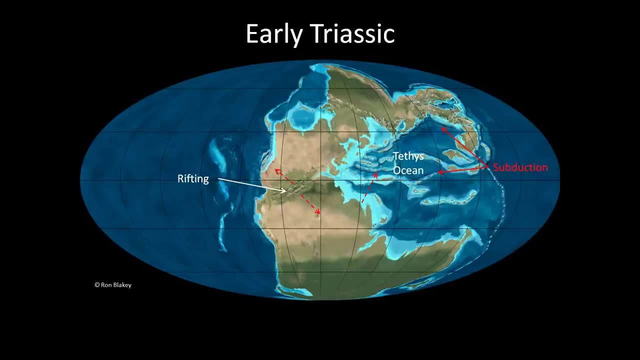 last minute of the cretaceous or maybe just into the cenozoic. okay, so it's been 20 minutes, so let's pause now and then, when you come back, we will have a look at these maps here, which is going to demonstrate how the con, you know how, uh how- pangaea fell to pieces. all right, so pause the presentation. 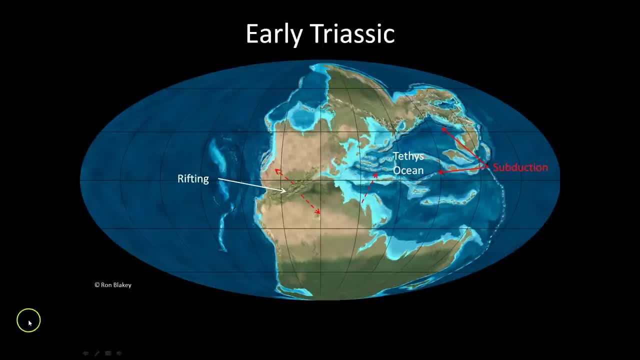 uh, going a glass of water, have a walk around, relax for a few minutes and then please come back, okay? so this is the situation in the early tratic. so here we have pangaea, so we've got asia over here, the ural mountains here. this is europe, north america's, here we have south america, here. 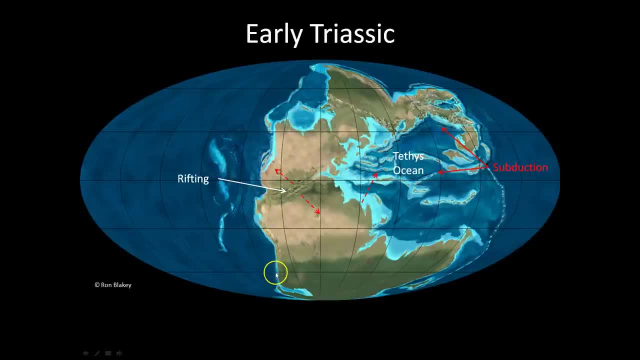 in fact you can just kind of make up the west coast of south america. there we have africa here. so here's west, here's that kind of the northwestern africa. it's going to come around like this: come around here. so this is going to be saudi arabia, here egypt's going to be. 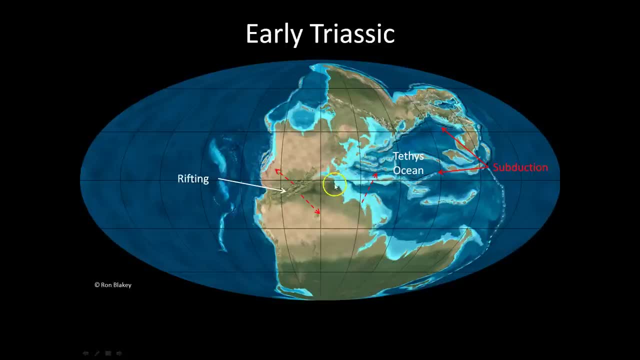 around here. libya, north africa is going to be around here, the southern, north, southern coast of the mediterranean, we have india about here, we have australia over here and we have antarctica down here. so, the early trassic: what starts happening? well, to begin with, we have the teffis ocean here. 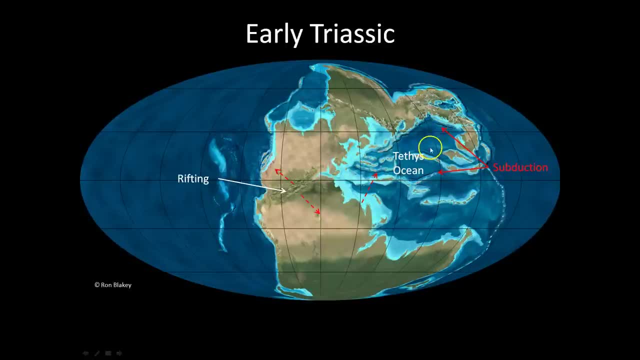 and we start forming several subduction zones on the northern margin of the teffis ocean, and so this is going to start taking all of this oceanic crust here and it's going to start pulling it in this direction and it's going to start stretching all the pieces of crust that the 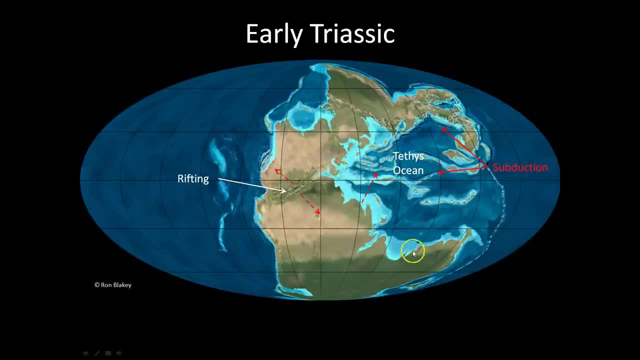 well, it's going to start taking all the pieces of crust that it's attached to with it. so you know, africa, india, australia, antarctica- they're all going to start being pulled in this direction now. at the same time, we have the rift opening up here between north america. 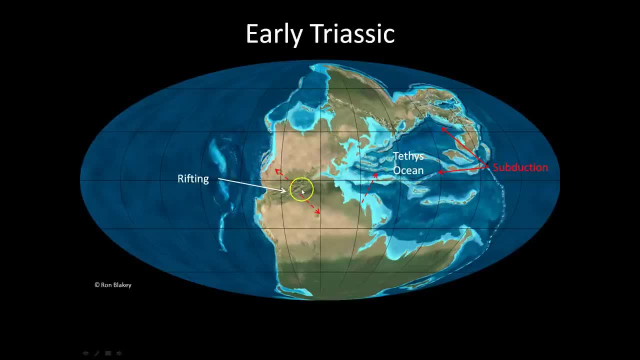 and well, what is now modern day, south america and africa, and that's going to start pushing this entire landmass towards the southeast. so we have two forces operating on gone, operating on gondwana, one pushing southeast and one pulling northeast. at the same time, we obviously 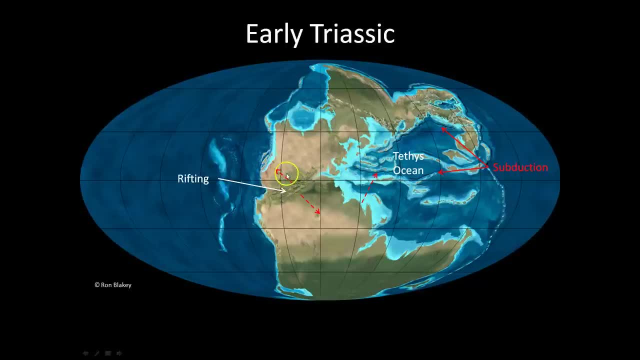 have this pushing force now due to the creation of the north atlantic and that's going to start pushing north america this way and obviously, as europe and asia is still attached to it, they're going to go with it and they're going to rotate a little bit as they go. so, by the late trassic, what's going on? 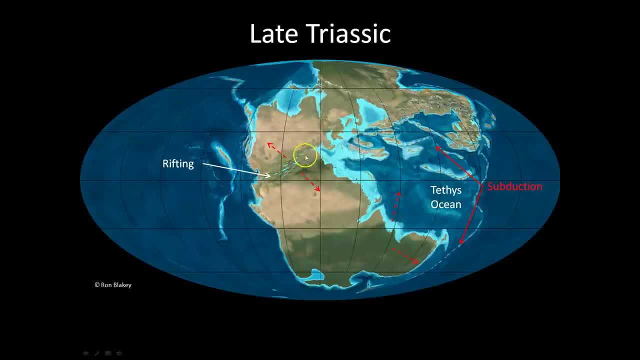 well, the rift here between north america and gondwana is developing nicely and it's slowly but surely beginning to fill up with water- still not a complete oceanic basin yet. we still don't really have oceanic crust being made. now, you can see, by this point. let me just go. 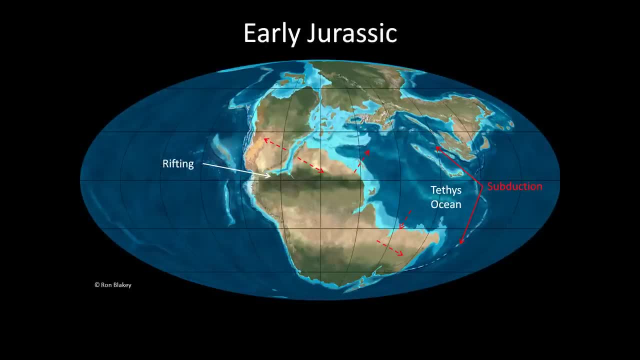 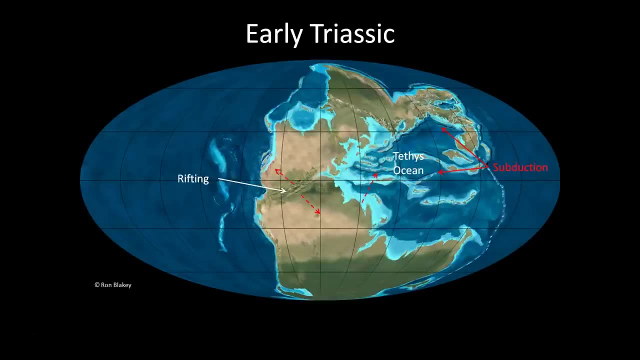 over to the left here for a second. we can see there hasn't been too much movement from the uh, from sorry from the going the wrong way, sorry from the late, from the early trantic into the the late trassic. but you can see there is a little bit of movement there along the north coast here. 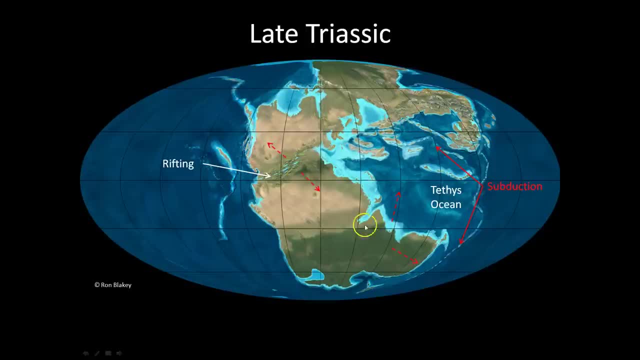 of gondwana, but by the late trassic, this rift is developing, it's still pushing north america this way, gondwana this way, and these subduction zones over here are still operating, and they're still India and Australia in this direction. Now, the most important thing, though, is we also have 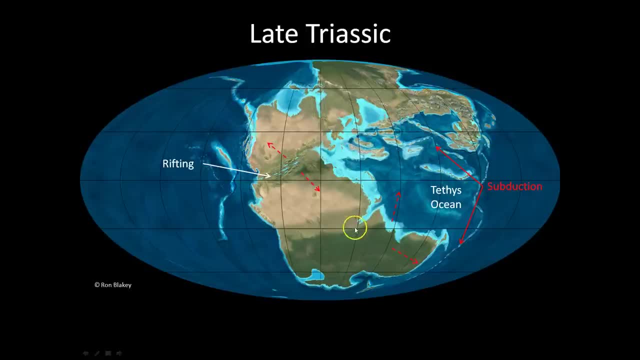 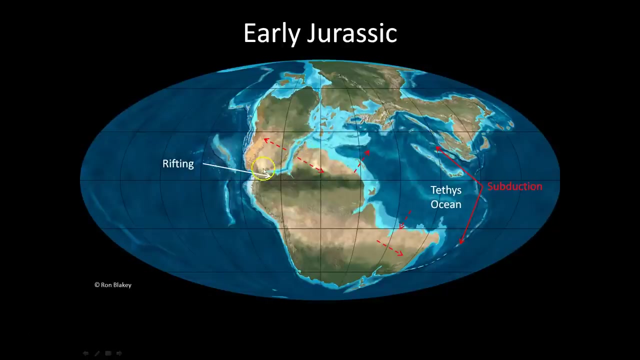 another rift opening up here, okay, and this rift is going to develop and it's going to separate India, Australia and Antarctica from South America and Africa. So as we move into the early Jurassic, we now have a fully formed rift between North America and Gondwana. So now we have the North 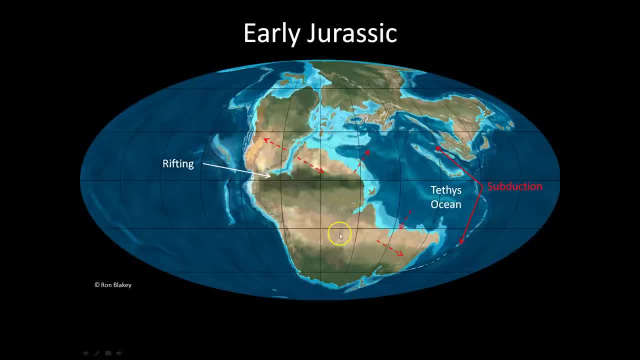 Atlantic Gulf Coast region is down here. We now have this rift beginning to further develop here between Africa- India, so it's going to slowly cut down here, it's going to separate off India, Australia and Antarctica, and once again, though, we still have these subduction zones working up here. 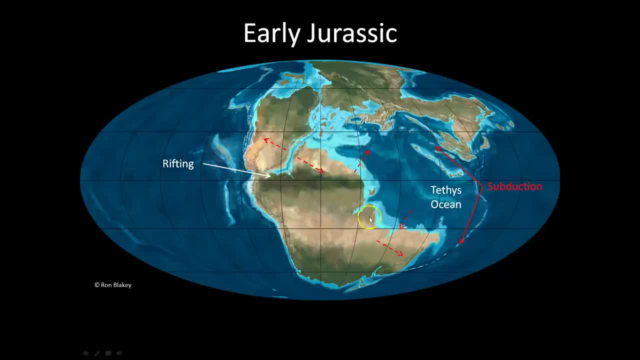 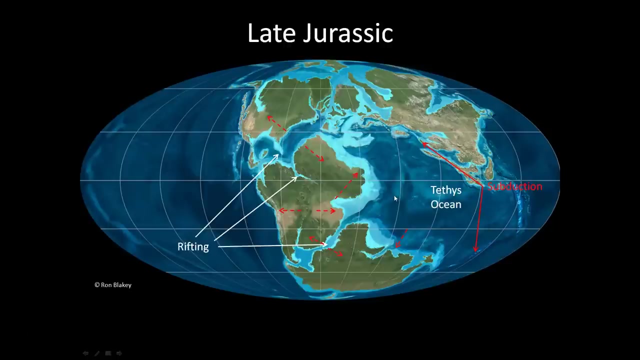 and they are still going to be pulling Africa, India and Australia. They're going to try and be making going to try and make them move in an approximately north northeast direction By the late Jurassic. you can see, okay, now we have most of the continents beginning to. 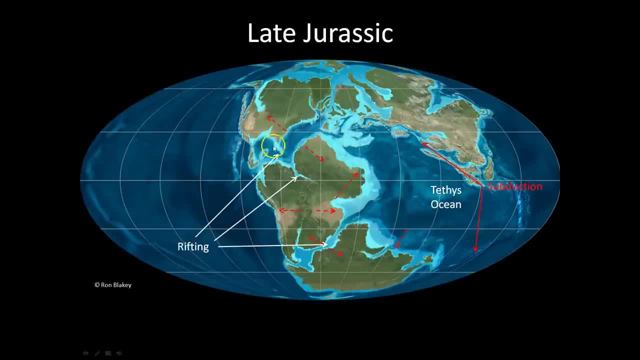 separate away from each other. Okay, so the North Atlantic and Gulf and Gulf Coast and Gulf region has opened up nicely. We now have the start of rifting between South America and Africa. You can begin to actually see South America and Africa properly now. We have a fully formed rift here. 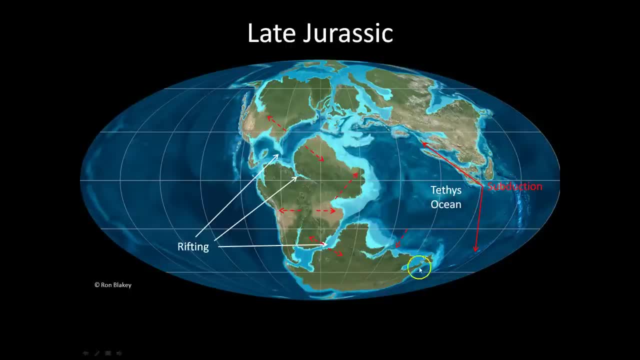 that's now separated off India, Antarctica and Australia, And we have a fully formed rift here that's now separated off India, Antarctica and Australia, And we have a fully formed rift here that's now separated off India, Antarctica and Australia. We can see the rift between India- well, this is actually India plus Madagascar- is now slowly. 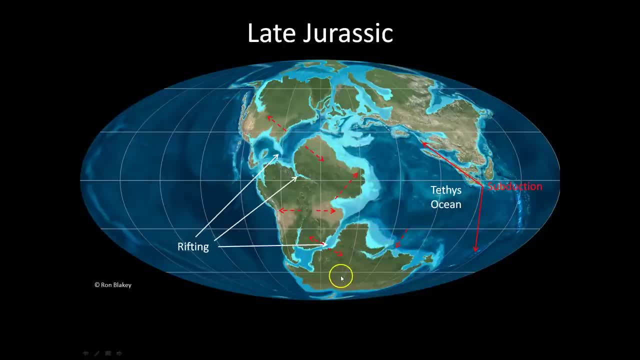 starting to rift off the side of Antarctica. Once again, we have the subduction zones here. These subduction zones are pulling Africa in a northerly direction, They're trying to pull India in a northerly direction and they're trying to take Australia in a northerly direction. 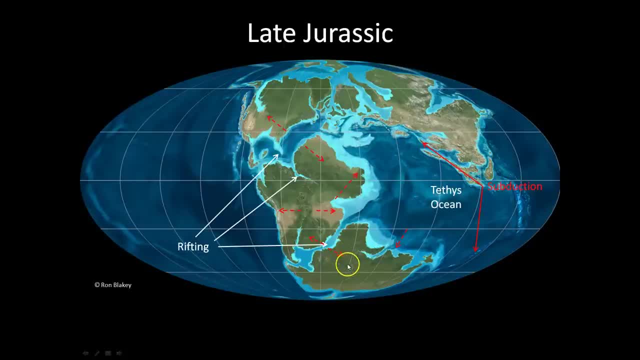 Now, this rift here, though, is taking Antarctica and Australia in an approximately south, southeasty direction. This rift here is going to start pulling, pushing South America this way and Africa this way, So what you can see is you can see that Africa is essentially being pushed both this way and pulled. 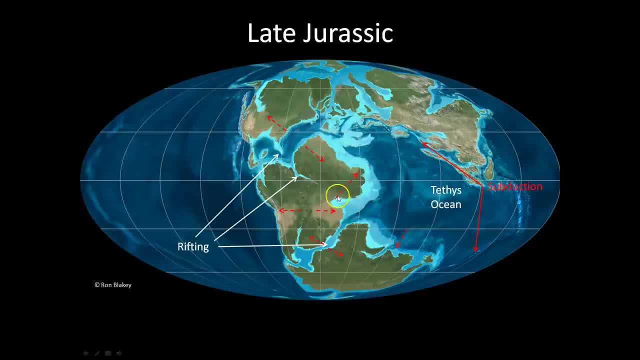 this way. So it's going to start rotating towards its current position. So this this, this corner here is going to start coming up, It's going to start hinging around here and it's going to start sweeping up, and so it's until it's in its modern orientation, So by the early Cretaceous period. 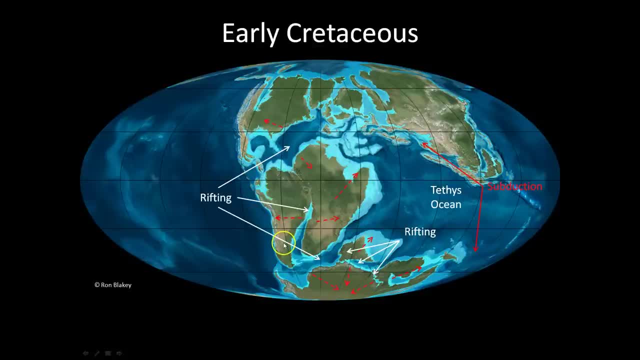 this rift between Africa and South America is developing nicely. We have a nice ocean basin here between Africa and India, Antarctica, Australia, So- but at this point India is now fully separated and it's going to start going on its journey towards Asia because of this. 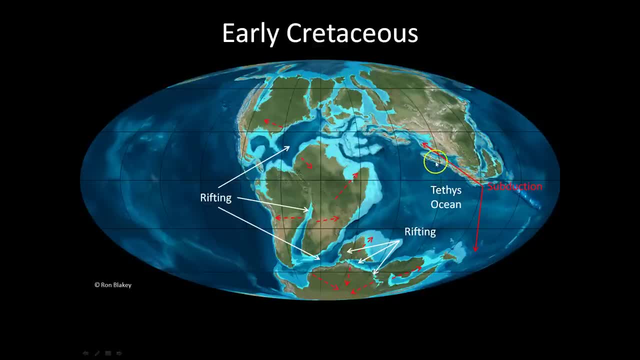 subduction zone here pulling the oceanic crust this way. Once again, the subduction zones along. here is pulling Africa, trying to make Africa move in a northerly direction, Still attached to South America, so it's still not quite there yet- Antarctica is now trying to move straight towards the South Pole and at this point you can see the 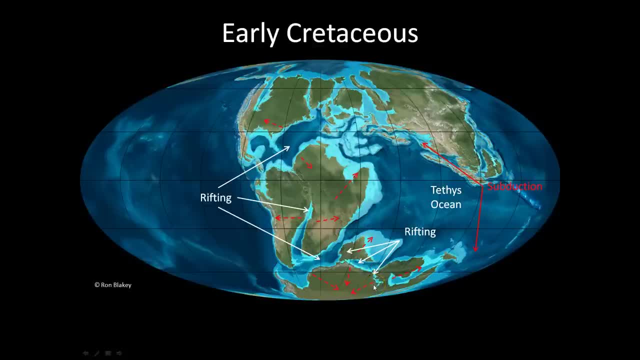 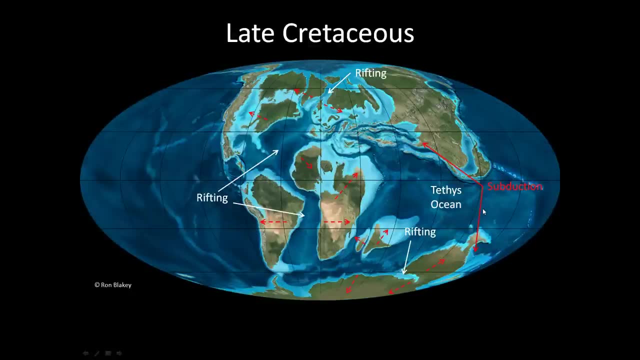 rift between Australia and Antarctica is beginning to form because Australia is still wanting to move in a northerly direction along with India And by the time we're into the late Cretaceous, we have full separation of South America and Africa and the formation of the South Atlantic. 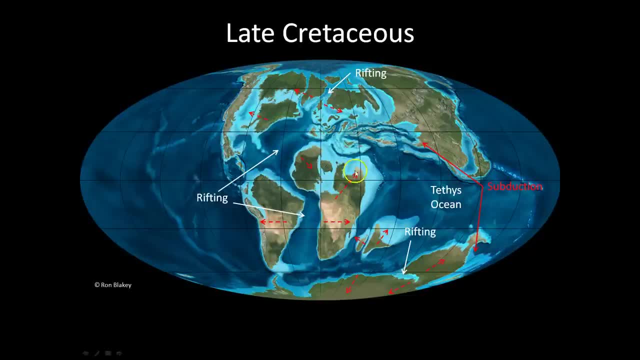 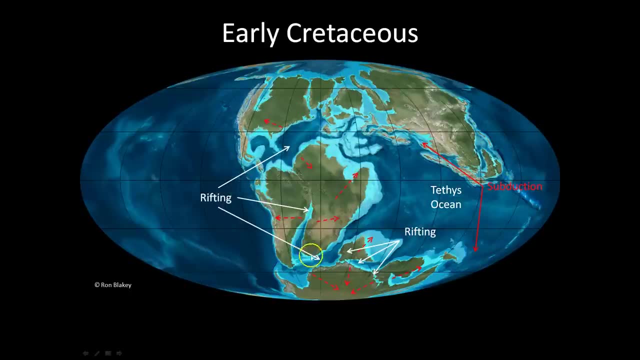 Now this means that Africa can now move this way and this way. You will have noticed as we go, as we go back to the previous slide- sorry- you'll notice that it's begun to rotate. So look at the southern tip here of Africa. You'll see it starts off over here, and by the late 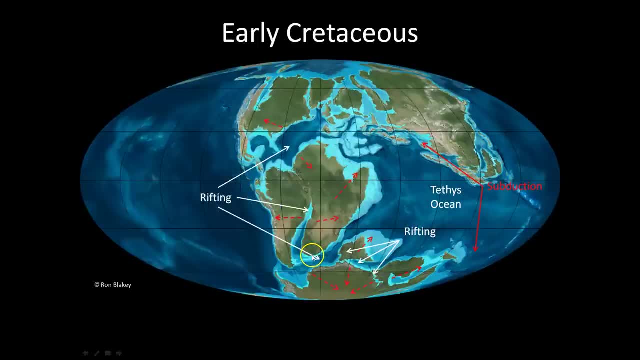 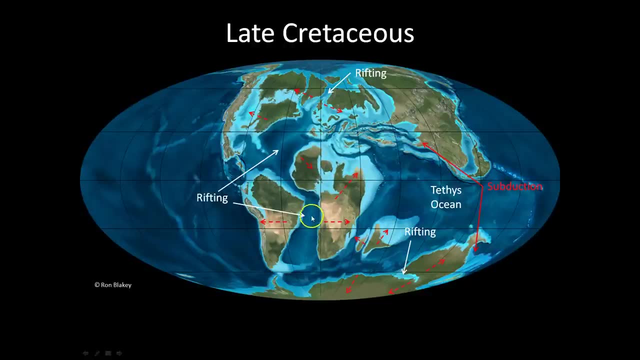 Cretaceous is over here, So you can see the continent's beginning to rotate slightly. So it's rotating around here and the southern point and this eastern side is coming up like this. That's because it's being pushed this way and pulled this way. We can see, by the late Cretaceous. 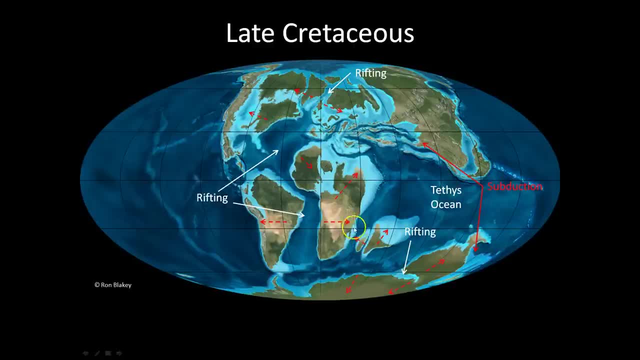 Madagascar is separated off India and it's going to essentially stick. it's going to move towards Africa, Where it's going to essentially stick itself onto the side of Africa, and that's going to be it until the present day. India is now going to start moving towards Asia and I want you to take notice of all of this. 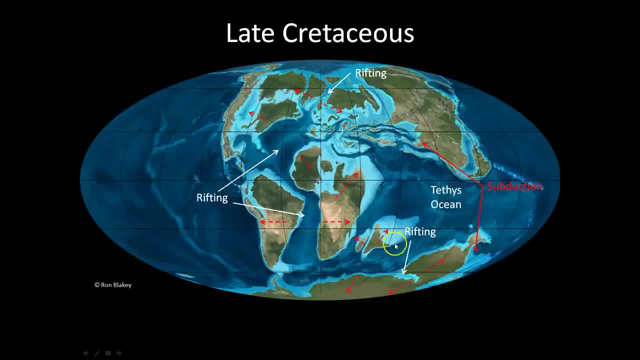 continental shelf to the north of India. All of this continental crust here that's underwater, Okay, so this is about the size of modern India here. So all of this material here is going to get squished when it hits Asia and that's what's going to form the Himalayas By the late Cretaceous you. 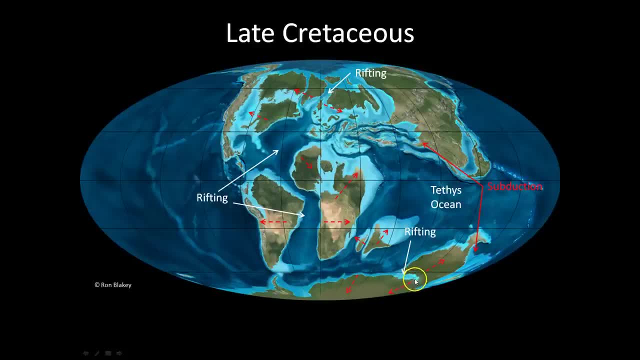 can see, Australia is going to start moving towards Asia and that's what's going to form the Himalayas. Australia is nearly completely separated from Antarctica. By the end, by the very end of the Cretaceous, it will be a separate land mass in its own right and it will be moving towards the north. 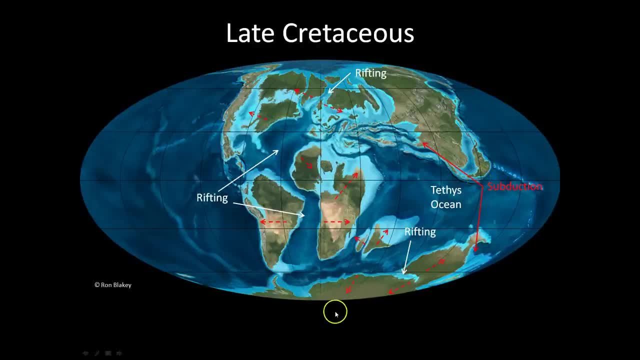 Antarctica is trying to move over the south pole. it's nearly completely there, As we can see up here. by this point we can see we have these rifts developing nicely. So North America and Europe are nearly completely rifted off each other and the rift is developing nicely between Greenland and North America. So you can see by the Lake. 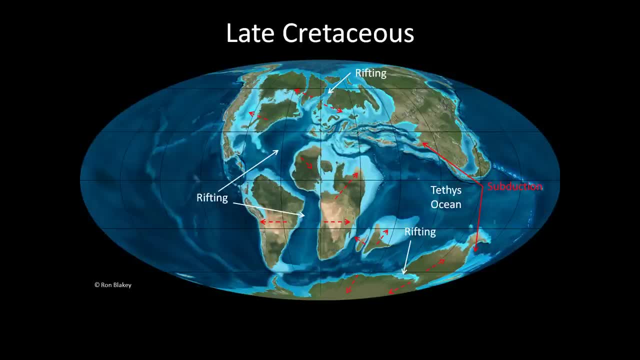 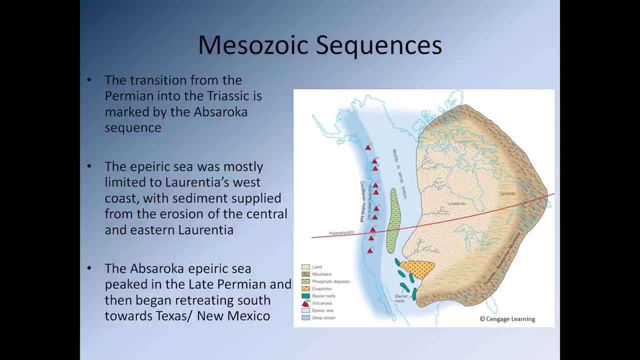 Pet Hamp that we are not right across Antarctica. When we go through the Porto, interacting with these rifts, we're essentially going to seeなら❤️. We have essentially the the modern continents around. We can see where they are and we can see. 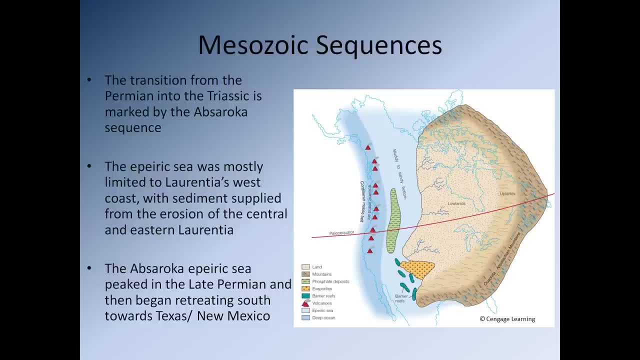 approximately where they're going. So Okay, so now let's focus in on North America and let's start thinking about the Mesozoic sequences. Let's start thinking about, you know, these shallow bodies of water that form on North America during the Mesozoic. 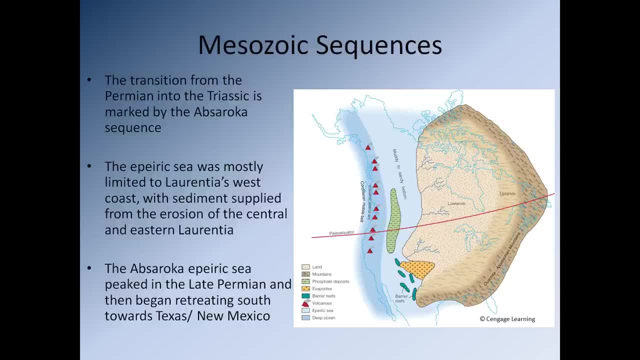 the boundary between the Permian and the Triassic, So the Absaroka-Pyrrhic Sea was mostly limited to Laurentia's west coast and southern margin. it will take a little bit. So if you remember the Soak, the Tippecanoe and the Kazkazkia. 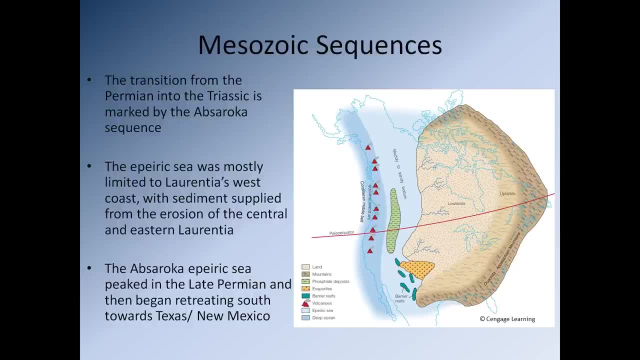 those marine transgressions resulted in the near complete coverage of North America by water. So, if you remember, for both of those three sequences the United States was completely underwater and a significant portion of Canada was underwater, And so this meant the supply of detrital sediment- clastic sediment, was severely limited. 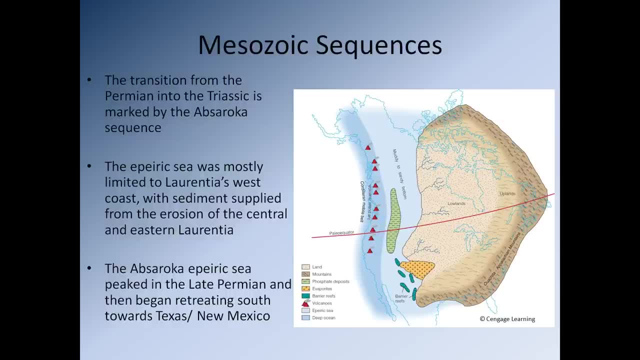 because there wasn't that much land above sea level which could be eroded. So that means that the water that was being, that means there wasn't much clastic sediment being dropped by rivers into those Epiric Seas, into the Soak Epiric Sea, the Tippecanoe Epiric Sea. 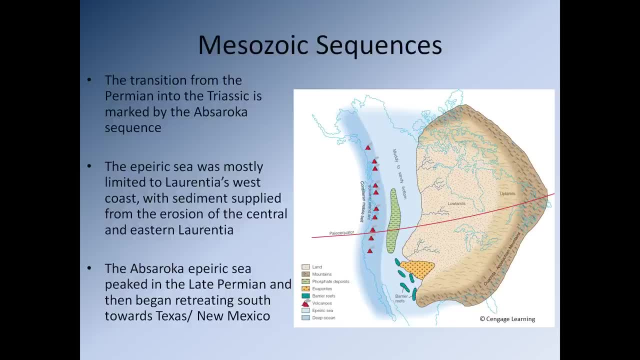 and the Kazkazkia Epiric Sea, And so this means that the water quality for those Epiric Seas was extremely clear. it was shallow water, they were situated over the equator, so it was warm water, and so that meant huge quantities of carbonates were deposited during those three marine transgressions. 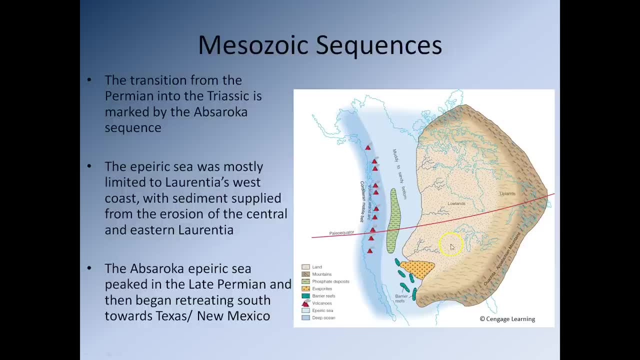 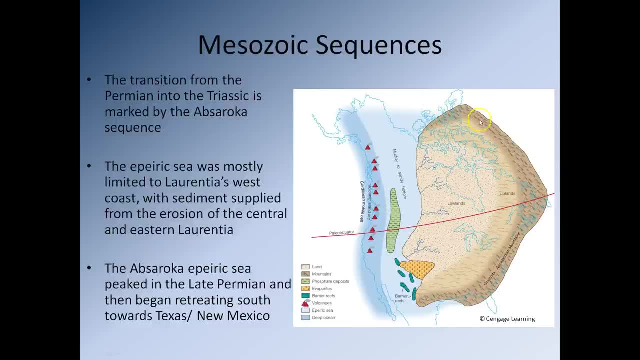 We also had the remains of North America above sea level. We saw the remains of the Iñ öğitian orogeny up here, the Caledonian orogeny over here, the Appalachian Mobar Belt here, the Achitin Mobar Belt down here. 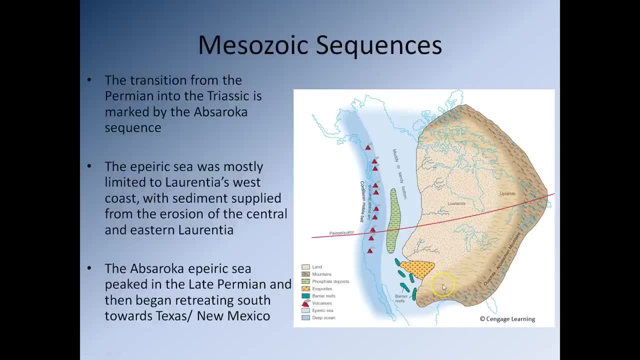 and the Proto Roqu'is down here. So essentially, what we have is choose. Richard A Rook's version of oxford farm joke is we have a situation where we have loads of high ground. high ground will naturally be eroded very, very quickly, producing huge quantities of sediment. 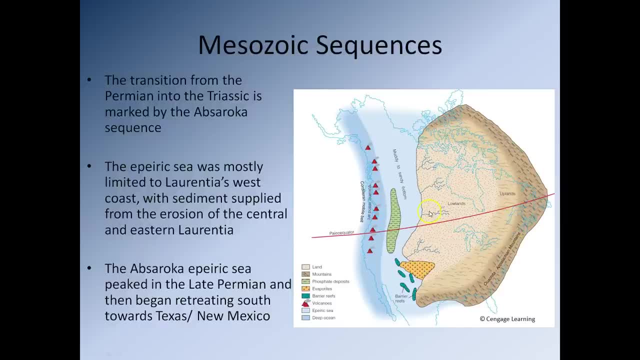 then we had a plain, essentially, which would have been covered by mass sediment, by massive rivers that would have transported all that eroded sediment from these upland areas and deposited into the Absaroka Epiric Sea, and so this means the Absaroka Epiric Sea had huge quantities. 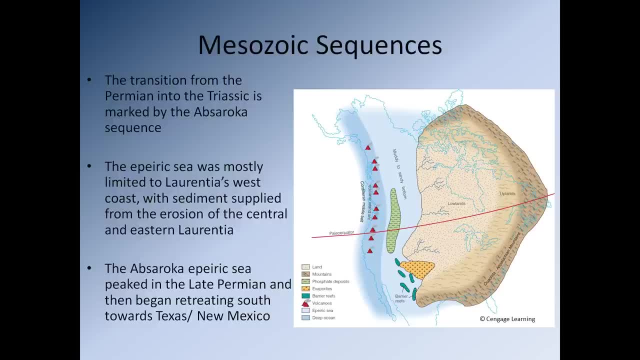 of clastic sediments going into it, so the water quality was nowhere near as good as the water quality that occurred during the soak, the tipper canoe and the Kaskaskia. So that's why we don't see large-scale carbonate formation during the Absaroka Epiric, during the Absaroka. 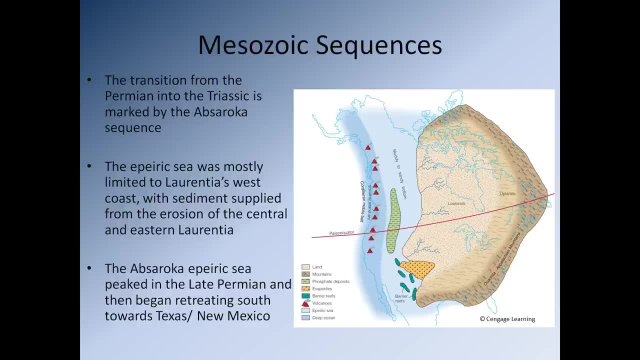 as part of the Absaroka sequence, because the water quality was nowhere near as good. We do see limited carbonate formation down in this southwesterly corner down here. This is the area where water quality was probably at its best, and so we see carbonates. 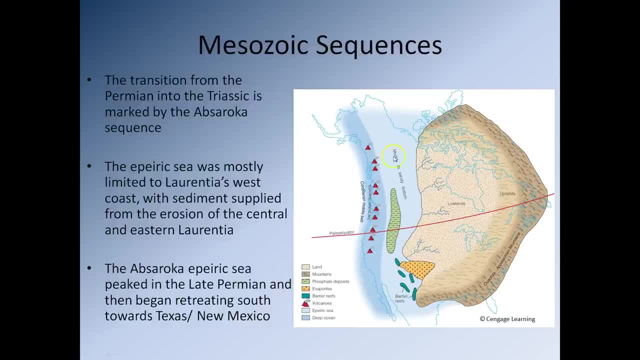 forming down here. However, the rest of this area here that that's going to be dominated by clastic sediments. so we're going to see lots of sandstones, lots of mudstones in this area here, a little bit of a few carbonates forming down here. 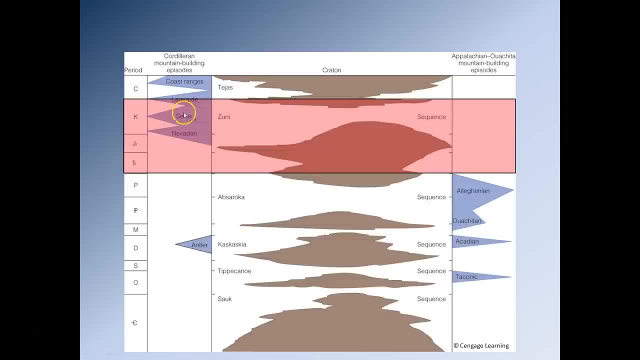 so here we go. so this is the mesazurk here marked out in red, and we can see the mesazurk itself. we're still in the last stages of the absaroka sequence. we can see the absaroka epirxy has been. 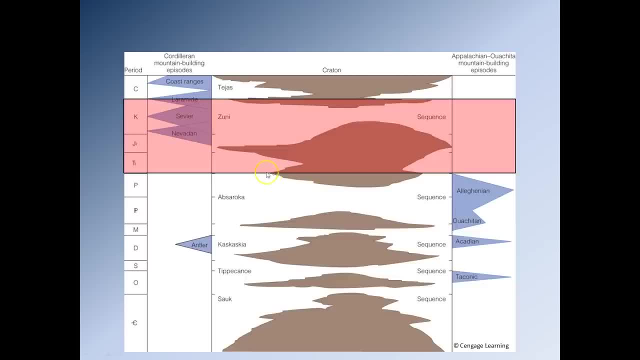 retreating all the way through the permian and by the time we make it to the permian trassic boundary, you know, about half of north america is exposed. there's going to the tracet, there's going to be a small marine transgression followed by a very large regression. and at this point, during the 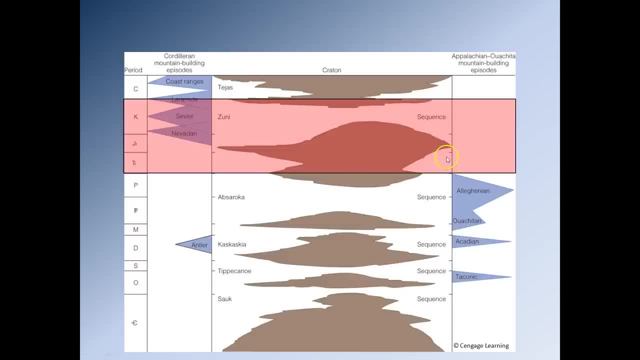 middle of the jurassic nearly all of north america is going to be exposed to, so it's going to be actively eroded and then, as we move from the middle jurassic into the cretaceous, we're going to steadily see a large-scale marine transgression and we're going to see the formation of the zuni. 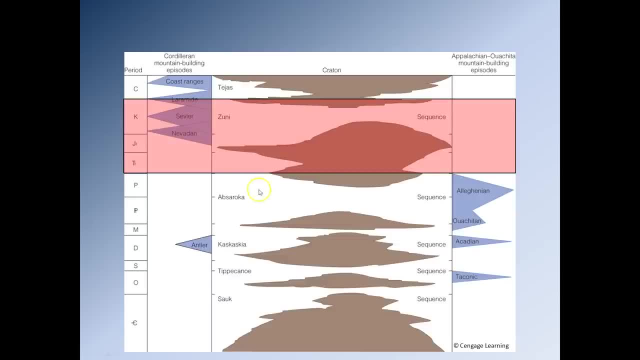 sequence and the zuni epirxy. you'll also notice that during this period we have no orogenies on the east coast, because that area is undergoing active extension, it's being stretched, so that means no convergent plate boundaries, so no mountain range formation. on the other hand, on the west coast, during the 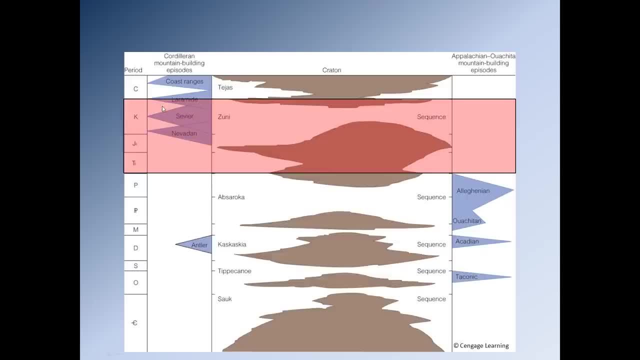 mesazurk. the west coast during the mesazurk is nearly a non-stop subduction zone, and so that means there's lots of stuff hitting the west coast during the mesazurk, and so that leads to the formation of the nevadian sevier and laramide orogenies. 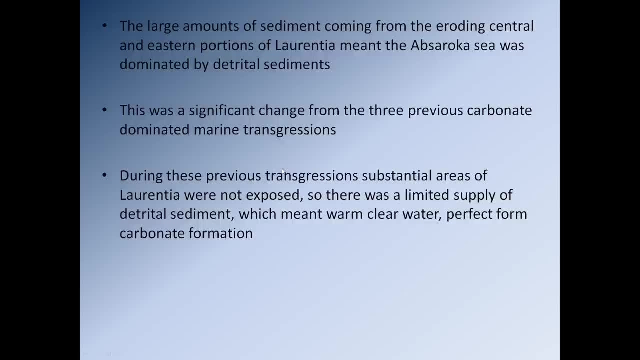 so the large amounts of sediment coming from the eroding central and eastern portions of that should say, north america meant the absaroka sea was dominated by detrital sediments and obviously, as i mentioned, that's a that's a significant change in sedimentation compared to. 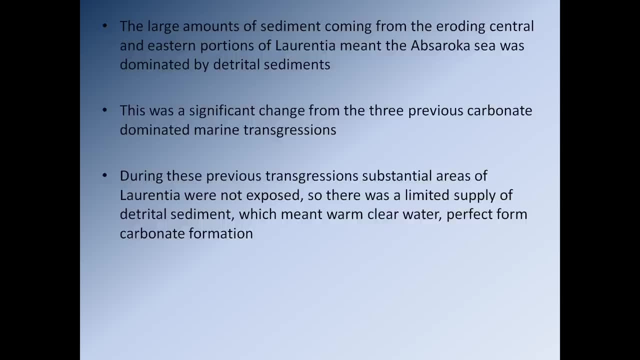 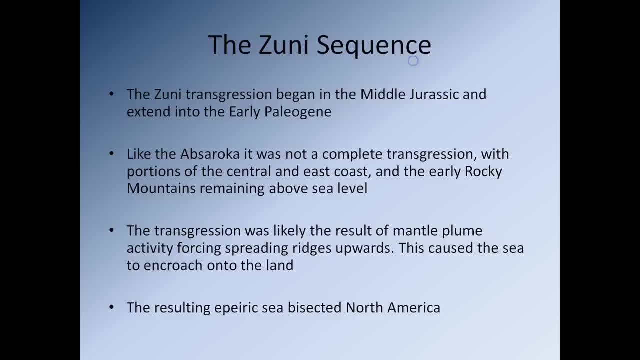 so the left-hand corner apparel here in the right corner. our warnings and the are very simple. normally, suni 있고요 could occur at the正続 flora sea land on the azure tri accredited region, the middle jupiter ocean and breast, or was that okay and they were? actuallyAll of them in the old detalestra here in the western going toолько is also Baku, so currently there's a four million. there are very, a lot of resões he. then there's another zone in �baum or preهleди. we have a very dense energy zone, but the the this building has then 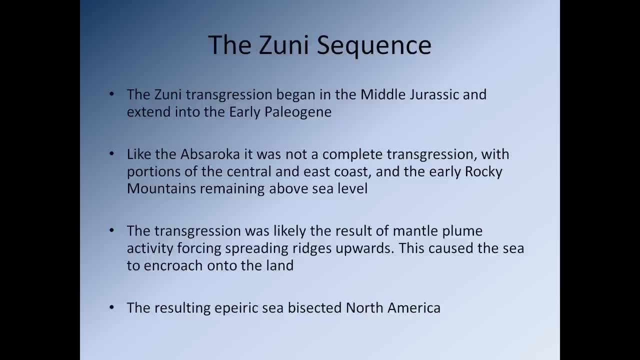 the Absaroka. it was not a complete transgression, so portions of central and the central North America and the east coast of North America and the early Rockies remained above sea level throughout the Zuni sequence. So this means that once again we're going to have quite a bit of 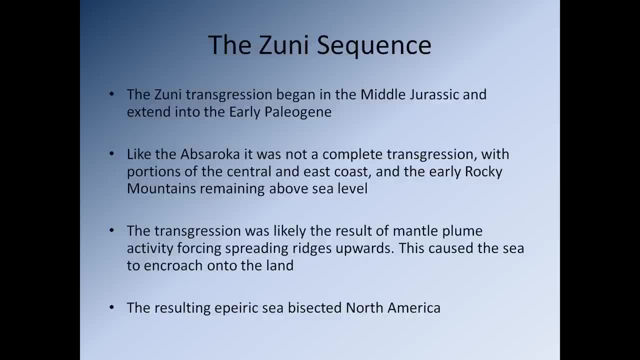 plastic sediment produced, so we're not going to see huge quantities of carbonate produced during the Zuni sequence. So what causes the Zuni sequence? Well, the Zuni sequence was likely the result of mantle plume activity forcing spreading ridges upwards, So it looks like 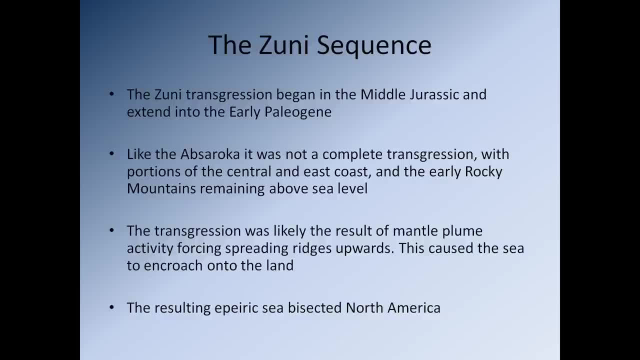 during the Cretaceous especially, there was a lot of magma that got trapped underneath spreading ridges, you know in the ocean basins. We think that most of this magma was trapped. that got trapped was from hot spots, so mantle plumes. So we think that during the Cretaceous there was a. 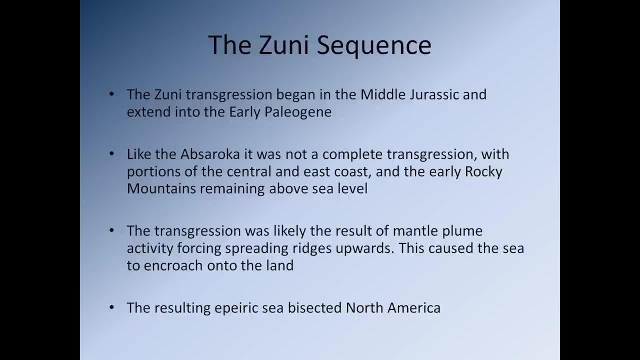 huge amount of magma that got trapped underneath spreading ridges. So we think that during the Cretaceous there was a huge amount of magma that got trapped underneath spreading ridges. So we huge mantle plume activity that meant you had these big balls of magma that came flying from. 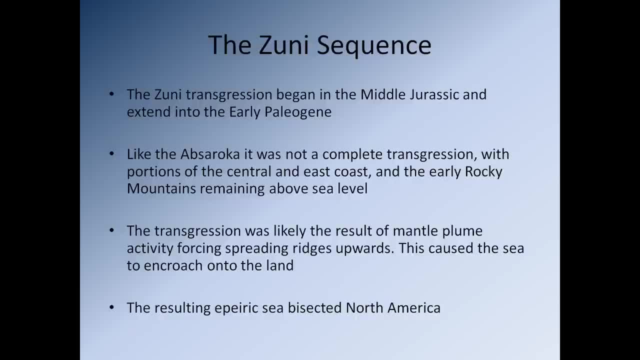 the core mantle boundary all the way up through the mantle and they got stuck at the base of the crust and they tended to get stuck under spreading ridges. And obviously, these balls of magma, they're very, very buoyant, they want to rise and so they push up the crust above them, they make it dome up. 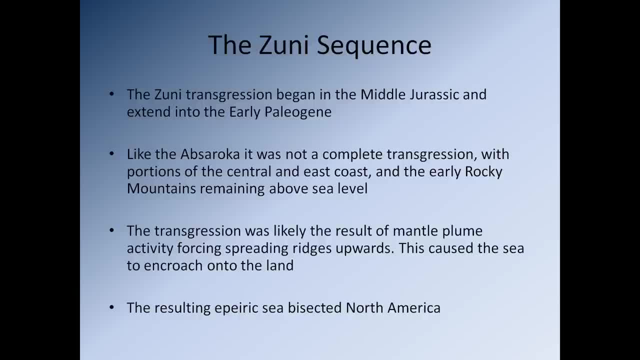 And so, essentially, what that means is, when you have all these- you know, all these mantle plumes stuck underneath the spreading ridges, well, they're going to push up the spreading ridges. And as they push up the spreading ridges, well, that means they're going to start displacing. 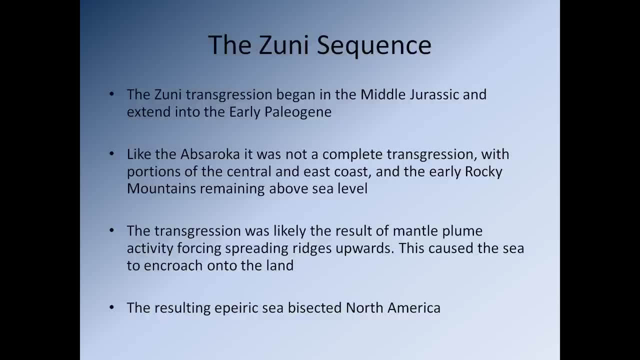 water And as they begin to displace the water, well, that water has to go somewhere and so it goes onto the land. And just to give you some idea, as I think I mentioned already, the sea level during the Cretaceous especially is predicted to have been about 250 meters higher than the 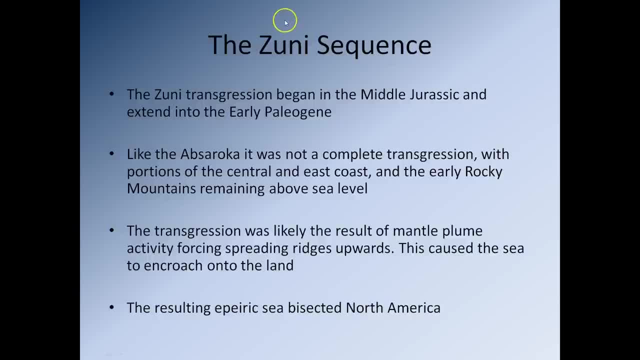 present day sea level. So obviously this movement of water onto the land is going to be very, very impressive. You can actually see that in the picture on the right. this is an example of which is this transformation that took place in the Cretaceous, And, of course, this was only a mere 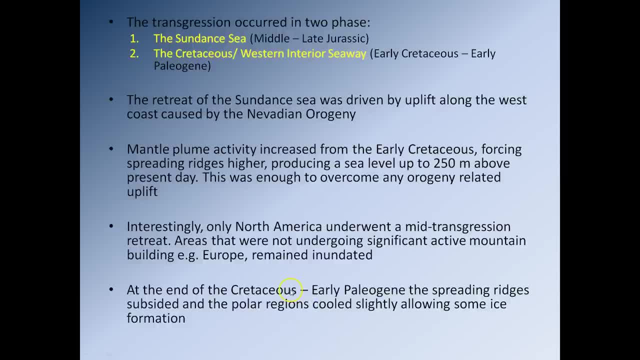 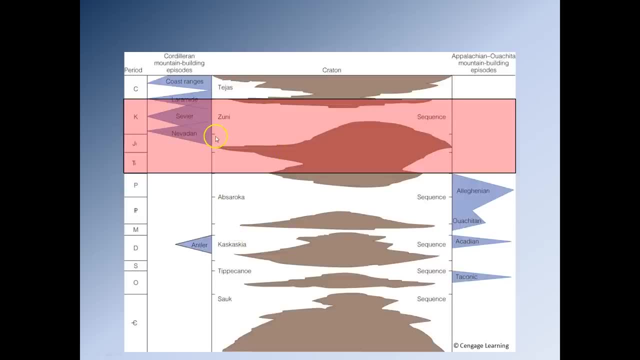 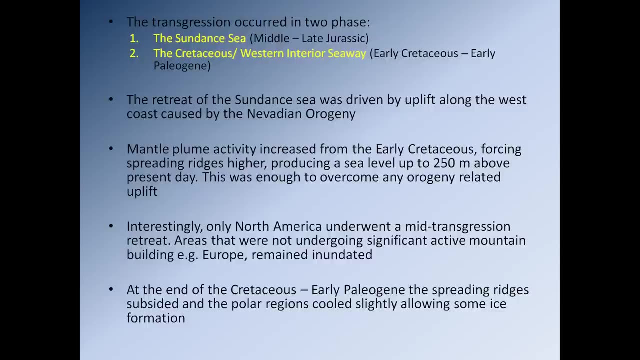 fraction, because the land resulted in the formation of the Zuni Epiric Sea in North America. So the transgression that was part of the Zuni Sequence actually took place in two phases. So if we just go back to this diagram here you can see it makes it look like the Zuni is just one smooth. 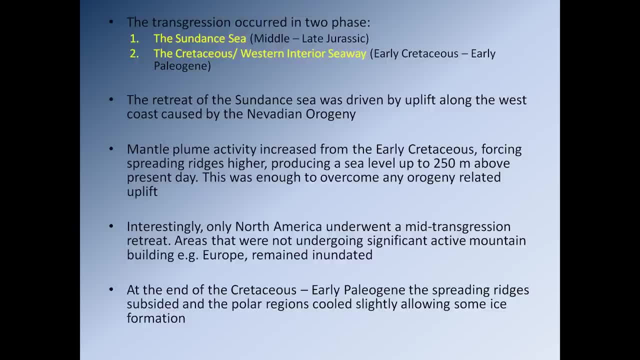 event. well, actually it's not. It actually takes place in two parts. the first portion of it produces what's referred to as the Sundan Sea, And that occurs between the middle and the lower Cretaceous late jurassic. the second part of it is formed what's referred to as the cretaceous interior. 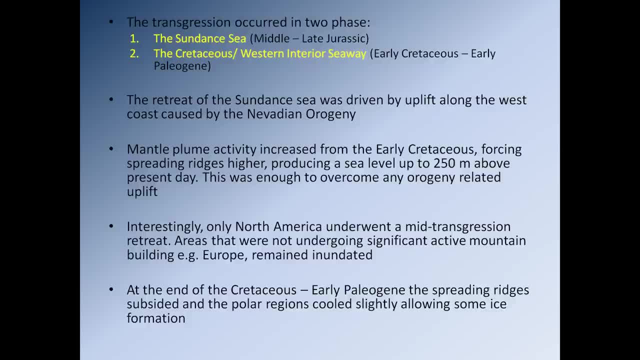 seaway, also sometimes referred to as the western interior seaway, and that goes from the early cretaceous to the very early paleogene, so it makes it all the way into the, the cenozoic. so the retreat of the sundan sea was driven by uplift along the west coast caused by the 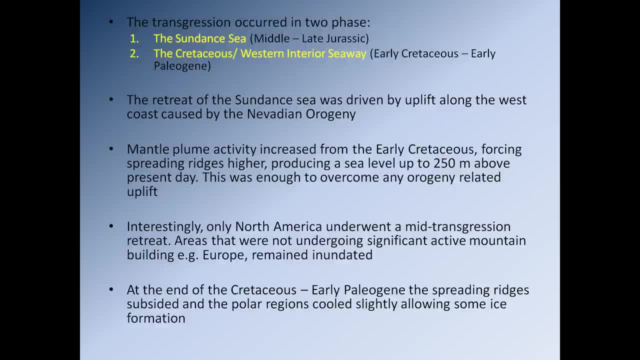 nevardian orogeny. so what happens is is we get this marine transgression right at the, you know, during the. well, should i say we get this marine transgression that forms the start of the zuni sequence and that inundates the western side of modern day north america, so the west side of 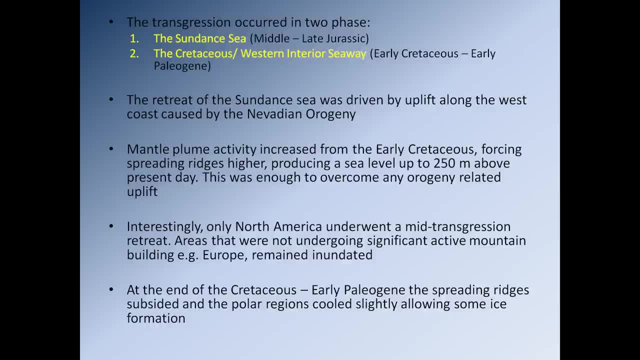 modern day north america is underwater, then what happens is we get the nevardian orogeny forming and that starts to form the first stages of the rocky mountains. and so what we see is we see the west coast starts being pushed up as the rocky mountains start forming. well as that, obviously that land starts to go up. 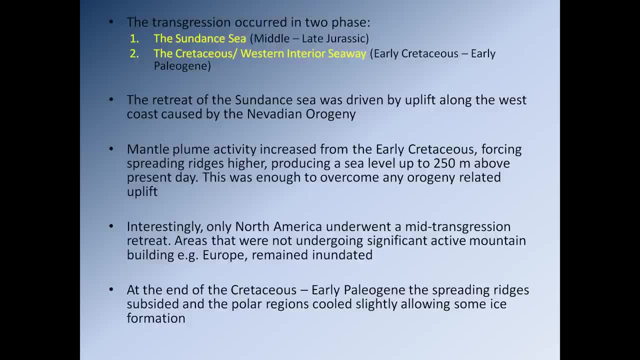 it means there's. it means the epiric sea on it obviously has to start draining away into the pacific ocean, and that's exactly what it does now. what then happens is, during the cretaceous, we get this sudden burst of mantle plume activity. those mantle plumes get stuck. 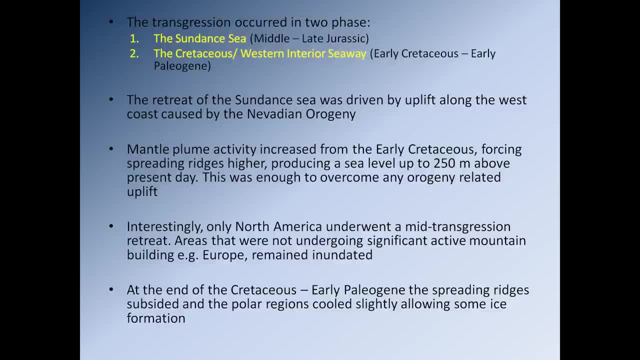 under the spreading ridges. they push the spreading ridges higher and that results in that 250 meter increase in global sea level, and that's when we get the nevardian orogeny forming, and so that very significant increase in sea level is sufficient to allow the water to go back. 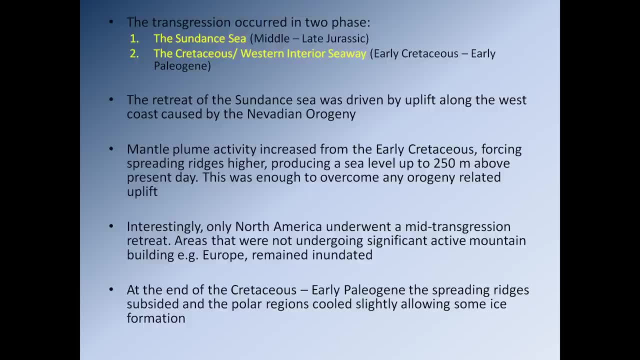 onto north america, especially along the west coast. so you know that that increase in sea levels is enough to overcome the uplift of the west coast caused by the formation of the rocky mountains. interestingly, only north america underwent a mid-transgression retreat. everywhere else in the world didn't really undergo a retreat because you know, nowhere else in the world was undergoing. 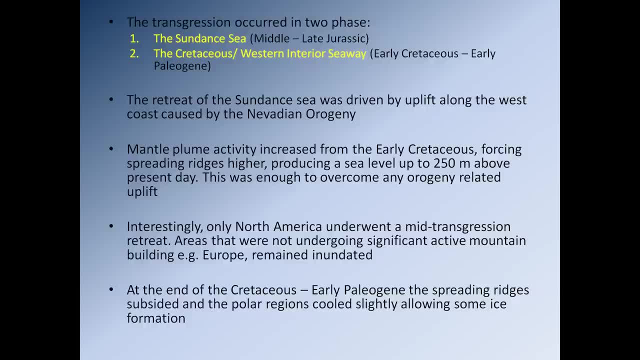 a mountain building, like in the area of the modern day rockies. so, for instance, europe, during the during the meseric, spent nearly the entire uh spent nearly the entire time underwater. so at the end of the cretaceous and into the early paleogene we see the spreading ridges begin to. 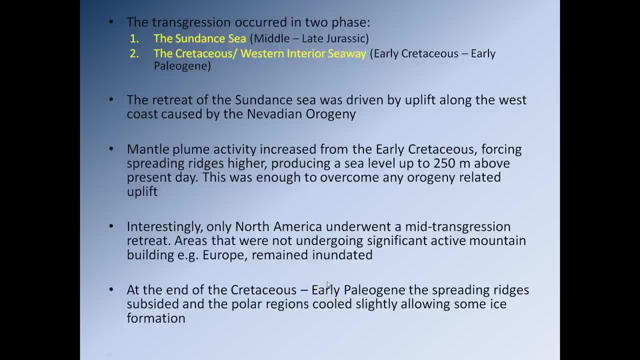 subside as the mantle plume activity beneath them decreases. so that means number one is that as the ridges subside, that means they drop down. that creates empty space and the water flows back into the ocean basins from the land and also as we move from the cretaceous and into 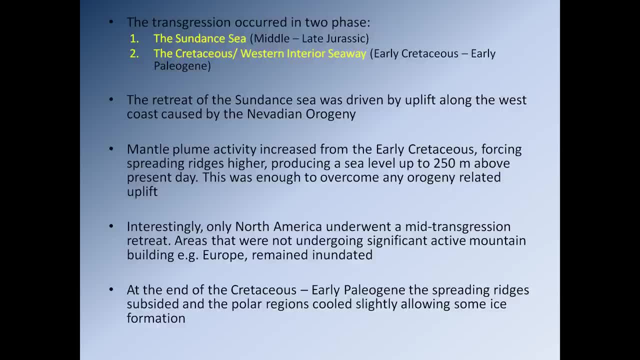 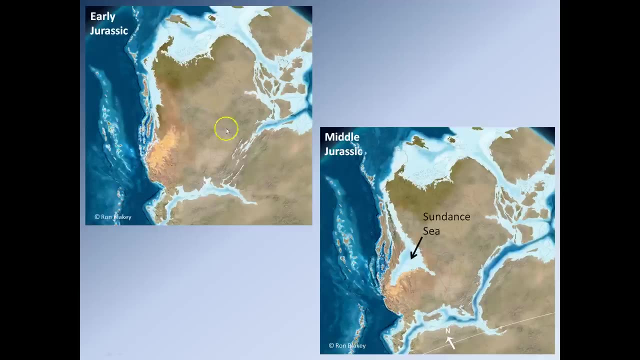 the early cenozoic, we begin to see the formation of ice sheets at the north and south poles, and that's going to start locking up water and that's also going to cause global sea levels to begin to retreat, or should i say decrease, leading to a retreat. okay, so once again here. 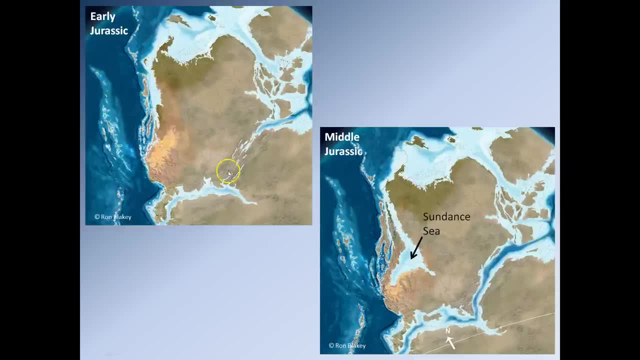 are diagrams. so here's the early jurassic and we can see in the early jurassic of the rift valley what's developing. nicely, you know, we can see we have this early stages of the rockies occurring down here. okay, there's nothing really left of the achiton mobile belt. that's pretty much eroded away. 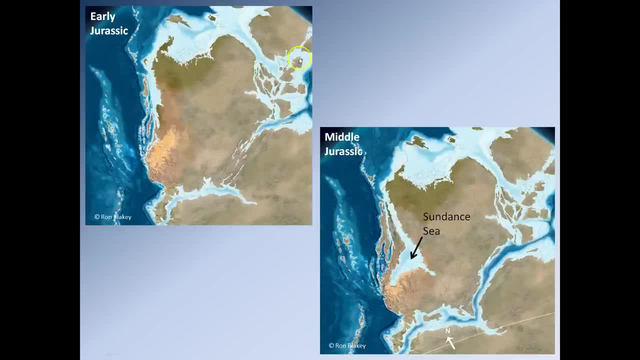 the caledonian mountains pretty much gone, uh, hasinian mountains pretty much eroded away and there's only a little bit left of the appalachian mountains there. you know they're mostly eroded away as well. so essentially we have a fat flat plain here now as we move into the middle jurassic. 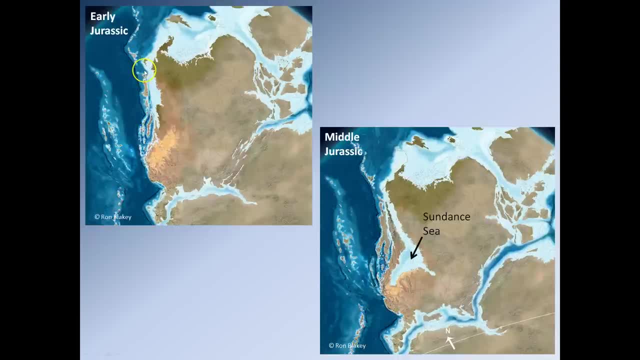 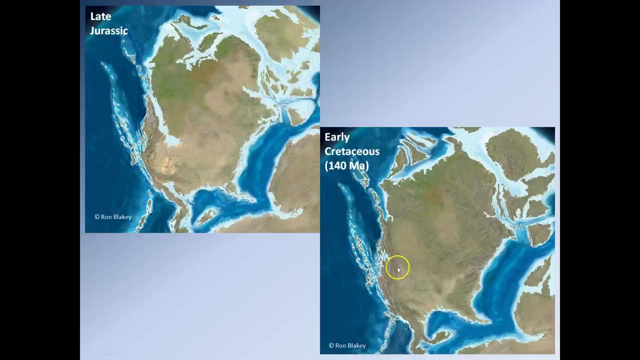 global sea levels begin to rise and we see water begins to move in from this northwestly area here and it starts to move down into the central and western united states, and so this is the sundan sea now, as you move into the late jurassic, you. 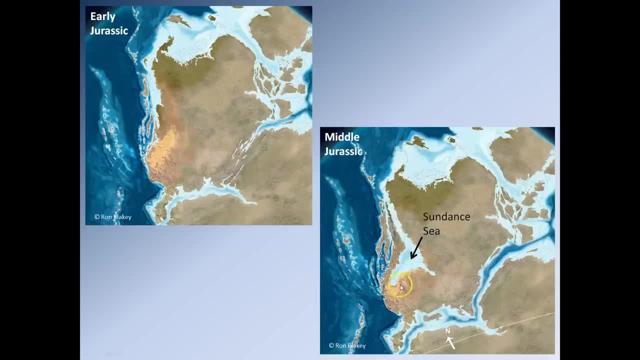 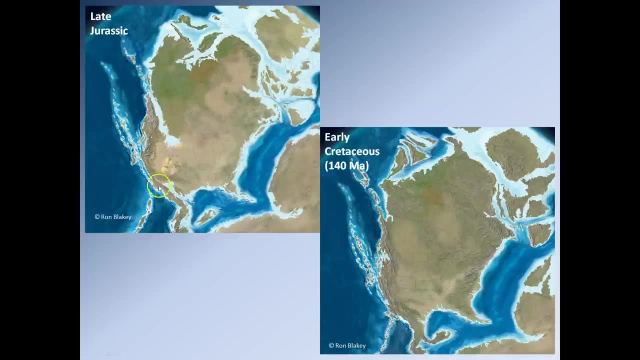 will see that the sundan sea actually goes into retreat. so it's quite large there and by the late jurassic it's actually retreating back into the pacific. that's because the entire west coast is being pushed up as part of the early stages of the formation of the rocky mountains. so obviously, as this area gets, 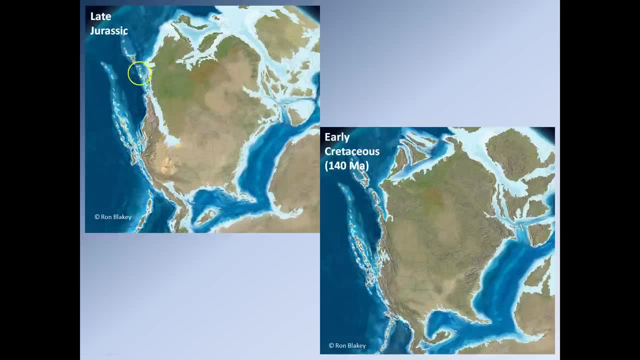 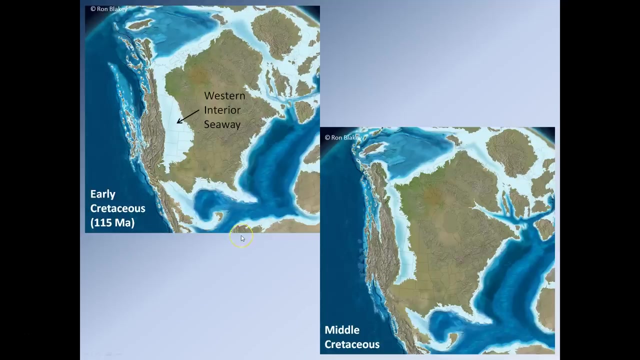 pushed up, well, obviously the water on it starts to drain back out towards the ocean basin, and by the time we're into the early cretaceous, you can see the sundan sea has fully retreated and we have the rocky mountains developing nicely there. now, as you move into the early cretaceous, we then have 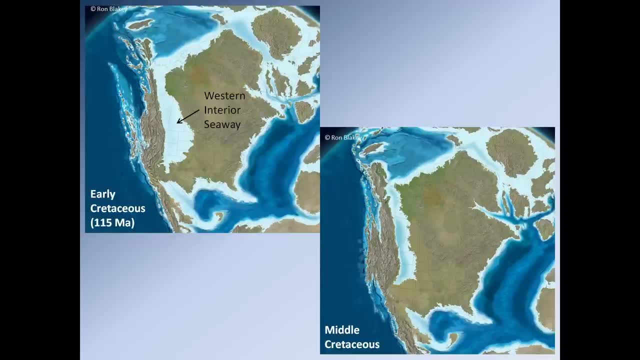 this increase in mantle plume activity and spreading rigidity, and we can see that the ridges, and so these spreading ridges, are getting pushed up, displacing sea water, and that sea water has to go somewhere, so it has to end up moving onto the land, so you'll notice areas like florida. 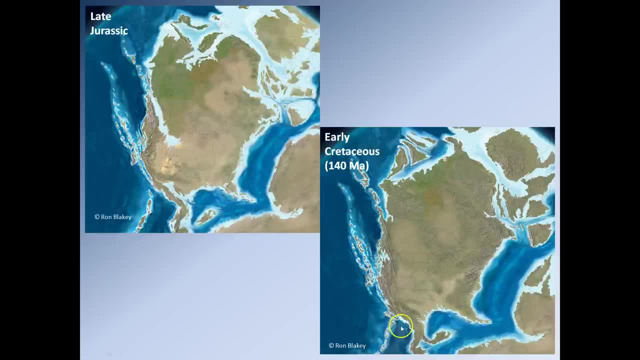 for instance, are thoroughly well above sea level. most of the southern states at this point are well above sea level and obviously this area here is also well above sea level. but what's going to happen is, as the water begins to come in, we're going to see water moving in through here, through. 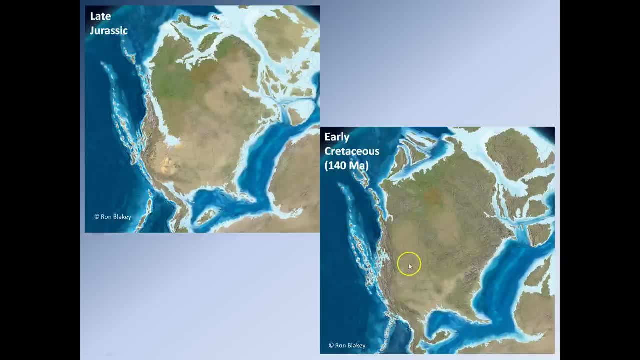 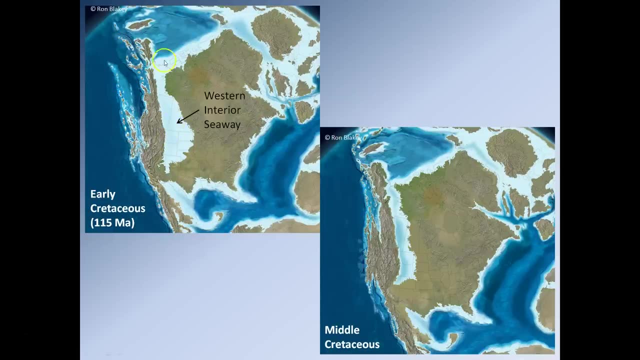 this plain for this region. there's plain here, so water's going to come down here and we're going to see water moving in from here. it's going to come in from the gulf as well, so here we go. so in the early cretaceous the sea level goes up. we see water coming in from the arctic, working its way down the 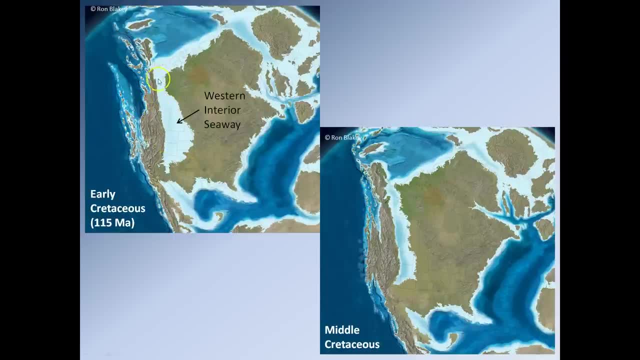 eastern side of the rockies. so the rockies are still above sea level, but the rise in sea level is not is sufficient to overcome the increase in in the western side of north america caused by the formation of the rockies. so we can see the water begins to come down along the eastern side. 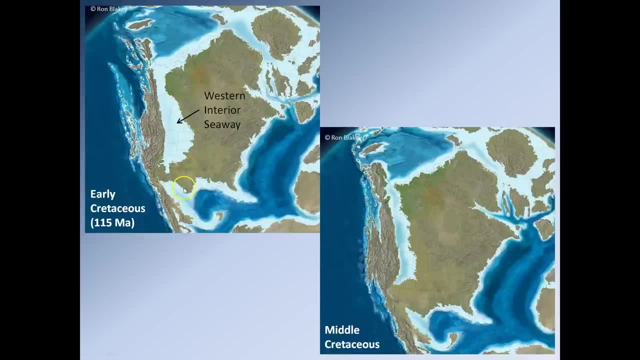 of the rockies. it also begins to move northwards from the eastern side of the rockies. so we can also see that. well, we can see, by the middle cretaceous there's a slight retreat going on. as we move into the late cretaceous there's a real burst of activity. in this point we can see. 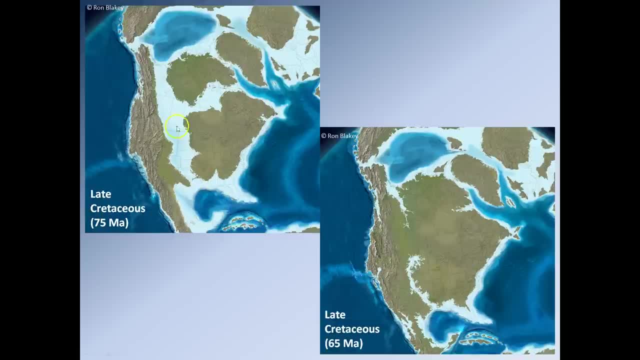 we now have a body of water that goes all the way from the arctic all the way down to the gulf of mexico. we also have the formation of another branch over here that goes from essentially alberta and saskatchewan over here- sorry, we're saying alberta and manitoba- and goes all the way. 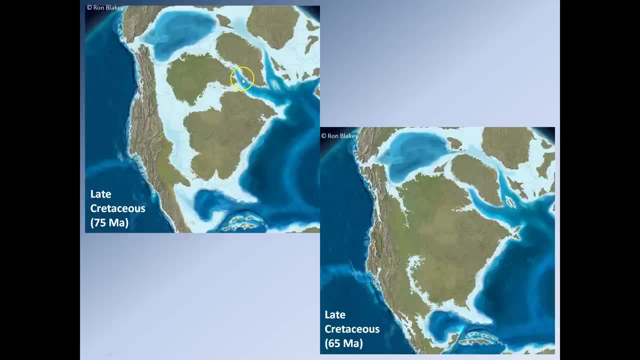 through to essentially the coast you know around newfoundland, greenland, that kind of area essentially along the what is now the modern day st lawrence skive will take a little bit and then you can see as we move from the late cretaceous into the nearly the essentially the cretaceous tertiary. 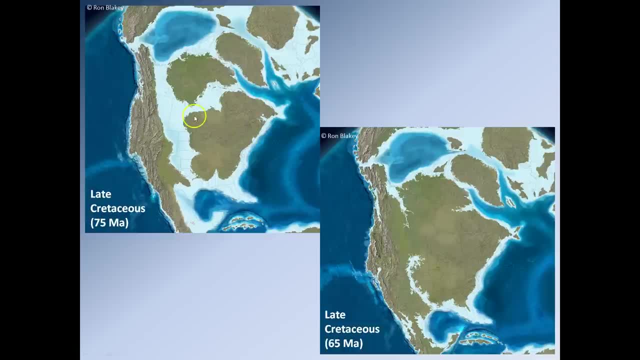 boundary. we can see that the zunia pyrexia is in full retreat. so it's retreating out towards north atlantic, out towards the arctic and back towards the gulf of mexico. so that's the zunia pyrexia. you can see that essentially, even at its maximum extent, there were still large quantities. 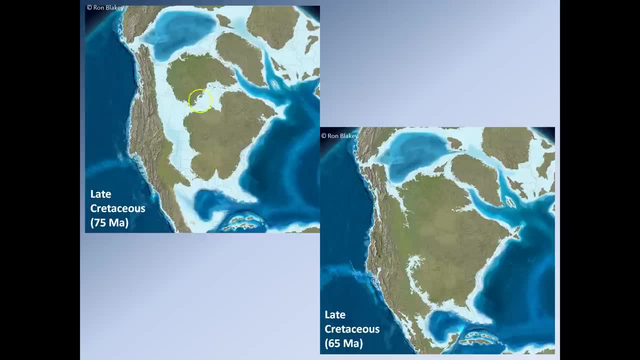 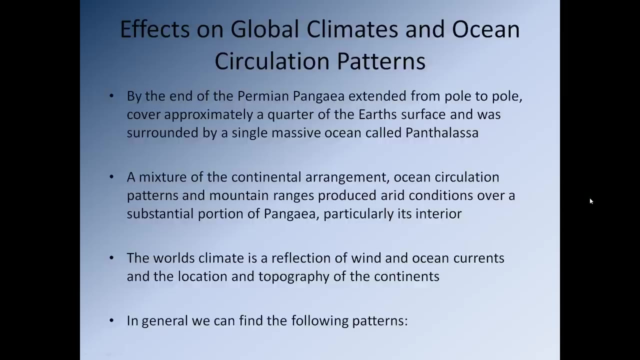 of continental north america exposed above sea level, and that means these seas would have been absolutely stuffed with clastic sediment coming off, coming, you know, being formed from the erosion of these areas of continental crust. so good, this is a actually quite a good time to pause for a second. so 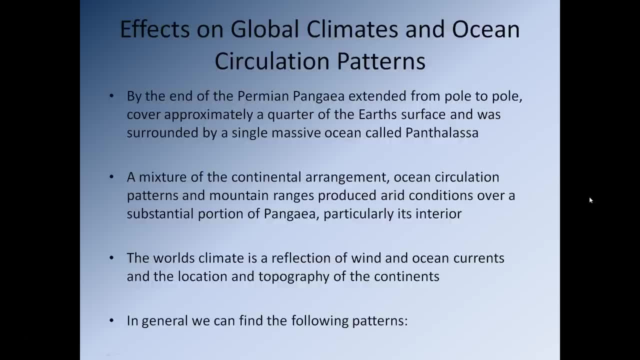 pause presentation: get up, have a walk around, get a glass of tea, of water, and please come back in a couple of minutes. so, as we've been going through the um, through the paleozerk, into the meser, one of the things that's been near consistent is the fact that, when it comes down to it, we've only really had 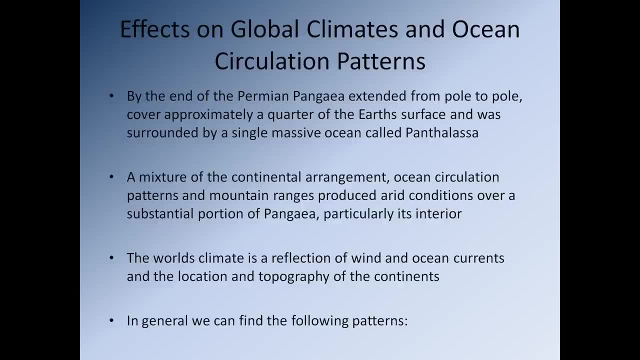 you know, two, one, two or three major land masses, and so this has meant that the oceans could circulate rather freely. now, when an ocean can circulate rather freely, that means warm water free, and then, when it comes down to it, we've only really had two, one, two or three major land. 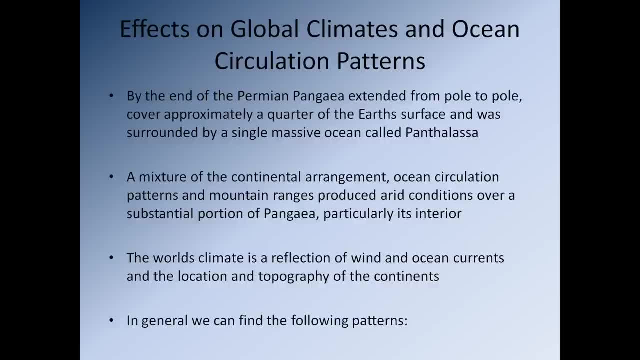 masses from the equator can move northwards or southwards towards the poles relatively easily and relatively quickly, and so this means that that warm water helps to keep these, uh, these higher latitude regions artificially warm. so a classic example of that now is the united kingdom. so the united kingdom is kept warm, uh, by the gulf stream, and that's a river of water that goes from. 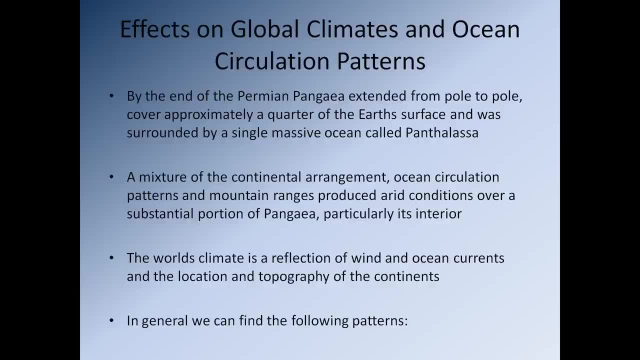 the uh, the caribbean sea and it goes all the way across the north atlantic and it makes you know it hits essentially the area around the united kingdom and ireland and it helps to keep the water around the united kingdom artificially warm. so one of the things you probably know about. 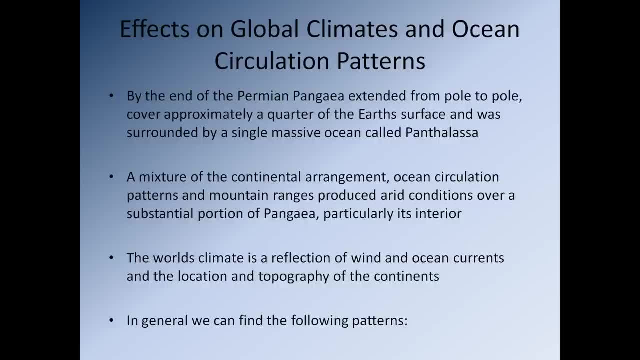 the united kingdom is that it's an extraordinarily wet country. you know it has heavy rain, at least, you know, 100 days out. you know, in the year the rest of the time is normally great. i should know, i live there. um now, one of the things that people don't realize about the united kingdom, though, is it is 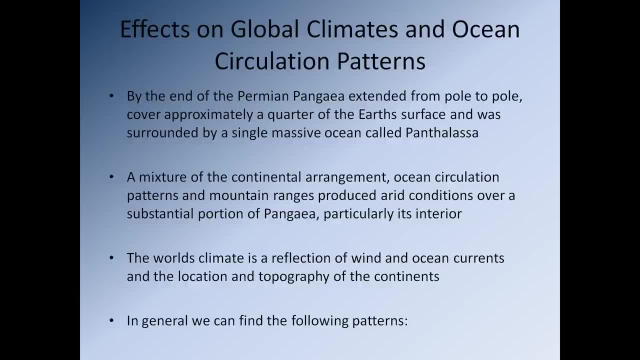 actually on the same latitude as moscow. however, the united kingdom is not known for its particular, particularly cold winters. Moscow, on the other hand, if you've ever been there in the winter, you will know it has very significant snowfall and temperatures can get down into the minus 30. 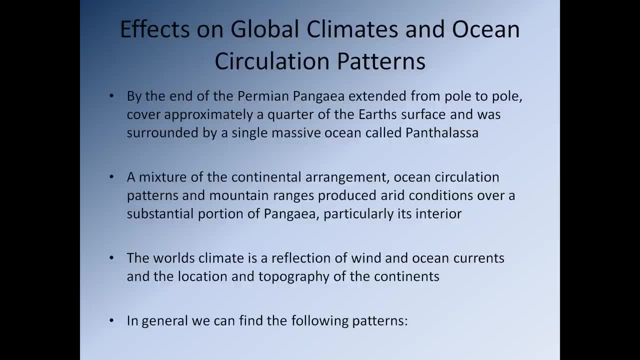 kind of range. So what's making the difference? Well, the answer is the Gulf Stream. That river of warm water coming across the North Atlantic, helps to keep the United Kingdom artificially warm, And so it means that the winters are nowhere near as harsh as they could. 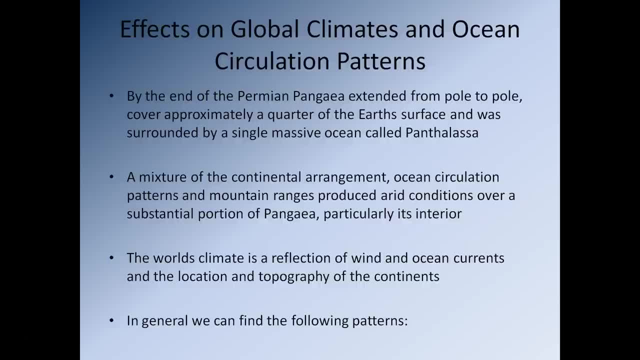 be So. it helps to keep the climate more stable, And that's exactly what was going on all the way through the Paleozoic. You had all this warm water coming from the equator going towards the higher latitudes, helping to keep the temperature up in those areas, nice and stable. 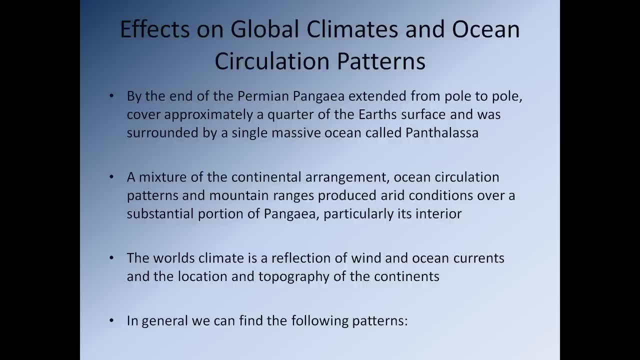 Now, what's going to happen as we move through the Mesozoic is, as you've seen, all the continents begin to break off from one another. We end up with all the modern continents all moving towards their current positions. Now this is obviously going to affect how the water in the ocean 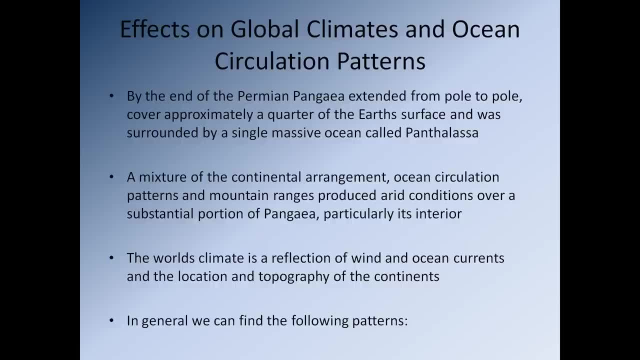 circulates And how the water in the ocean circulates is going to have a direct impact on the climate And that's going to affect how the water in the ocean circulates And that's going to have a direct impact on the climate And that's going to have a 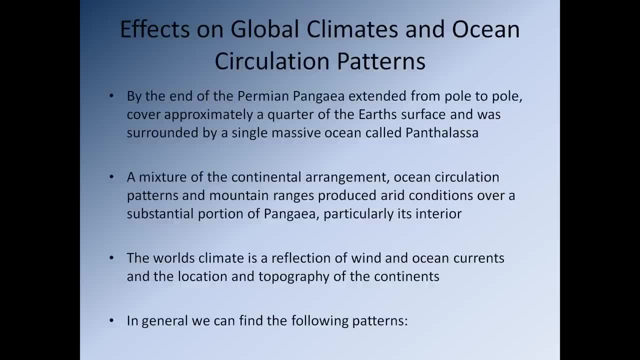 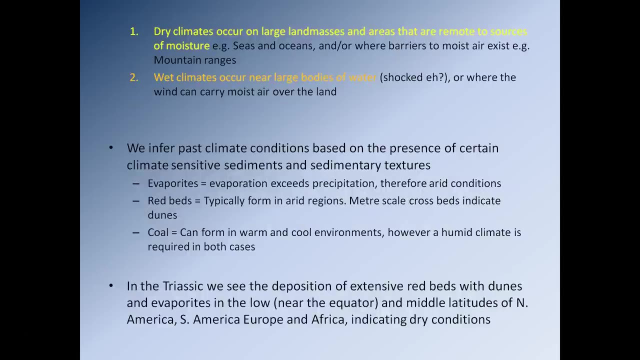 direct effect on how the air in the atmosphere moves. That's going to affect wind directions. That's then going to affect essentially the global distribution of certain climatic bands. So the general trends that we see is we tend to get areas with dry climates that will occur on large landmasses and areas that are remote to. 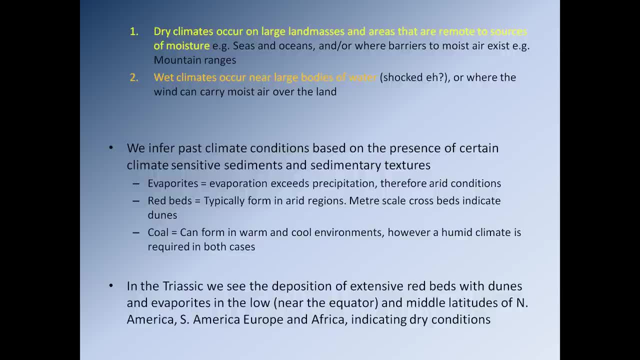 sources of moisture. So the further you are from a sea or an ocean, typically the drier your climate will be, And once again, the classic example of that is Asia. So if you ever look at a Google Earth image of Asia, what you'll notice is the center of Asia, the kind of Mongolia. 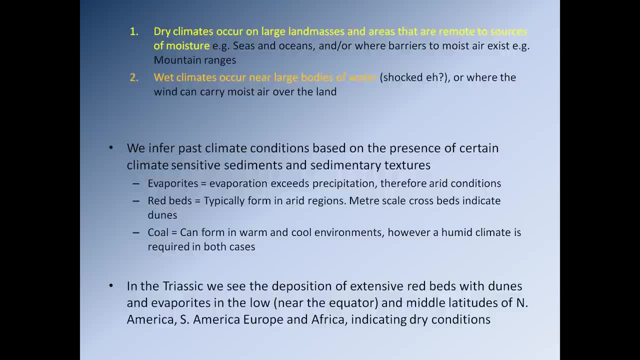 Western China, Tibetan Plateau into Kazakhstan, Tajikistan, areas like that. That area is, on the whole, either desert or semi desert, because it has a relatively low yearly rainfall. On the other hand, areas that tend to have relatively high rainfalls, which 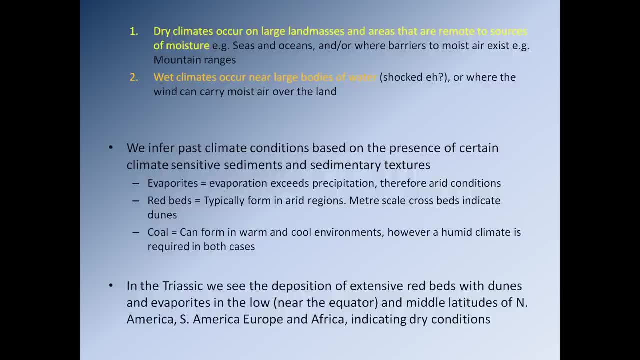 will often be situated near large bodies of water, typically towards the coast. And so, once again, if you ever look at- you know, a Google Earth image and just zoom out of the earth, what you'll know, zoom out and look at the earth as a whole, what you'll notice is the 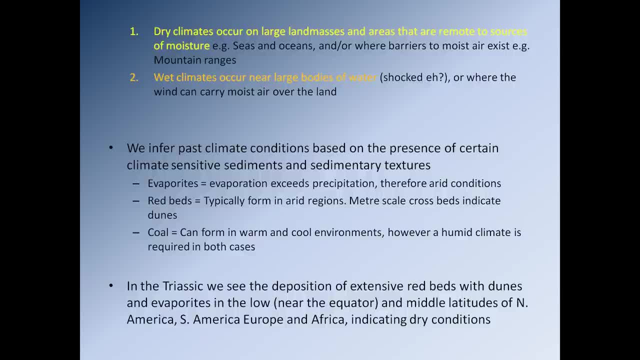 vast majority of the greenest areas are located- shock horror- near the coast. So we know that these general trends exist so that we can make very broad predictions based on those two trends relatively easily. So you know, we know, for instance, that through the Mesozoic you know the land mass that is Asia. So if we just 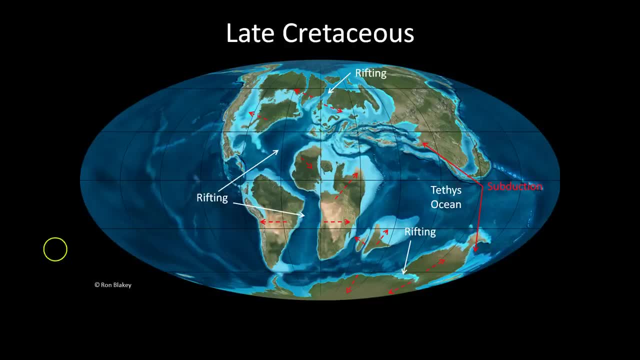 zoom back here, go back a few slides for this one. So we know that during the Mesozoic, we know that this large land mass here which is, you know, modern day Asia, we know the core it's going to be quite dry, And so we can say, right, we'll have, you know, arid or semi-arid conditions here. 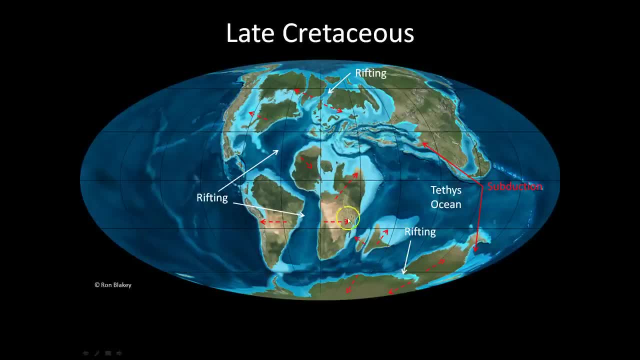 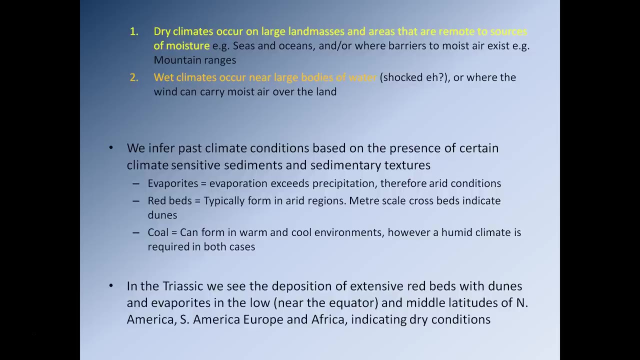 you know, whereas we know that these areas around here that are close to the coast, Well, we can say relative certainty that these areas are, on the whole, going to be quite wet and therefore, you know, quite heavily wet vegetated. so you know, we can make those broad assumptions straight away. so what else is going? 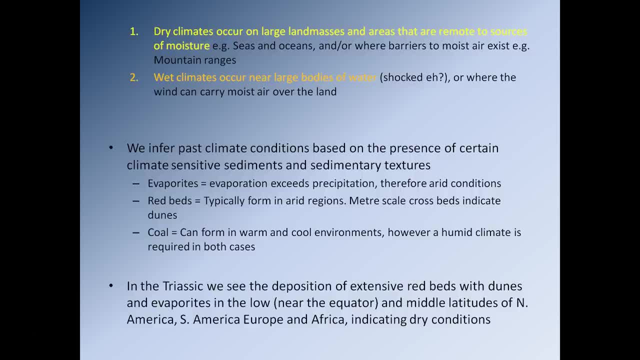 to give us hints about the past climate. well, as we've discussed in the past, there are certain sediments and certain you know things that we see in sediments that allow us to infer environments. these are: these are sediments that are essentially sensitive to climatic effects. 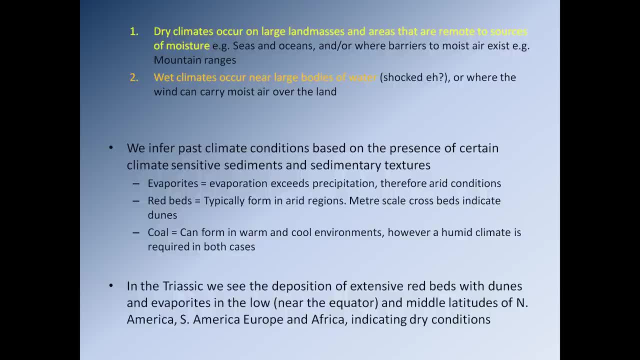 so one of the classic examples of that is evaporites. so if you want to form layers of evaporites, obviously you need an arid to semi-arid climate, okay, so whenever we find layers of evaporites in meseric rocks, well, clearly we know that during that time period. 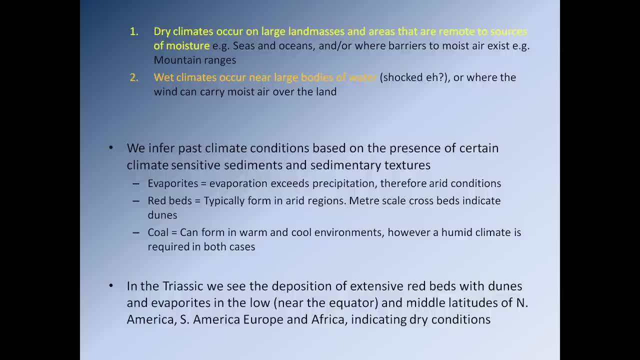 that area must have been relatively dry. same goes for red beds. so when we find sandstones that have that distinct rusty red color to them, well, once again we know that essentially those rocks must have formed, or should i say are very likely to have formed, in a hot, arid or semi-arid. 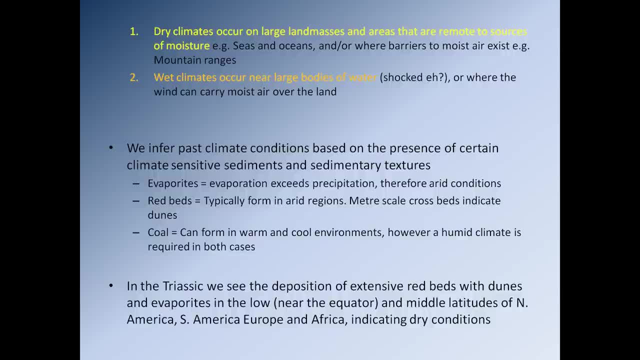 climate and then we have rocks like coal. obviously coal likes to form in warm, humid, swampy environments. so, once again, when we find layers of coal in meseric rocks, we can say that during the meseric that area was essentially warm and swampy, and there's actually one that i missed off the. 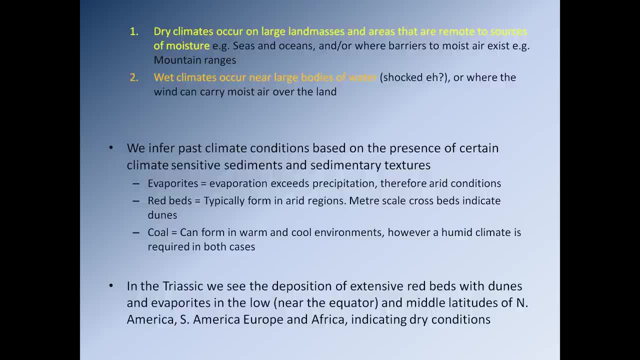 list there. the other one is, of course, limestones. limestones like to form in warm, shallow seas, and so, once again, if you find limestones, you know, chances are you were dealing with an area of the sea that was warm and shallow. okay, so the triassic sees the deposition of extensive red beds with with cross beds in them. 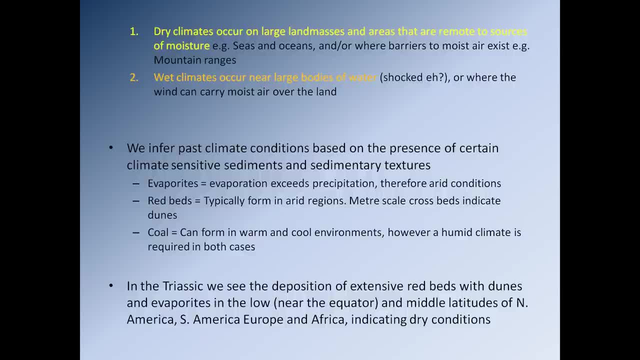 so we know there were dunes, there are lots of evaporites around, and so that clearly indicates that there were dry conditions in north america, south america, europe and africa. and that makes perfect sense, because at this point in time pangaea is nearly still complete, so we have one. 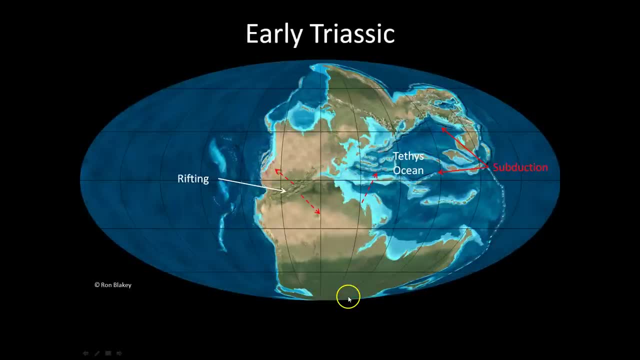 huge landmass. so if we go all the way back- sorry about this- so if we go all the way back to the early triassic, you can see that these huge landmasses are all the way back to the early triassic because these areas that are well away from the oceans are going to be very, very hot. 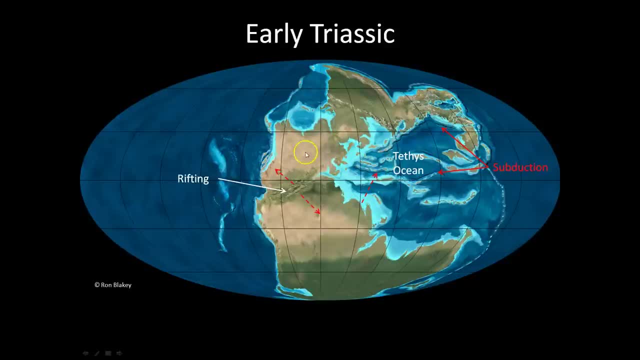 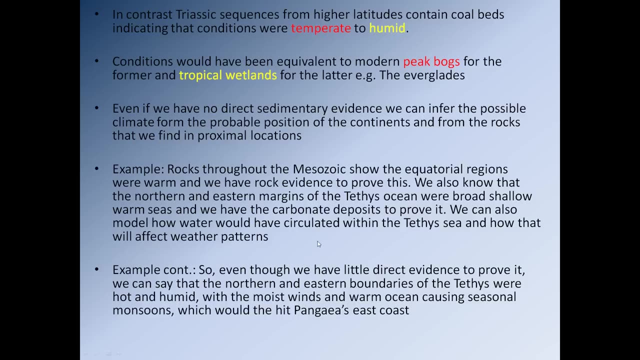 very, very dry, and so we're going to have huge areas of desert in these regions, here especially, okay. so, in contrast, triassic sequences from higher latitude areas, so that's more towards the poles, tend to contain coal beds. so that would indicate that as we moved towards the poles during the 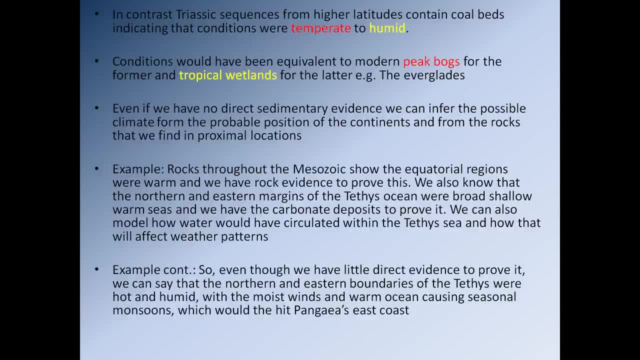 triassic temperatures dropped a little bit, and so we're going to have huge areas of desert in these regions. so that's more towards the poles. during the triassic, temperatures dropped a little bit, or at least the amount of humidity increased, and so we ended up with environments where having you. 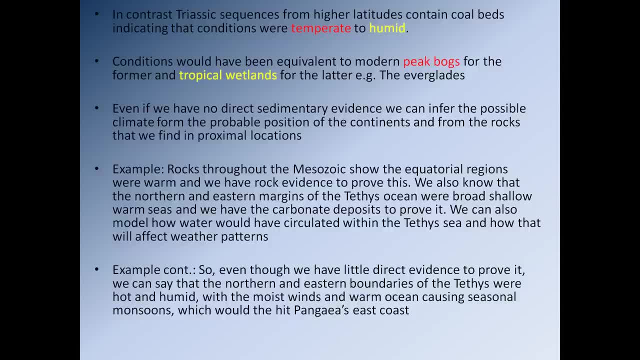 know, having temperate, swampy environments in which we could form large quantities of organic material became possible, and then therefore we had coal swamps. so today conditions would have been equivalent probably to modern day peat bogs or, in some cases, tropical wetlands. so, depending on 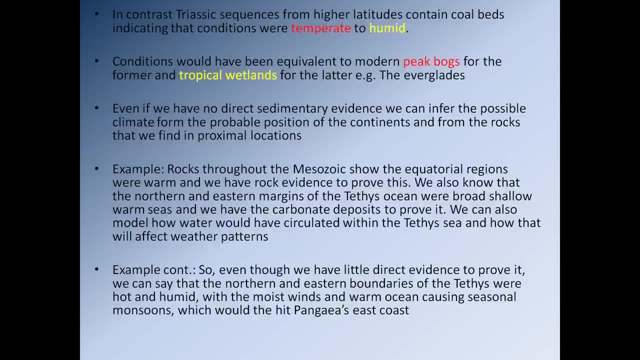 exactly how hot the climate was, you would have formed- uh, you know- build up of a lot of organic material that would have either been like peat, which is the kind of you know thing you could expect in places like ireland and scandinavia, so much lower temperatures, or in areas that would 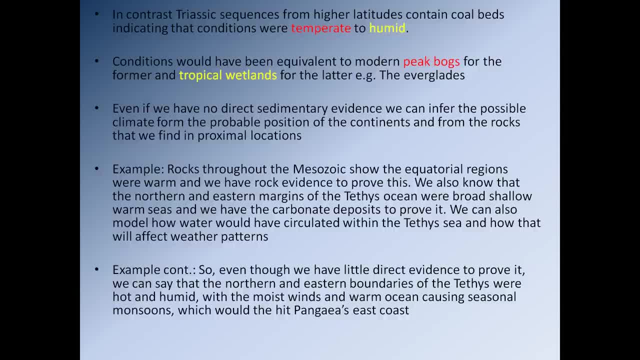 have been warmer, you would have expected more tropical wetlands to form, you know, kind of equivalent to the florida everglades, for instance. so in some cases we can make relatively strong inferences about the type of environment an area was uh under during the mesozoic. however, there 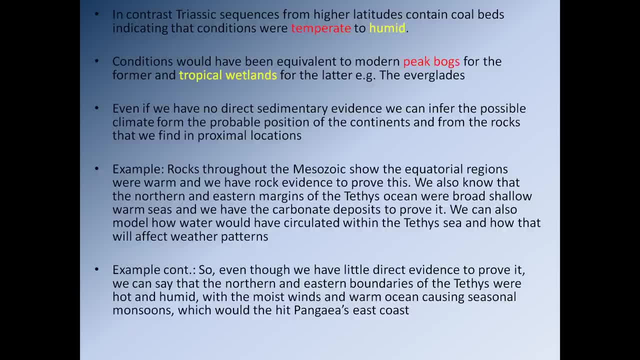 are some other examples of the type of environment an area was under during the mesozoic. however, there are some other examples of the type of environment an area was under during the mesozoic. however, there are some areas where we just don't have that evidence, and so you know the rocks there are. 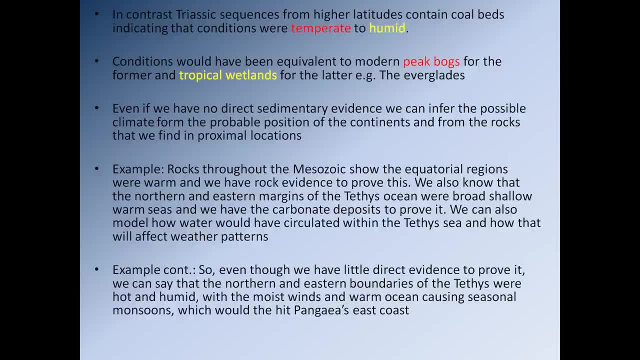 maybe pretty generic, and so we can't really draw many conclusions from them, and so what we have to do is we have to start inferring the probable climate based on some, you know, logical hypotheses and evidence from other proximal locations where we do have evidence about the climate. so a good. 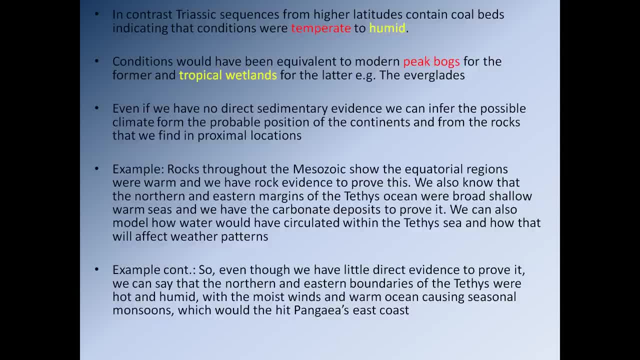 example is that rocks throughout the mesozoic show, the show. the equatorial regions were warmer and we have evidence, uh, to prove this. so sorry, i'm going to start that sentence again because i completely lost my train of thought. i do apologize. so yeah, rocks throughout the mesozoic show, the 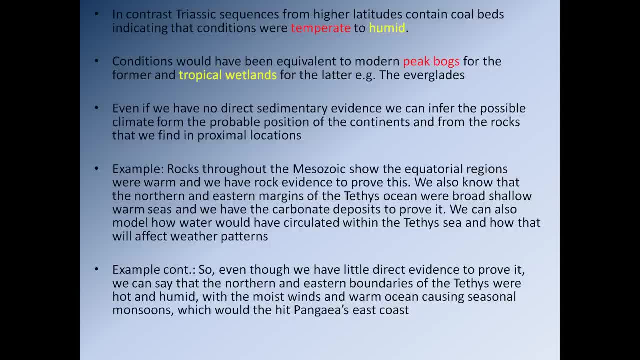 equatorial regions were warmer and we have evidence to prove this. so we have, you know, lots of desert sediments. so we know that the equatorial regions during the mesozoic were on the whole, you know, quite dry. we also know that the northern and eastern 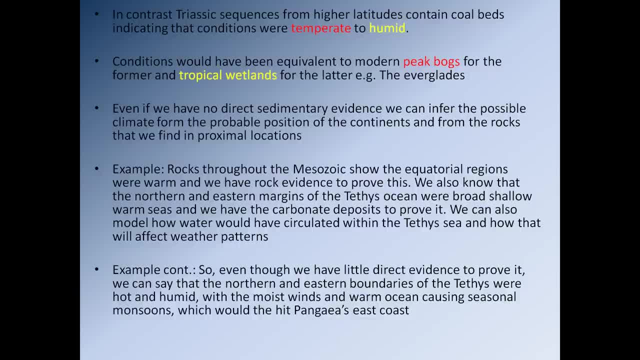 margins of the teffy's ocean were broad, shallow, warm seas and we have the carbonate deposits to prove that. so we can model how water would have circulated around the teffy's ocean and how it will affect weather patterns. so once again, if i just go all the way back up here, 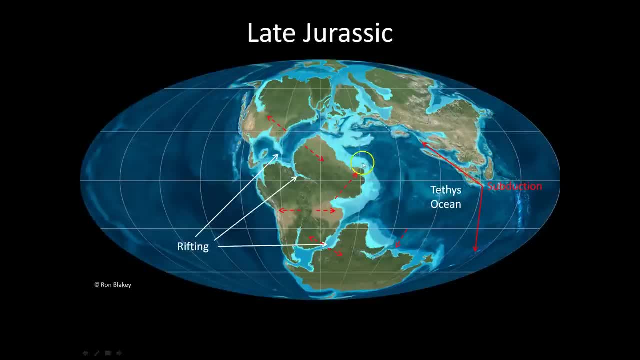 well, we know that the northern portions of the teffy's ocean and the eastern portions here, well they were limestone producing factories. so we know that these areas here would actually would be marine, warm shallow water and we know that during the mesozoic the entire equatorial region 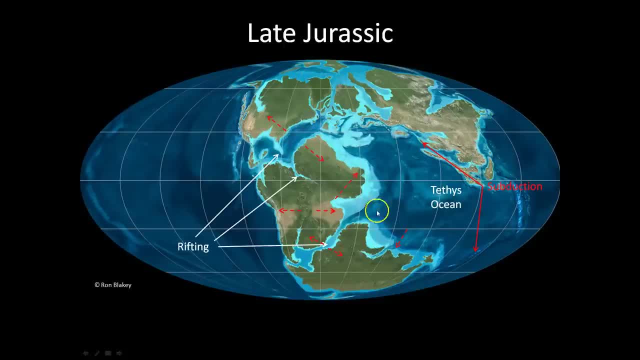 was nice and warm, just below 30 degrees celsius, like it is now, so we can make inferences about how the water would have been circulating around in the teffy's ocean. now, once we know how the water's moving around the teffy's ocean, 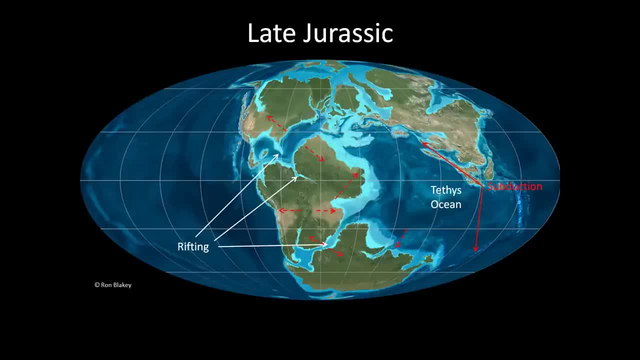 that then means we can make predictions about the how the air was moving in the atmosphere, and so that's going to allow us to essentially work out what the likely weather patterns would have been, you know, in this area of the teffy's ocean during the mesozoic. so even if we don't, 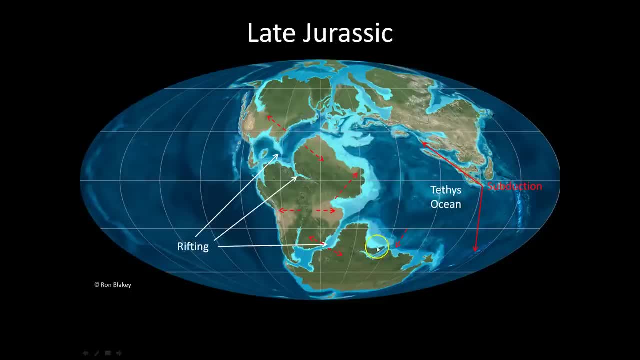 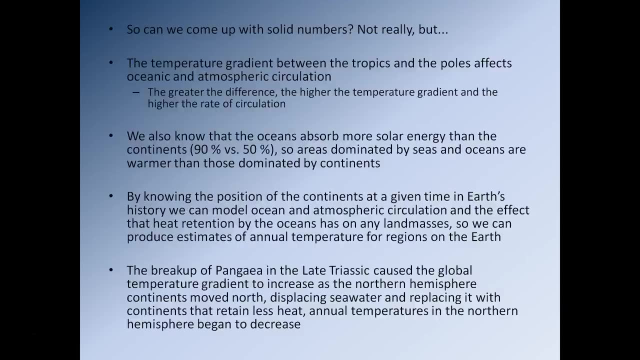 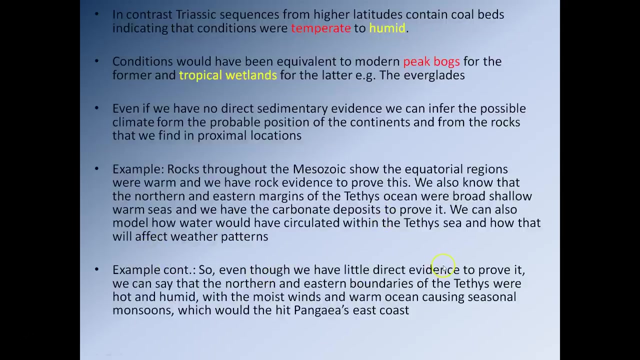 have evidence for you know, let's say, what the climate was like here. based on our modeling, we can make a very educated guess. so if we continue our example, so even though we have little direct evidence to prove it, we can say that the northern and eastern boundaries of the teffy's ocean 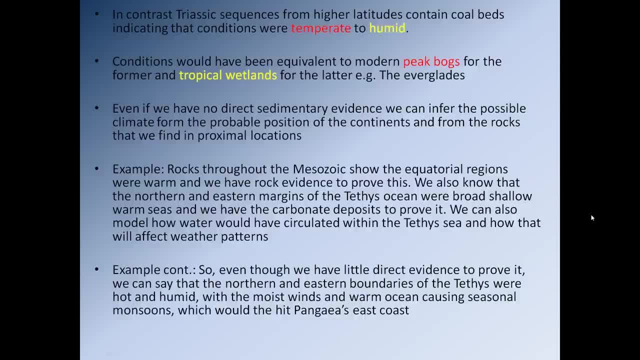 were hot and humid. so we don't really have the rocks to show what they what the conditions were like there, but we know that the continental rocks in that area were probably hot and humid and, based on our modeling of the weather patterns, we can say that there would have been moist winds. 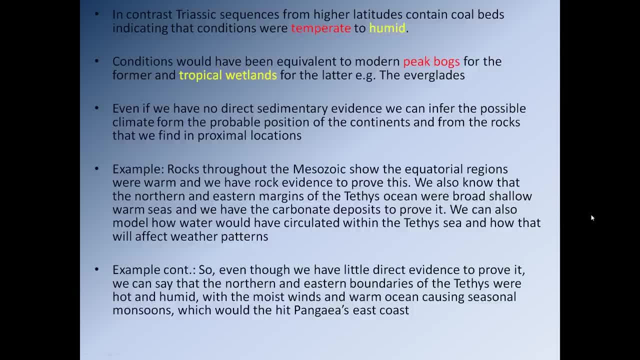 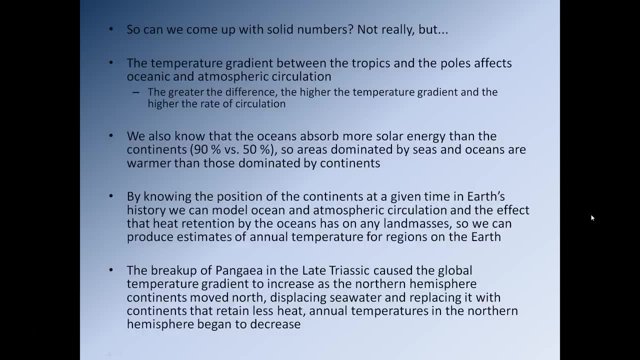 coming off the teffy's ocean, and that would, of course, seasonal monsoon, so conditions would have been a lot like modern day southeast asia now. so next question is: when it comes to discussing past climates, can we come up with solid numbers? the answer is no, we can't. so the temperature gradient between the tropics and the poles. 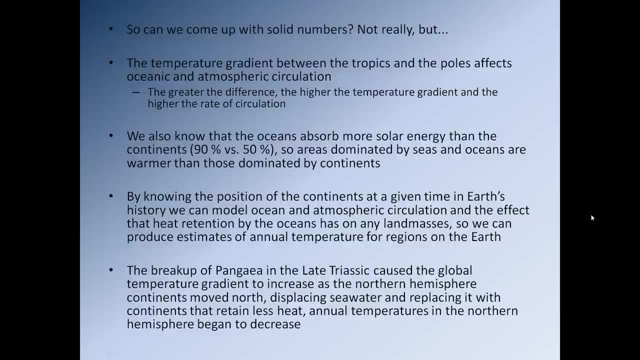 affects oceanic and atmospheric circulation. so the greater the difference between the poles and the equator, the higher the temperature gradient, the higher the temperature gradient and the higher the rate of circulation. so if the poles are very, very cold and the equator is very, very warm, the water that's circulating between the two will go very, very quickly. 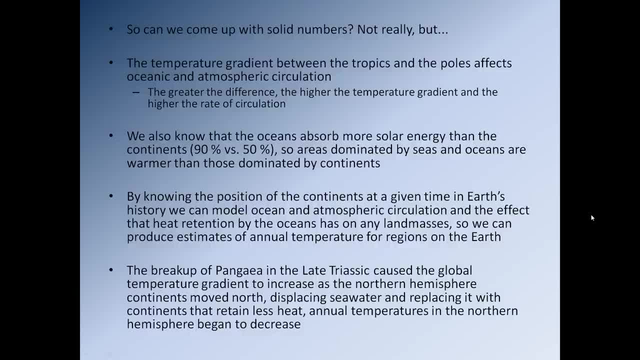 what we also know is we know the oceans will absorb more solar energy than the continent. so sea water will absorb about 90 percent of the solar energy that hits it, whilst the continental crust will only absorb somewhere in the region of 50. so, essentially, the seas are much more efficient. 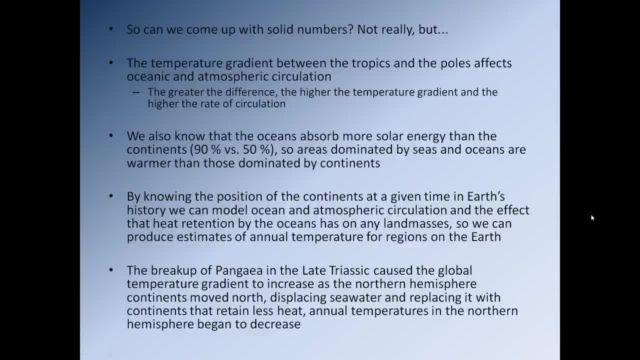 at absorbing sunlight. so that means we can say areas dominated by the oceans are clearly going to be warmer than those that are dominated by continental crust. so by knowing the position of the continents at a given time we can model ocean and atmospheric circulation and the effect of heat. 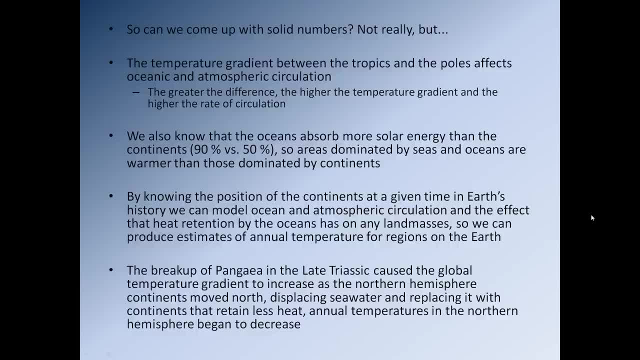 retention by the oceans and the land masses. so we can produce estimates of annual temperature for regions on the earth's surface. so you know, just through some relatively basic assumptions, based on you know, what we know from the modern environment, we can come up with broad assessments of what annual temperature would have been like, you know, in certain, on certain parts of the earth. 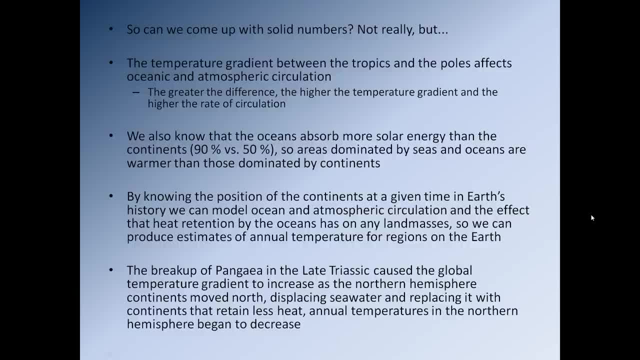 during. you know the meteoric. so what we notice is the breakup of pangea in the late triassic caused the global temperature gradient to increase significantly. so why is this? well, during the late trassic we begin to see the northern hemisphere continents move north, so north. 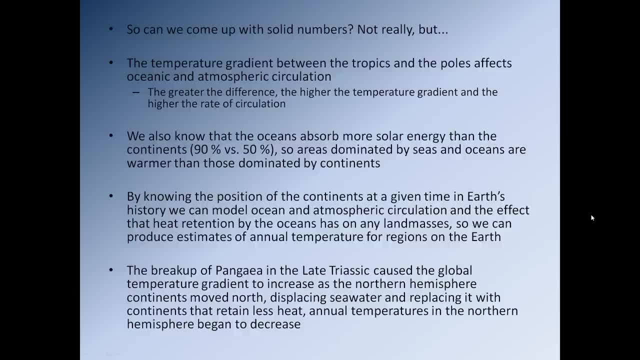 europe and asia start moving towards the north pole. now, as they start moving towards the north pole, what that does is it displaces sea water. remember: sea water is really really good at retaining heat. continental crust is nowhere near as good. so as north america, europe and asia move, 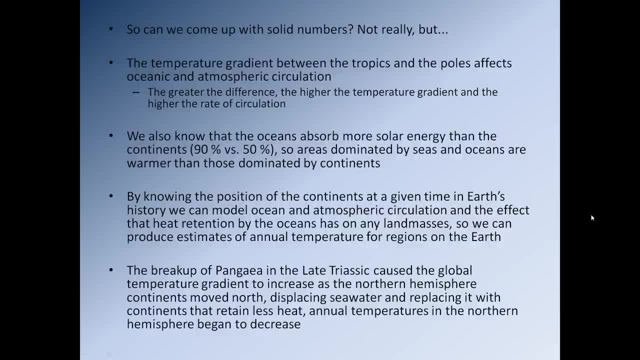 northwards. well, the northern hemisphere, or at least the higher latitude portion of the northern hemisphere, starts getting colder because there's less sea water up there to retain heat, and so we begin to see a shift in the sediments. and we begin to see a shift in the sediment. so we begin to see. 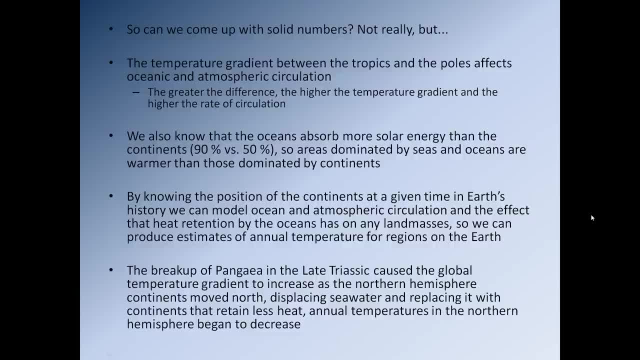 this in north america, europe and asia, throughout the cretaceous especially. we begin to see this shift from relatively warm weather sediments into colder, more temperate weather sediments. we can also begin to see this. we can also begin to see that there may be some. 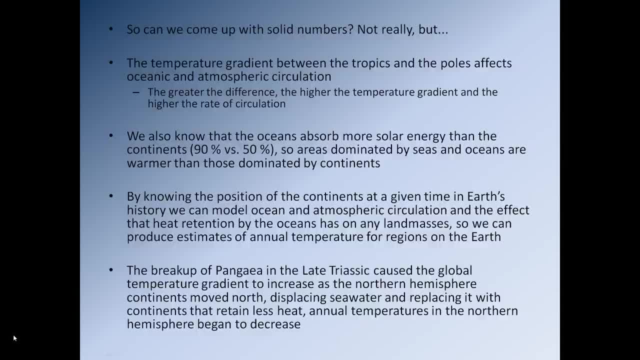 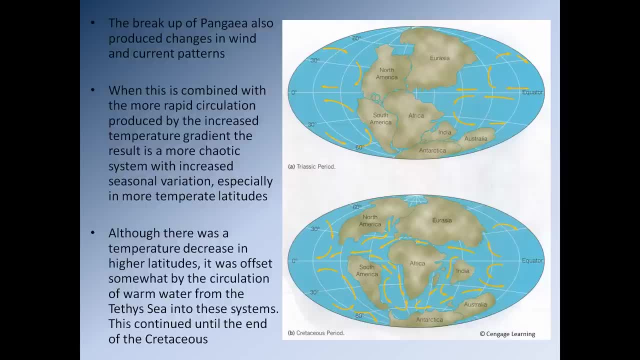 seasonal variation beginning to appear as well, you know, start getting cold winters and warm summers. so when changes in ocean circulation occur, it also has an effect on the atmosphere. so as pangaea breaks up, it's also going to change how the atmosphere circulates and therefore how. 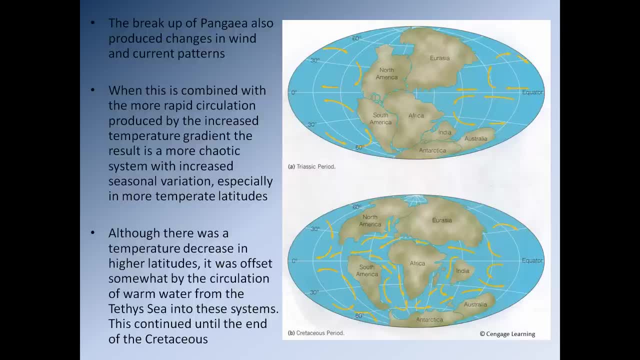 the winds in the atmosphere move. so when we combine this data on how the air in the atmosphere starts moving, or these changes how it moves, and the combination of this more rapid ocean circulation, we begin to be able to come up with, you know, a relatively good model of how the climate. 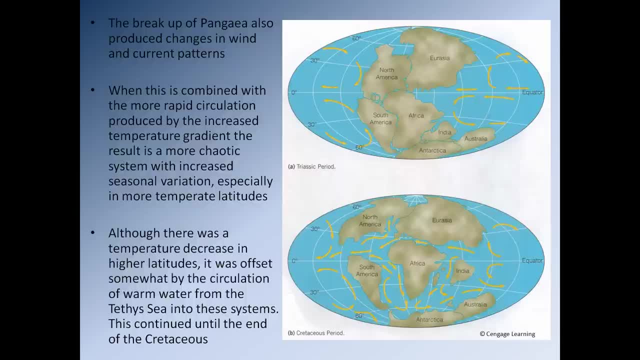 began to change through the mesozoic, and so what we see is especially in the cretaceous: as the continents begin to separate from one another fully, we begin to see that ocean circulation becomes far more chaotic. we begin to see that. well, we can see it here. so 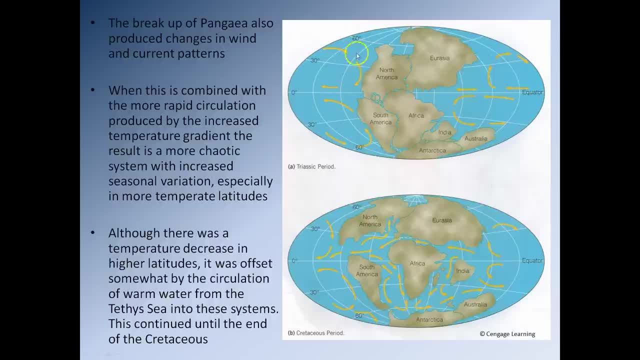 here's pangaea we can see the ocean is circulating freely. therefore we have good homogenization between the equator and higher latitudes. as we move into the cretaceous, we see north america and europe and asia pushing north, replacing warm sea water up here with cold continental crust. 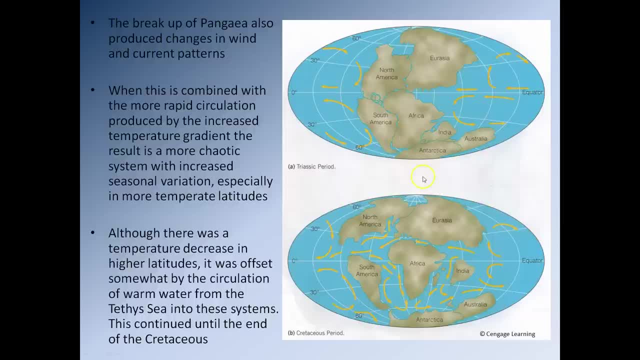 so the northern hemisphere starts to get colder. we can see that antarctica starts to move fully over the south pole, so we're going to get large scale glaciation forming there, which is going to help to cool down at least the area around the south pole. and we can also see these nice open circulation, this nice open circulation of 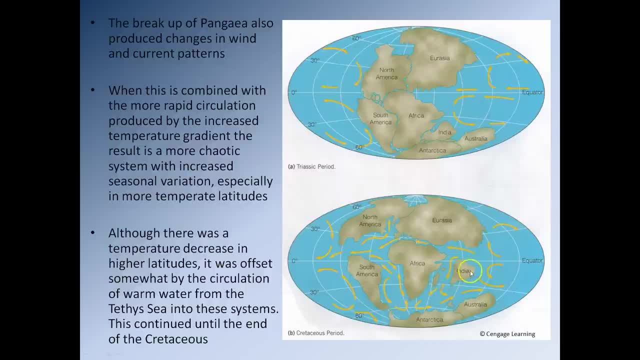 sea water begins to get completely destroyed. as all the continents start to move in their own directions, we start to get very localized circulations of water. this is all going to affect how you know the sea, how the seas circulate, also how the atmosphere circulates, and so what we know is, as we move into the mesirc, especially the 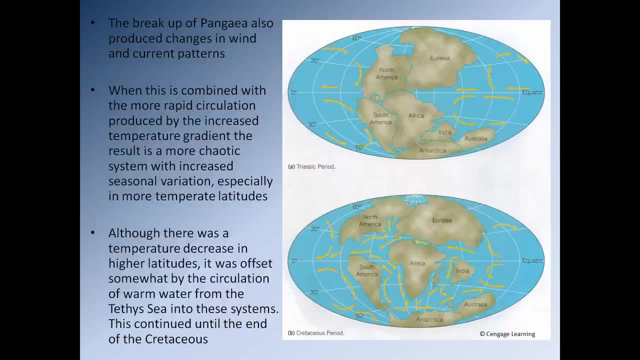 cretaceous. we begin to see a significant change in global temperature, so we begin to see the poles get colder. we also begin to see the temperate band begins to move south. that means the equator starts to get squished, so the equatorial region starts to get a little bit compressed. 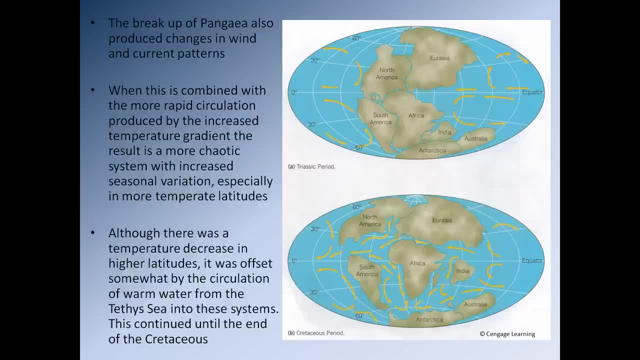 and we begin to see far more chaotic weather, and by chaotic weather what we really mean is seasons- begin to see evidence that in the northern hemisphere, you know, we start having a winter, we start having a summer. same goes for the southern hemisphere continents. so all of a sudden, 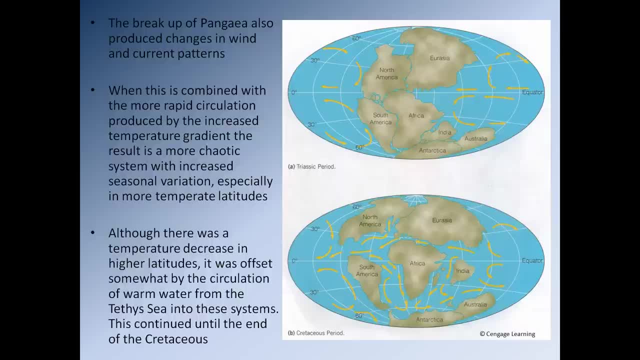 if you're a reptile like a dinosaur and you really really love it when you have constant hot conditions. well, all of a sudden, if you're living in north america and you know from from november all the way through to march, all of a sudden the temperatures are getting pretty darn low. 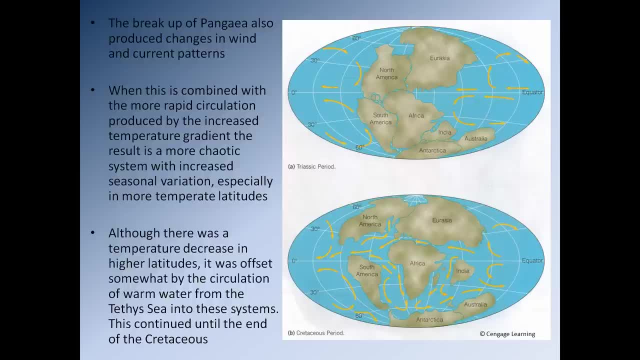 well, you're going to be in a lot of trouble. and so this breakup of pangaea is one of the reasons that the population of dinosaurs starts to become stressed, because all of a sudden, you have dinosaurs that like living in these. you know relatively warm, relatively dry conditions and all of a sudden, 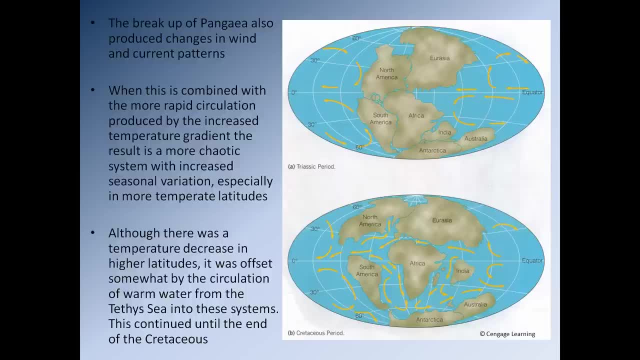 they're finding that their, their climate is becoming, you know, colder, especially for part of the year, and maybe in some areas it's typically becoming a lot wetter and a lot cloudier, so that means less sunshine. So that's obviously going to start stressing the dinosaur population quite severely. 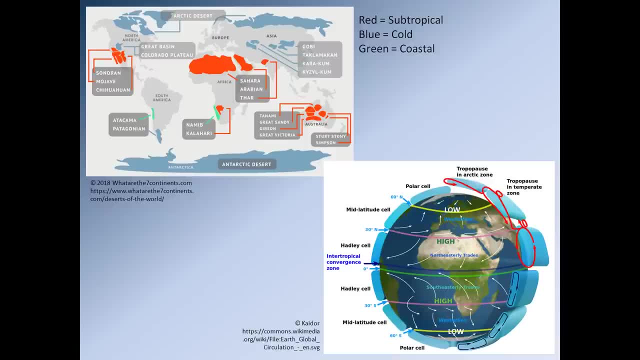 it also means that air circulation is going to move more towards the modern pattern. so if we look at this diagram down here, it shows you how air moves in the modern environment. so let's have a look at the globe. so what you'll notice is: here's the equator, this dark blue line here. 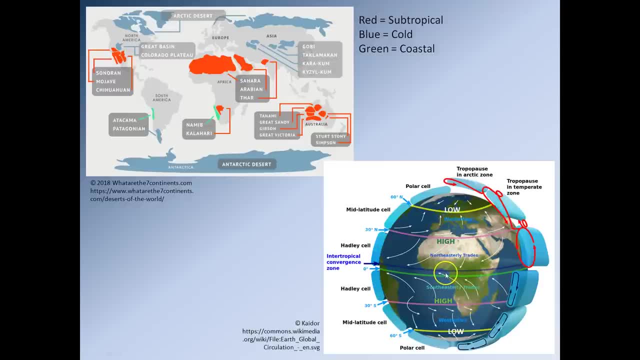 you'll notice that air moves towards the equator, and you also notice that air moves away from this pink line towards this low pressure line here at about 60 degrees north. okay, so what this means is is air gets pulled away from this band here about 30 degrees north and south of the equator. so what this means is all the air gets pulled away. 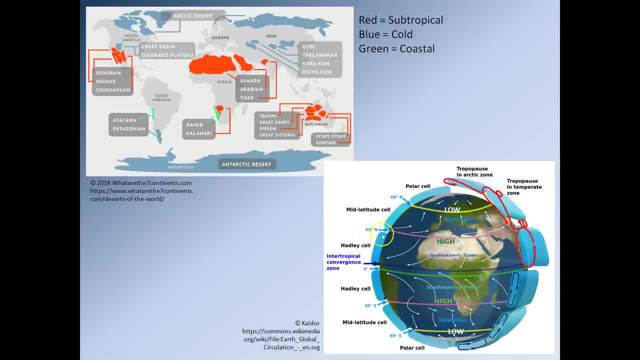 from here to the left of a band essentially of relatively dry air in this area, and you'll notice that when we look at where the deserts are located, there's the 30 degree band there north and here's the southerly 30 degree band. here. 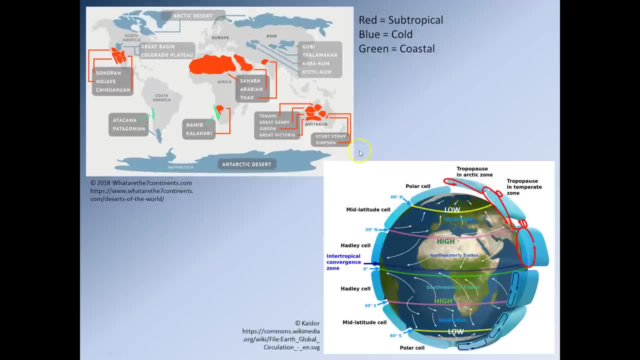 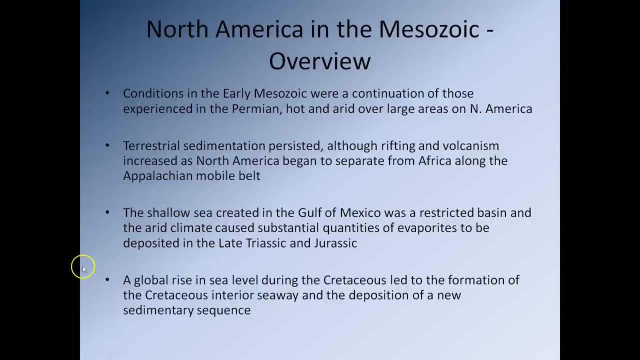 So what this eventually ends up causing is it ends up causing, essentially, the atmosphere to begin to separate into these distinct bands, and we end up setting up the kind of climatic zones that we have now. Okay, so we've been going for an hour again, so this would be a good time for a break. 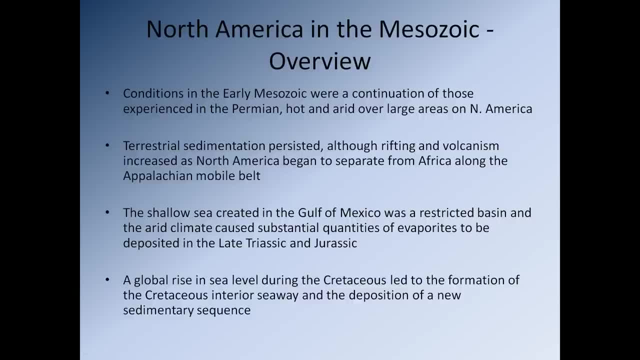 but before you go, let's do today's code word. So today's code word is Beowulf. Yeah, do you know what that is? I'm sure some of you might, some of you might not. so Beowulf is a famous Anglo-Saxon, so old. 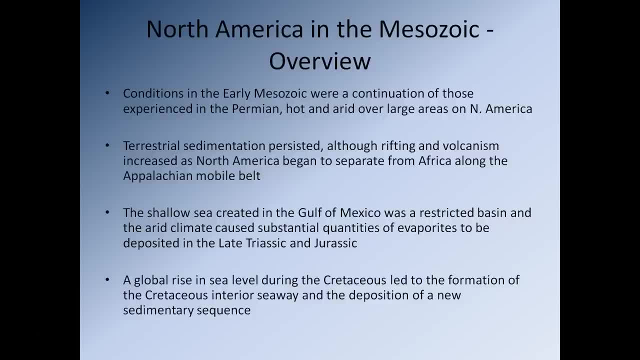 English story. uh, well, you know, you can guess I'm kind of running out of things to do code words about. I'm staying in my bookshelf right now and it was the first book that I saw. so that's Beowulf, that's b-e-o-w-u-l-f, so make sure you write that down for the code word quiz, okay. so, uh, pause the. 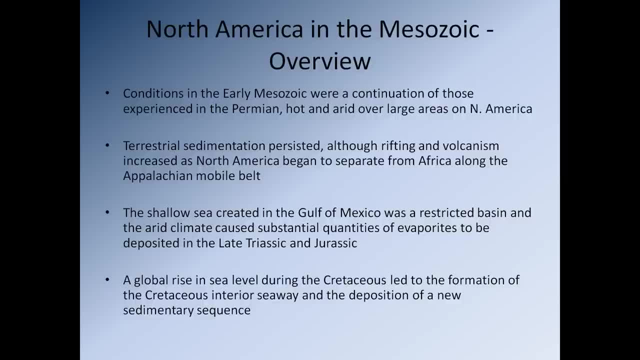 presentation. get up, have a walk around, get in a glass of water and please come back in a few minutes. okay, so what's happening in the Mesozoic for North America? well, conditions in the early Mesozoic were continuation of those experienced in the Permian. it was very hot, it was very arid. 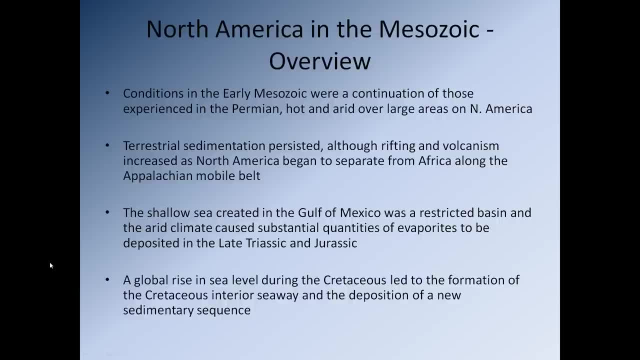 over a large quantity of North America. so essentially conditions in the Triassic were very similar to those of the Permian. so terrestrial sedimentation persist persisted, although we had rifting and volcanism increasing as North America began to sedimentate and the Mesozoic started to separate from Africa along what is now the modern Appalachian mobile belt. so we had a 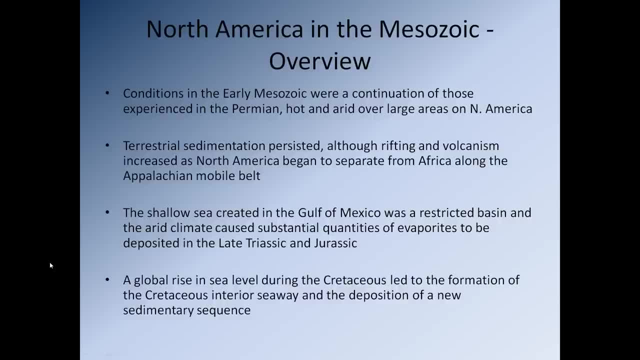 shallow sea created in the Gulf of Mexico and that, for a period of time, became a restricted basin and, due to the fact it was in an arid climate, you had substantial quantities of evaporation leading to uh sequences, sequences of very thick evaporites being deposited in the late Triassic and very 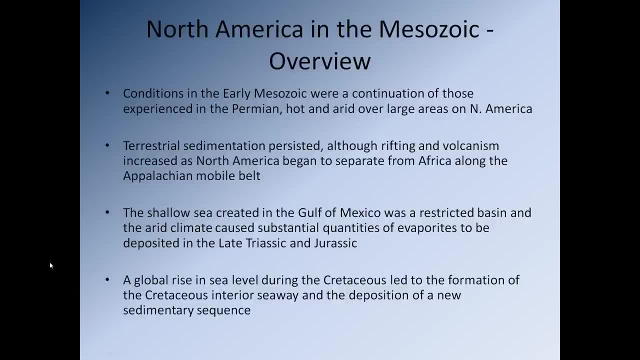 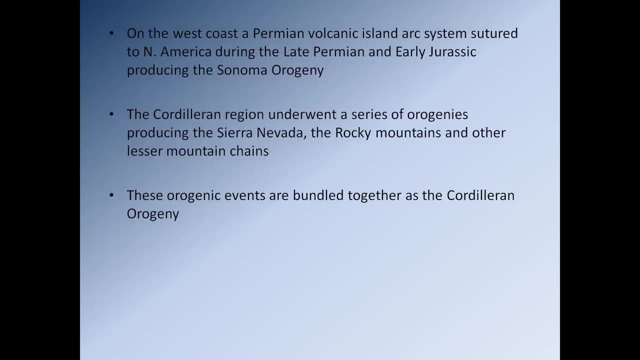 early Jurassic. and then we get the global sea level change of the Cretaceous, leading to the formation of the Cretaceous interior seaway and the deposition of a new sedimentary sequence. so, if you remember, that's the Zuni sequence. so on the west coast we have a 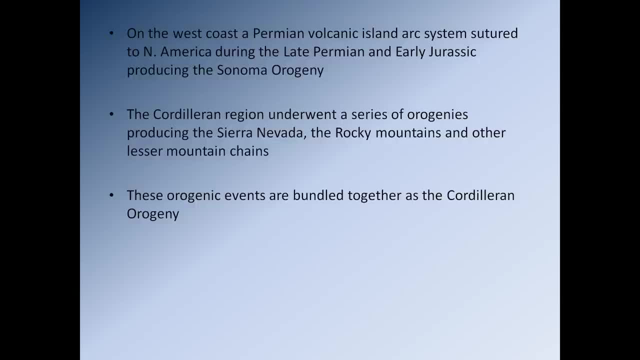 Permian volcanic island Arc system suturing itself to North America during the late Permian and early Jurassic and that leads to the Sonoma orogeny. we also have the uh cordial region undergoing a series producing the Sierra Nevada, the Rocky Mountains and a few other lesser mountain chains. these are 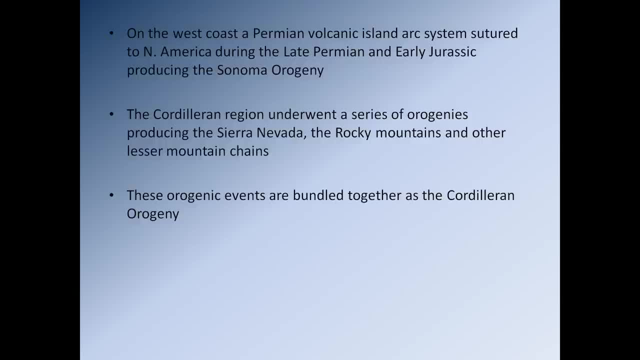 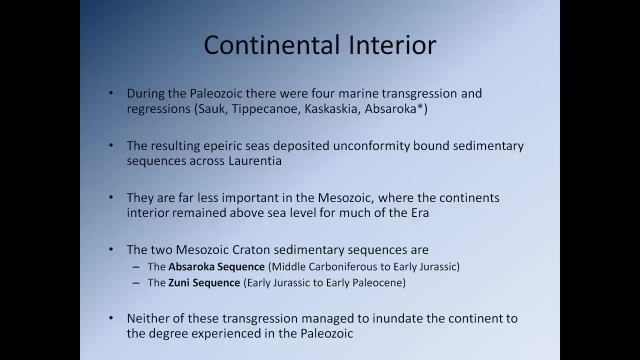 all lumped together generally and referred to as the Rockies. so these orogenic vents are bundled together as the cordial orogeny. okay, so what's happening in the center of North America during this period? so during the Paleozoic, there were four marine transgressions and regressions: the 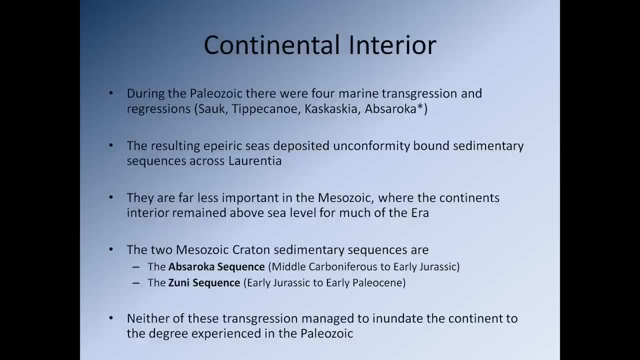 soak, the tip of canoe, the cascassia and the absaroka. if you remember, the absaroka straddles the boundary between the Permian and the Triassic, so the resulting Epiric seas were the focus of the deposition of lots of sediment and we have 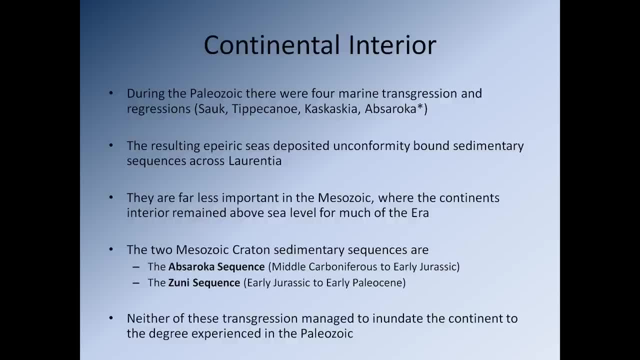 unconformities at the top, of, the top and bottom of these sedimentary sequences. so these sedimentary sequences are far less important in the Mesozoic, where the continent's interior remained above sea level for the vast majority of the Mesozoic. so the two Mesozoic cratonic sedimentary sequences are of course the absaroka, which is middle. 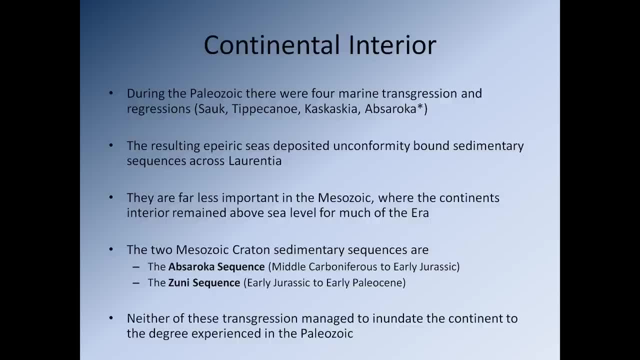 Carboniferous to early Jurassic, and the Zuni, which is early Jurassic, to very, very early Paleocene, so just into the Cenozoic. so neither of these transgressions produced managed to inundate the continent to the same degree experienced during the Paleozoic. so, on the whole, these 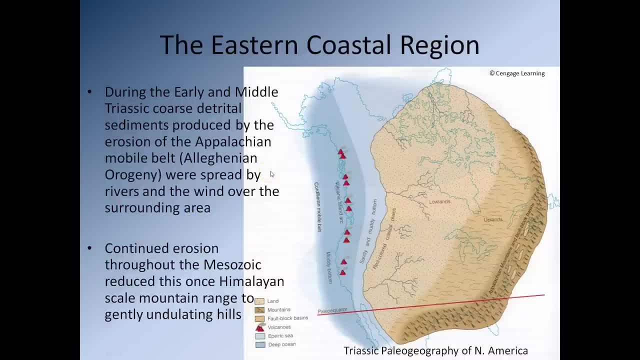 sequences were nowhere near as expansive. all right, so what's going on the East Coast during the Mesozoic, so during the earlier Middle Triassic, we have coarse detrital sediments produced by the erosion of the Appalachian mobile belt, and they were spread by rivers and wind over the surrounding. 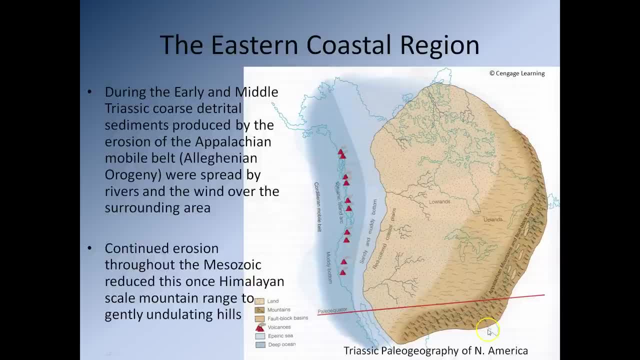 area. so we have the. you have the erosion of the Appalachian mobile belt here and we have rivers depositing those sediments to the northwest and to the southeast. we have the continued erosion of the Appalachian mobile belt throughout the Mesozoic and that's going to reduce this one's. 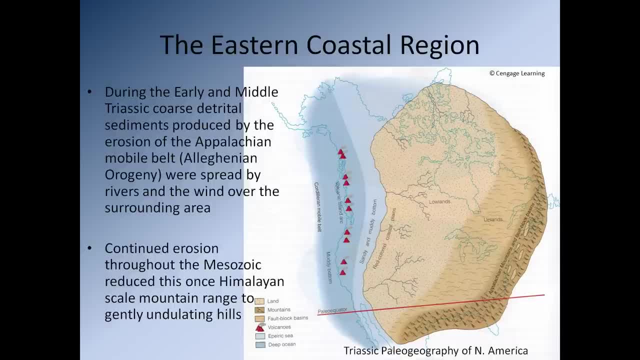 Malayan-sized mountain range to essentially a set of gently undulating hills, and there is some argument to suggest that by the end of the Cretaceous the Appalachian mobile belt was completely flat and was in fact a river plane. so you know, topography wise it would have looked. 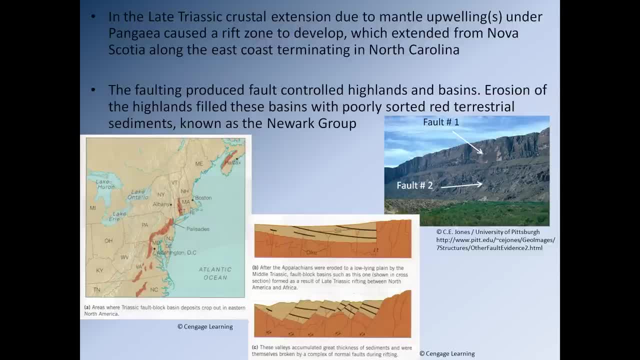 quite a lot like the area around Houston. so in the late Triassic there was crustal extension due to upwelling, just so, due to mantle upwelling under Pangaea, and that caused a rift to develop that extended from Nova Scotia down the east coast of the United States, terminating somewhere. 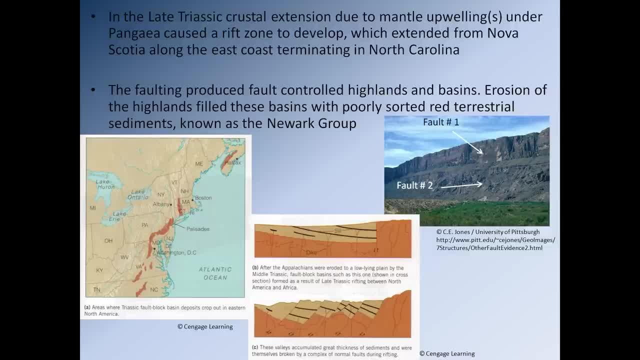 around North North Carolina. that's essentially where it started, and so we can see here on this map here, these areas marked out in this kind of brown color. these represent areas of rift related volcanics and sediments. so this entire area was undergoing extension, it was being stretched and 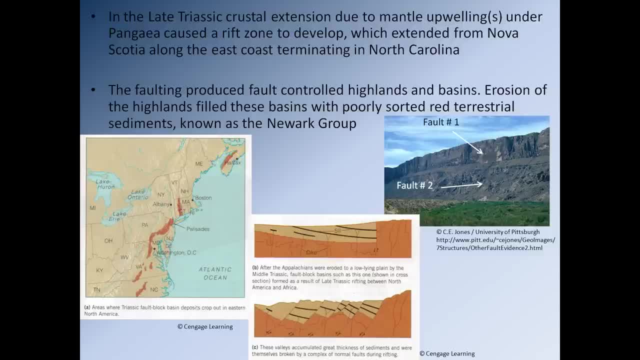 as I already touched on, when you start stretching a rock, initially for a short period of time, it will behave like a liquid. it will behave like a piece of silly putty. as you stretch it it will begin to become thinner. now we'll only do that for a little while. eventually you get to the point: 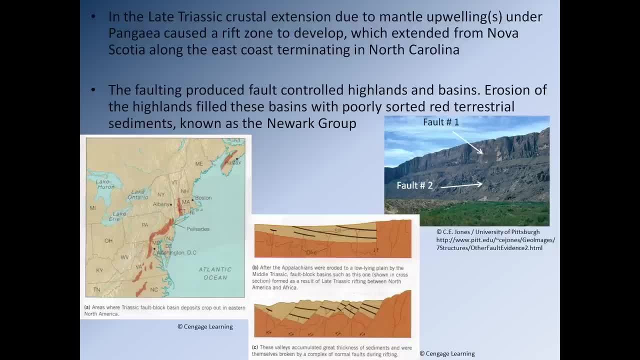 where the rock won't stretch anymore, at which point it will just simply break like a solid. so if we look at this diagram here, we can see this is the kind of situation we have in these regions. here these rocks have undergone extension and as they've been extended they've broken into. 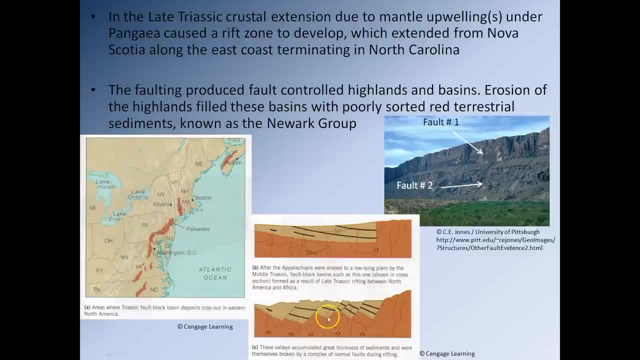 these big fault bound blocks. they've got a fault on one side and a fault on the other, and so, as the crust was stretched further and further and further, one block would drop down, another block would drop down, drop down, drop down. so the blocks would drop down relative to each. 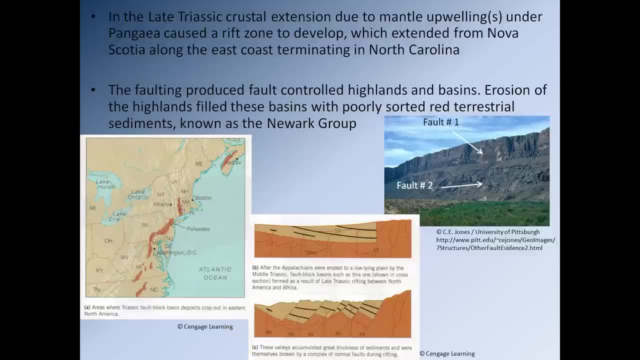 other and this produces a depression, otherwise known as a rift Valley. so these are big, normal faults. okay, and we can see so if we look at this picture here. this is actually a rift Valley here, so we can see this is one fault block up here. so this flat surface is flat cliff face here. 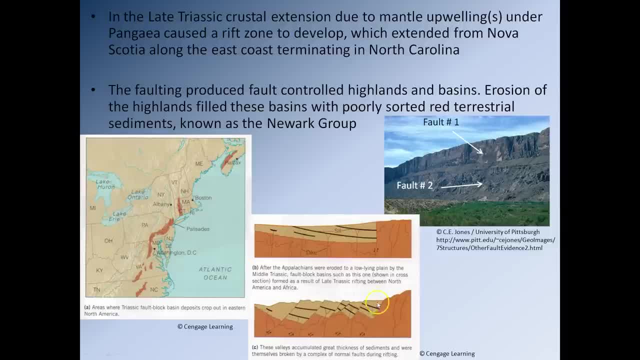 that's the fault, okay. so let's say this represents this fault block here. okay, so then we have this fault block here. okay, that's dropped down relative to this block up here, and so let's say that's this block here. then we actually have this fault block here, which is the one the photographer's standing. 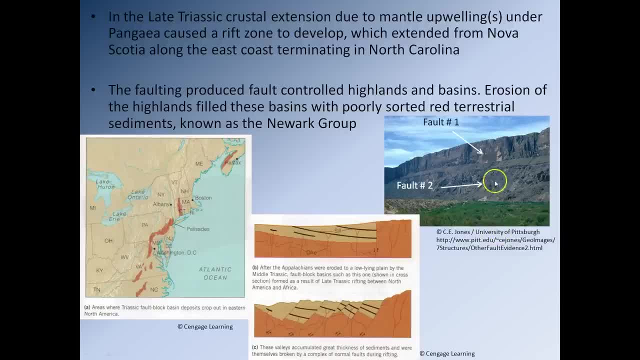 on. okay, this is dropped down relative to this fault block here, so let's say that is this fault block here. so what we have essentially is we have blocks of rock dropping down relative to each other as the crest crust gets stretched and you can see it's formed a topography. the person taking the 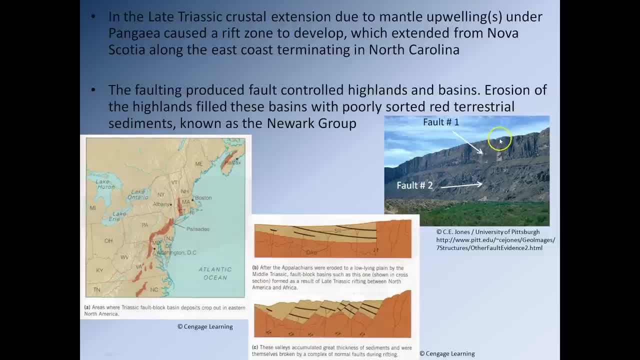 photograph is much, much lower than the initial land surface up here, and so, as this entire area undergoes extension, you end up forming a long, linear Rift Valley. now, obviously, what happens is is these faults here become a channel for magma, so as this crust gets thinned, the mantle underneath is under lower pressure and of. 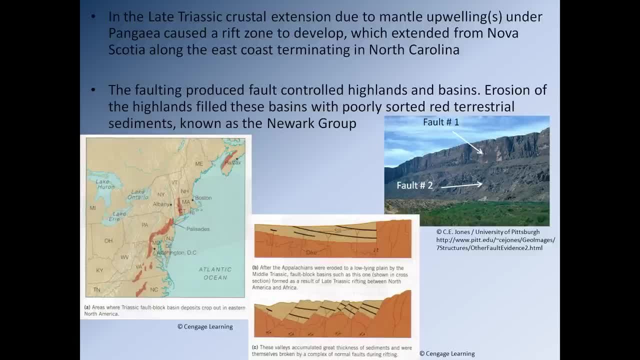 course it starts melting and, as we've already discussed, that melting magma is going to produce a mafic magma that's going to enter the crust and it's going to work its way through the crust and it's going to focus itself primarily along these faults. here they're going to be nice easy pathways. 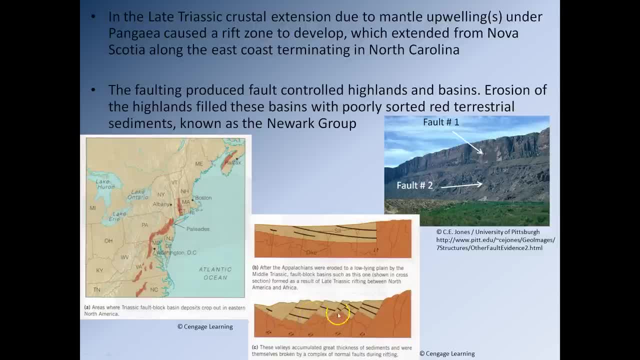 along which the magma can move. the other thing that's going to happen is these Highland areas that are produced by the faulting these, these areas up here. well, these are going to erode. so this area here is going to erode faster than this area down here, and so the 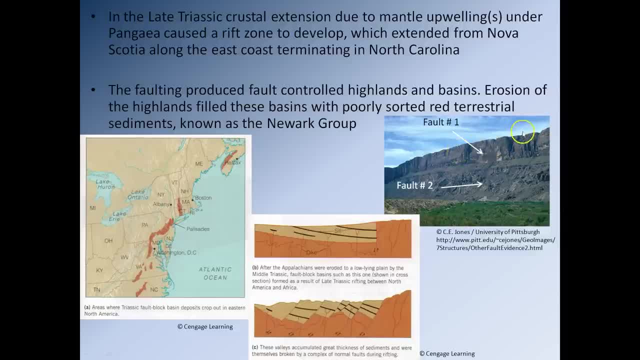 Highland areas produced by the, the, the rifting are going to be eroded. they're going to produce clastic sediments. they're going to be deposited into the Rift Valley. so the Rift Valley is going to be a mixture of clastic sediments produced by erosion and typically mafic volcanic rocks. 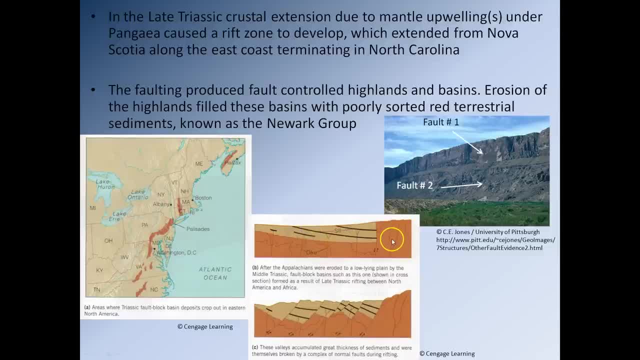 a lot of mafic dykes and a lot of mafic silts. so the erosion of these Highlands produced essentially a sequence of sediments, which is referred to as the Newark group, and it's dominated by red terrestrial sediments. that tells us the 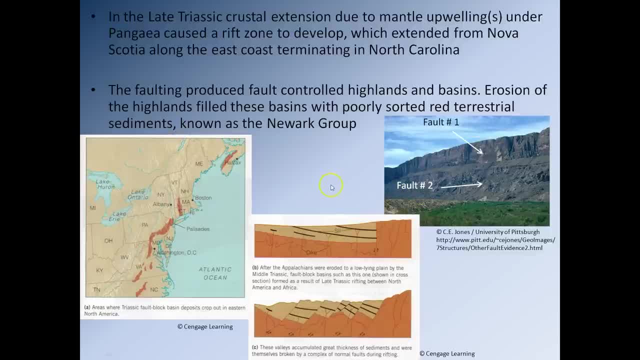 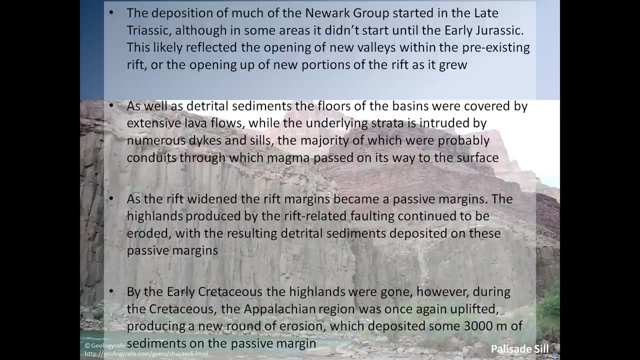 sediments are being eroded and deposited into a Rift Basin in a arid or semi-arid environment. so the deposition of much of the Newark group started in the late Triassic, and so that gives us an idea. and so that gives us an idea about 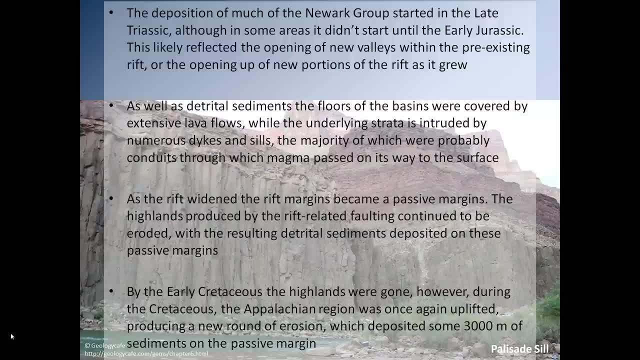 again. I do apologize for that. that was one of my children. so the deposition of the Newark group started in the late Triassic, although some areas didn't start until the early Jurassic. so if you remember the rift, the rifting started in the Northeast and worked its way down towards the 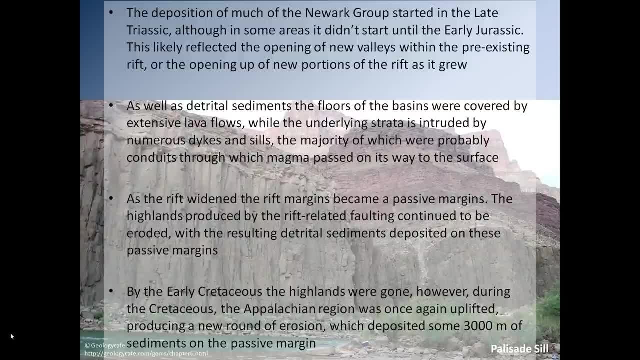 Southwest, so we. so we see the rifting started first in the Northeast. so we get the oldest uh parts of the Newark group in the Northeast and as the rifting progresses Southwest, we get steadily younger and younger sedimentary rocks being formed. so as well as the 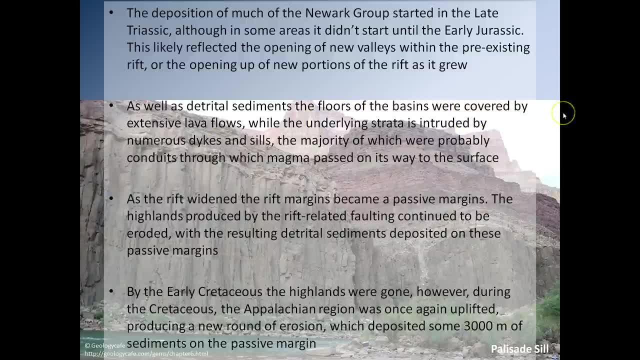 vital sediments. from the erosion, we obviously get the formation of extensive lava flows, and obviously these lava flows have to be fed by an underlying pipework, and so within the Newark group we have lots and lots of dykes and sills being intruded. all of its matrix mostly dominated. 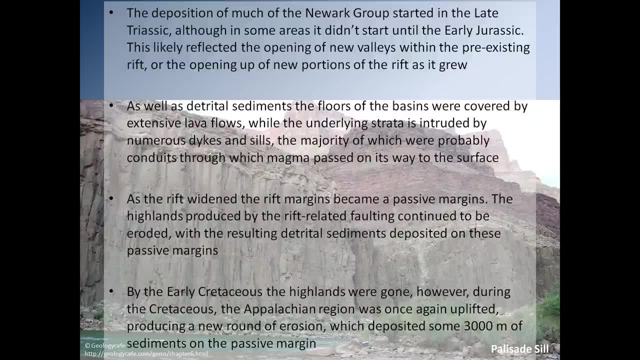 by basalt, so as the rift widened. eventually the margins became passive and we formed a proper ocean basin. so when we formed the North Atlantic proper and we start forming oceanic crust at a spreading Ridge, now at that point the East, the eastern seaboard becomes a boring passive margin, nothing much. 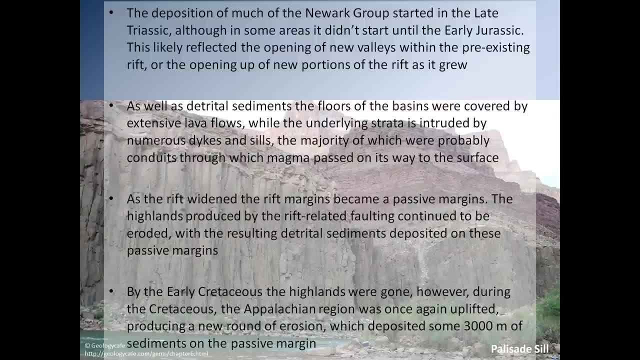 happens, it becomes nice and dull. so by the early Cretaceous any remain, you know, any remaining Appalachian highlands are gone. the area is almost flat, and so essentially you know nothing's going to happen until the Appalachian region is once again lifted up, and that's going to occur during. 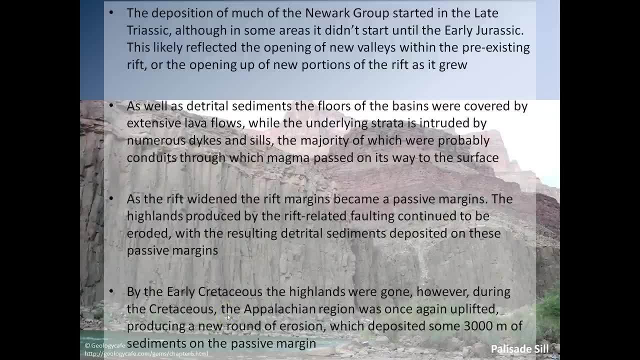 the Cretaceous. so during the early Cretaceous the entire thing's been plain flat. then there's a short area, a short period of uplift that pushes the area up for a little while. there's a round of deposition, there's a round of erosion- sorry, 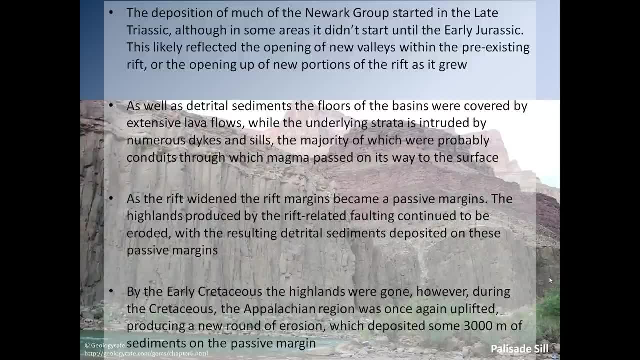 that's going to deposit around 3 000 meters of sediments onto the passive margin and then the uplift is going to stop again and the entire area is going to become a flat river plain once again. so just to give you some idea of the the newick uh group sediment. so here we go. you can actually 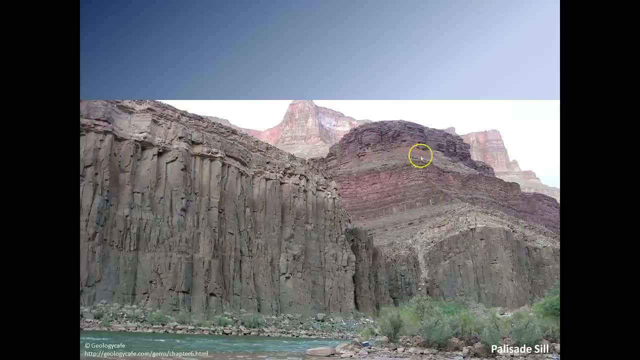 see the new group sediments, these nice red, mostly sandstones you can see in there. the red color obviously tells us they're being deposited into an arid to semi-arid environment and you can actually see we have this big layer of rock here. this is a sill. so this is a layer of mafic magma. 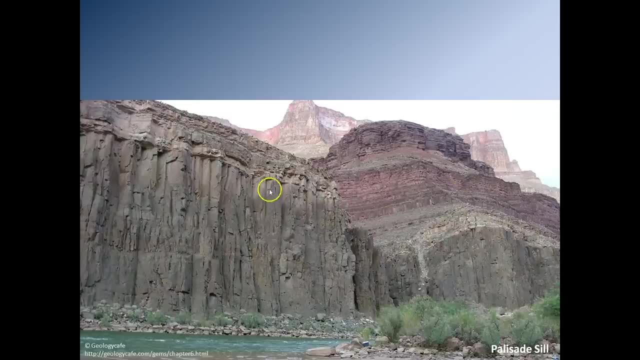 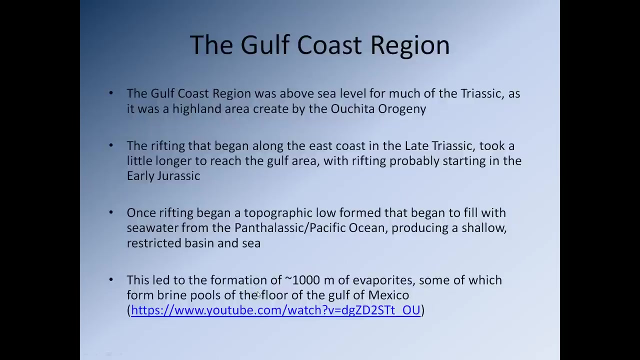 that's been injected parallel to the bedding and so that gives you some idea of the quantity of magma that was moving underground, so large quantities of magma, you know, being intruded into the crust during this period of extension. okay, so what's happening in the gulf region? so in the gulf region, the area was once again above. 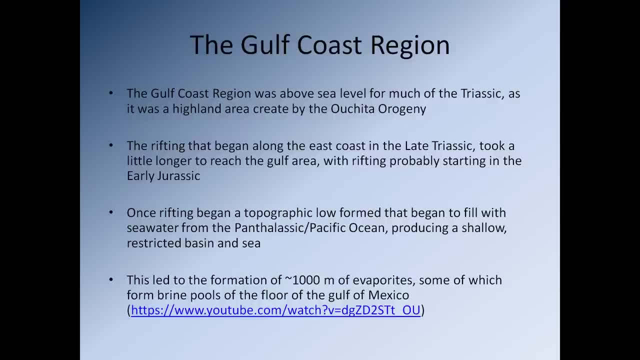 sea level for much of the trassic, as it was a highland area created by the achida neurogeny. so the rifting that began along the east coast during the trassic took a little longer to reach the gulf area and rifting probably started somewhere around the early jurassic. so once 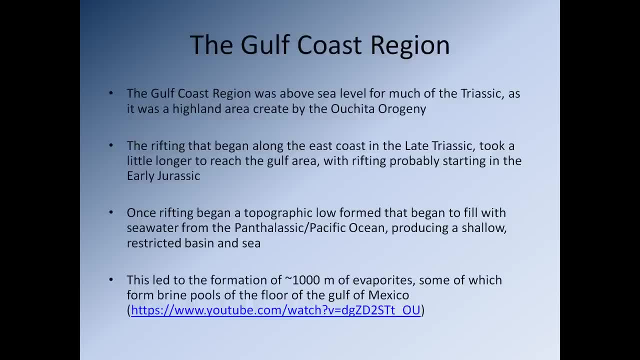 rifting began. we form a rift valley, so we form a topographic low and that topographic low eventually becomes deep enough to fill with water from the pacific ocean and that produces a shot that produced a shallow, restricted basin and that restricted basin obviously underwent evaporation and that led to 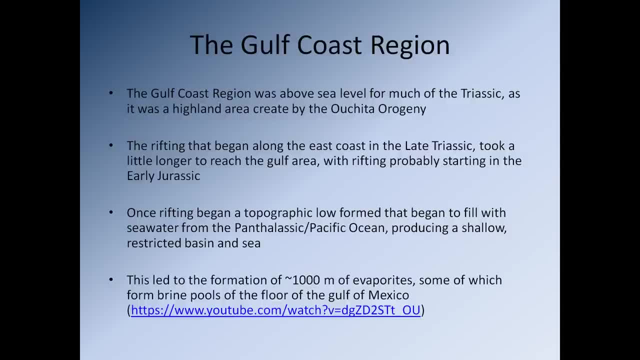 the deposition of quite a thick sequence of evaporites, approximately one kilometers worth of them, and that occurred, as i say. that occurred typically during the middle jurassic. during the early to middle jurassic, now by the late jurassic, the rifting was not so strong, and so the rifting was not so strong. 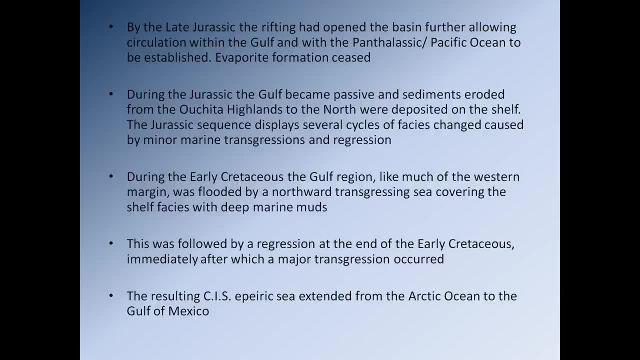 the rift had opened up even further. this meant even more water could flood in from the pacific, and so that stopped the evaporation. so essentially, that's the point where the evaporite deposition stops. so during the jurassic the gulf became a passive margin and sediments were eroded from. 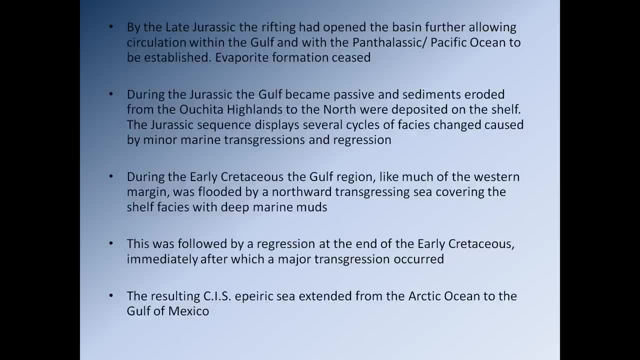 what was left of the achiton highlands to the north and they were deposited onto the newly formed continental shelf. so the jurassic sequence displays several cycles of fascius changes caused by minor marine transgressions and regressions. so the essentially the south coast of 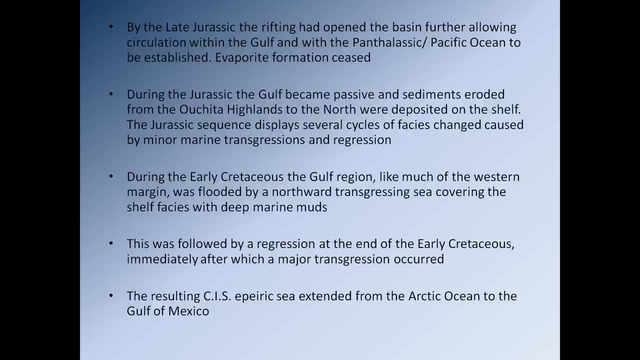 north america is exposed to lots and lots of sea level changes, going up and down quite a bit. so by the early cretaceous the gulf region, like much of the western margin, was flooded by. the northward transgrid was flooded as part of the zuni sequence and, as you know, eventually the body 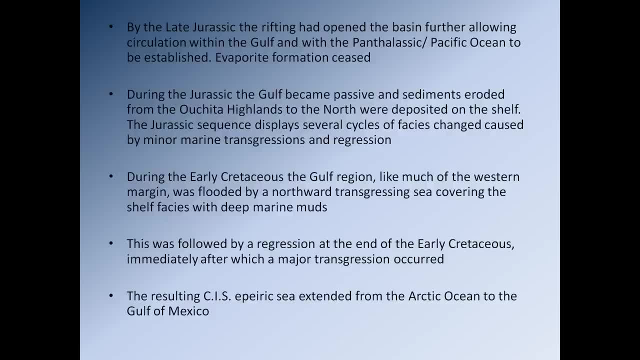 of water linked up with the body of water coming from the arctic sea and that created essentially the cretaceous interior seaway that stretched from the arctic all the way down to the gulf of mexico. so that pretty much covers what's going on for the 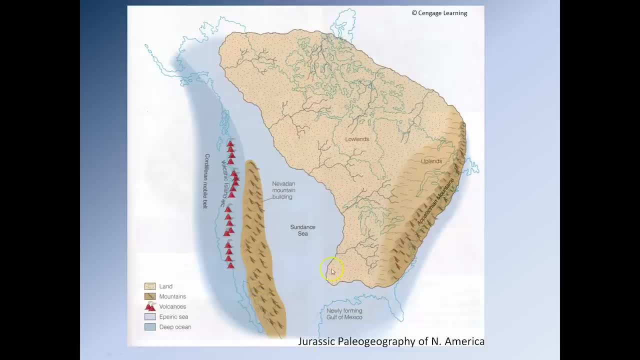 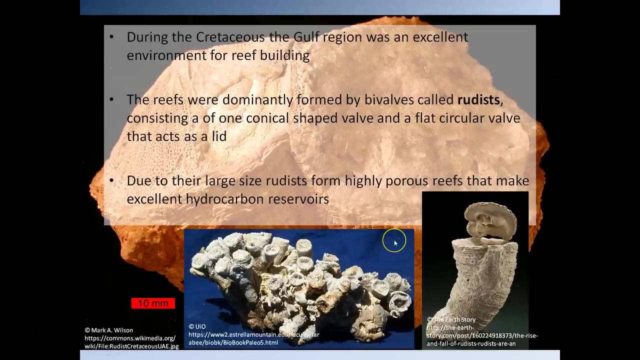 gulf region. so in by by the time we make it into the very late jurassic, into the cretaceous, you can see we have this body of water that extends from the newly forming gulf of mexico all the way up to the arctic ocean up here. so during the cretaceous, the gulf region. 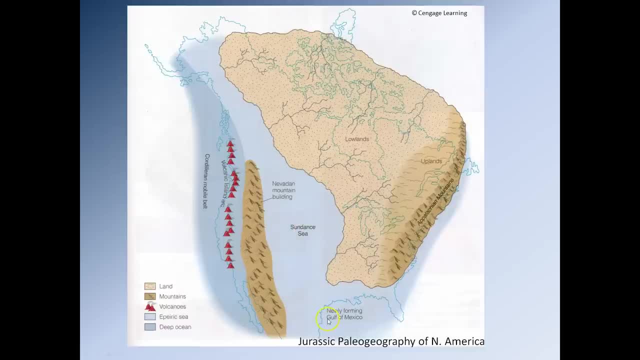 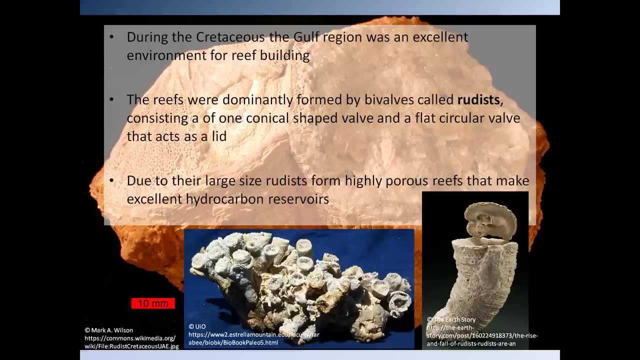 was an excellent environment for reef building, so this area down here was a prime location for large scale carbonate formation. and that's exactly what happened, and so the area became covered in reefs, and so the cretaceous reefs were dominated by an organism which is referred to as a rudist. 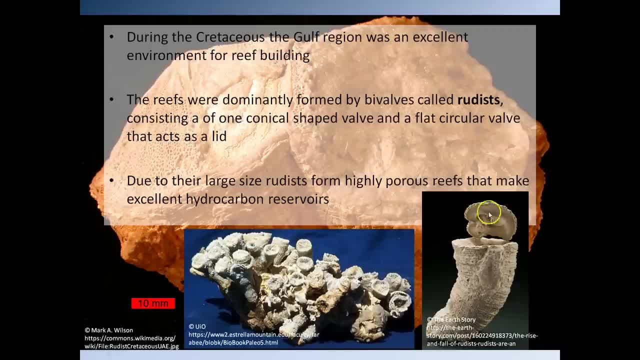 it's a type of bivalve and it has this distinct horn shape to it. so the lower valve has this kind of- you know, cone shape and the upper valve forms a lid. so due to their large size these rudists essentially would form huge reefs and obviously when one rudist fell over, 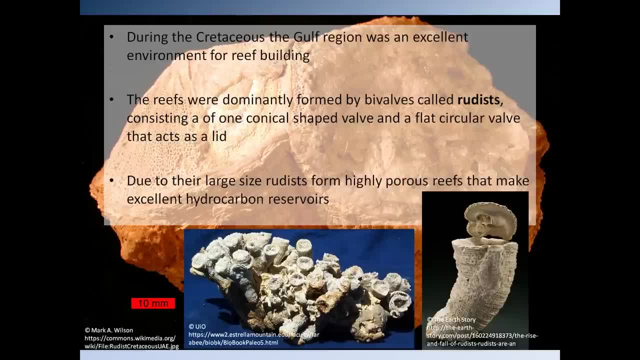 a new rudist would just grow on the shell of the old, old rudist, and so eventually, the limestone that's formed by these rudists is essentially just a pile of, you know, rudis. it's very, very porous. there's lots of gaps in between them, and so that makes this particular limestone that was forming 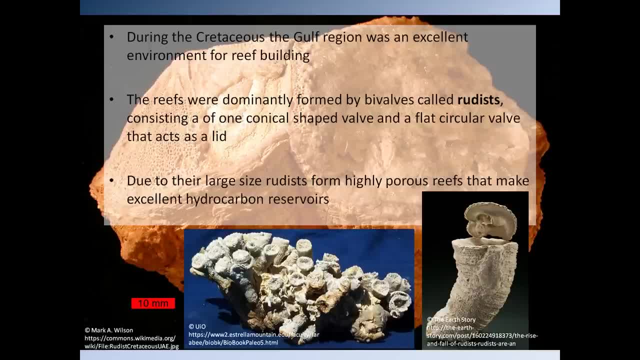 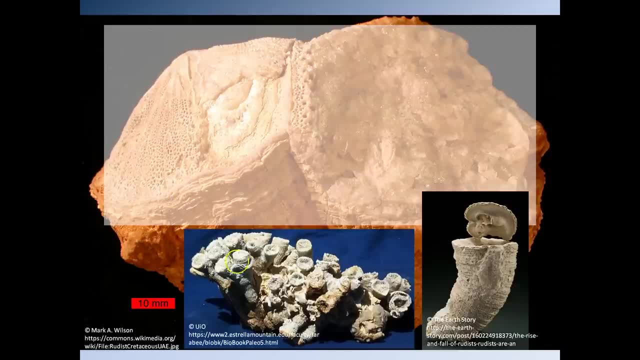 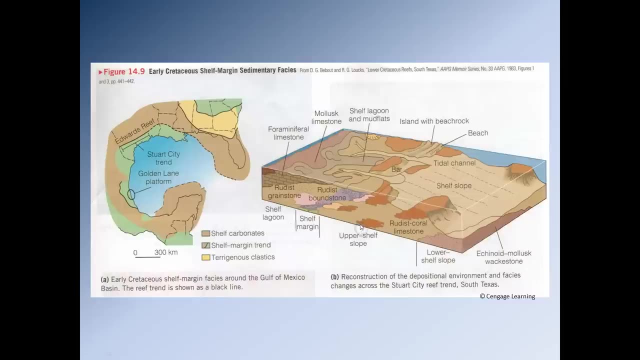 during the cretaceous, an absolutely excellent reservoir rock for oil because there's lots of porosity for the oil to move into. so you can kind of see. so here's a nicely preserved rudist here. here's a hand specimen that shows you a number of rudists all together and this picture behind. oh sorry, you're going to go back there and 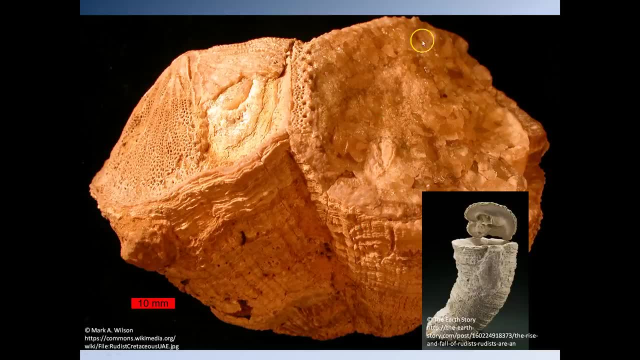 this picture behind shows you two rudists. so this rudist here you can see, you can kind of make out the core of it there, and you can see the shell coming around here like this: it's missing its lid now. this rudist over here is the same, is the same thing. so here's the cone. that's one half of the. 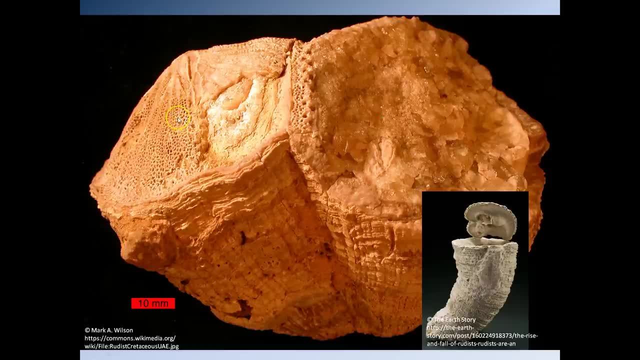 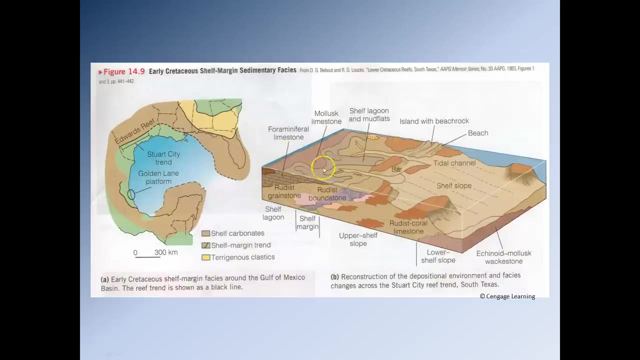 valve. here's the edge of the cone coming around here and you can see this kind of honeycomb looking material. that's the lid. okay, so you can see this valve. is this particular rudist is actually, you know, more or less complete. so the position, uh, the situation in the uh, 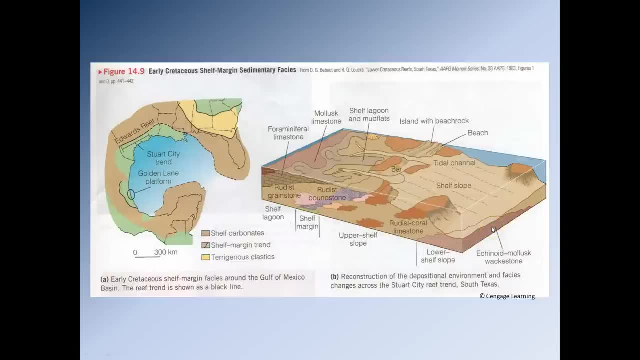 cretaceous will look something like this for the um, for the gulf coast region. so you know, we would have had closest, so we've had north america up here, deeper water down here and obviously we would have had several- uh, rudis dominated reefs forming that would have protected a carbonate lagoon behind, and so within that, 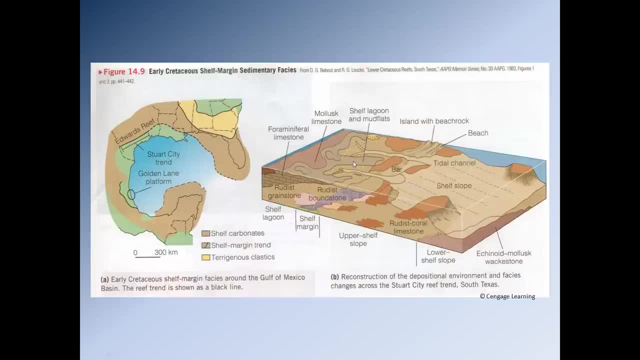 lagoon. obviously we would have had a build-up of essentially- uh- carbonate muds and obviously we would have had lots and lots of life in this area as well. so this carbonate lagoons would essentially be dominated by, you know, macritic carbonates, lots and lots of shells, lots and lots. 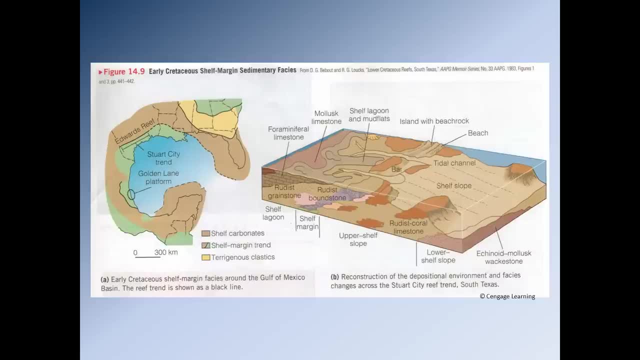 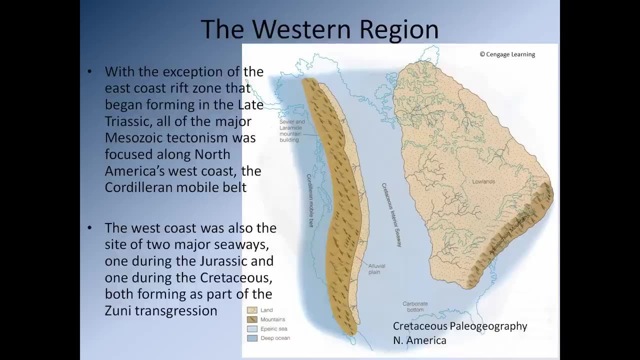 of fossils, you know, ooids and other, you know carbonate particles would also have been present, and so you can essentially see it's the classic carbonate platform, really, in terms of the western region, what's going on there? so, with the exception of the east coast rift zone that began in the late triassic, everything that's, you know, everything that's. 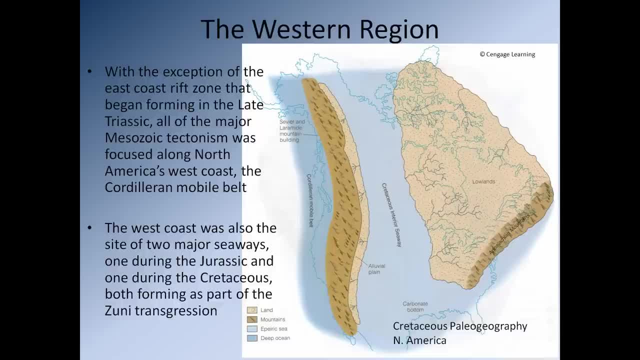 going to happen in terms of tectonism during the mesurk is focused on the west coast. it's the west coast where it's all happening. so the west coast was also the side, the site of two major seaways of course we have during the 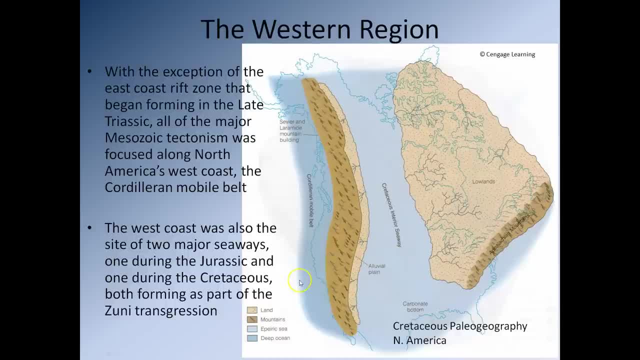 jurassic, we have the uh, the sundan sea, and during the cretaceous, of course, we have the cretaceous interior seaway. both of those bodies of water are, of course, part of the larger zuni transgression. now, in terms of the western region, as you can see, because it's a, you know, an area that's undergoing,